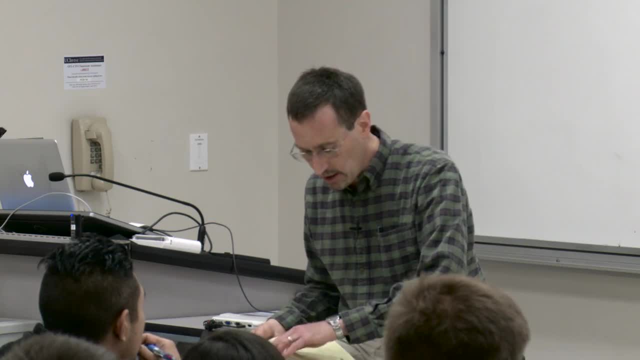 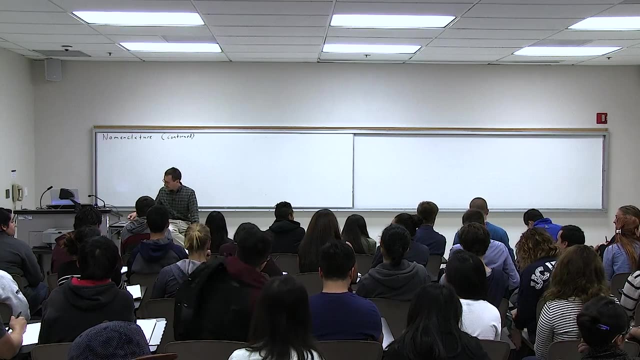 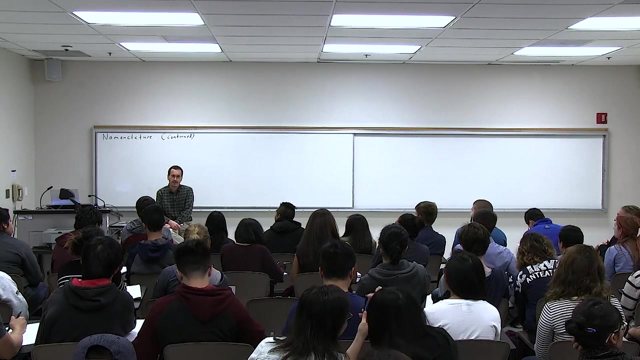 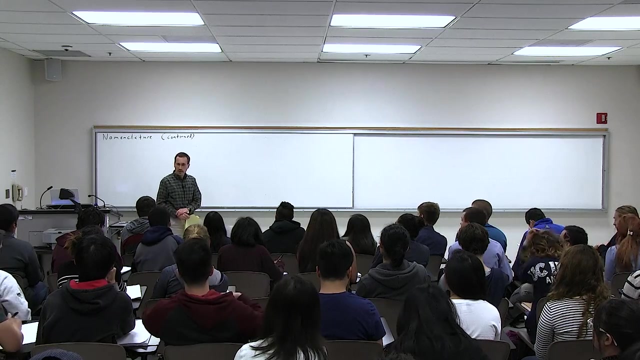 and we'll share a lot of answers and so forth. All right, we'll give it just one more moment here. Any questions to begin? All right? well, in that case, let's pick up with our discussion of nomenclature. 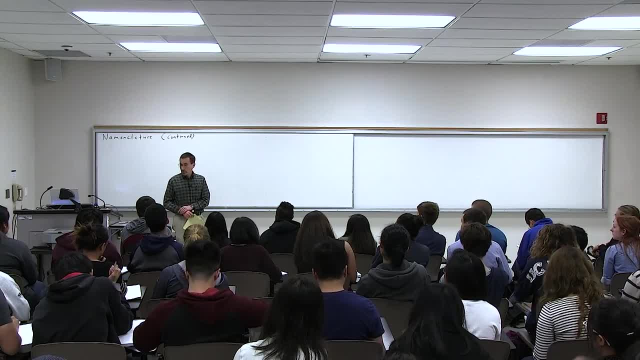 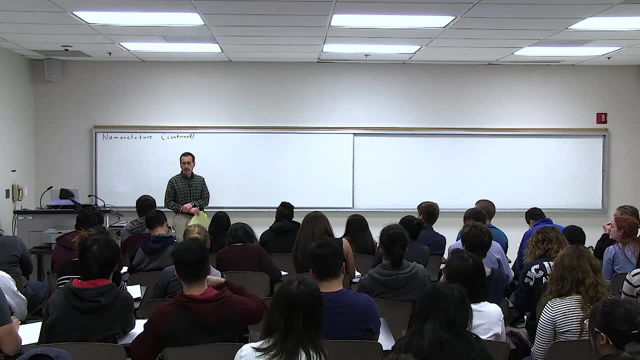 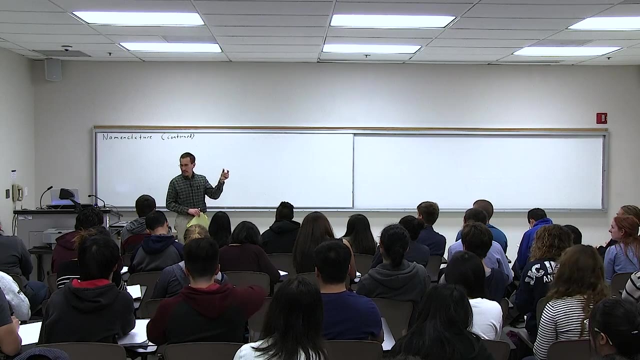 and this is going to finish it off, and as I for chapter one, and as I said last time, what I want us to be doing is not to be 100% masters of organic chemical nomenclature. I've got a book this thick- 300 and some pages- called the IUPAC Blue Book. that goes ad nauseam. 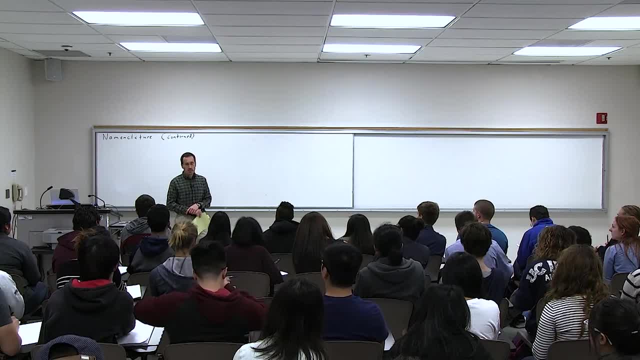 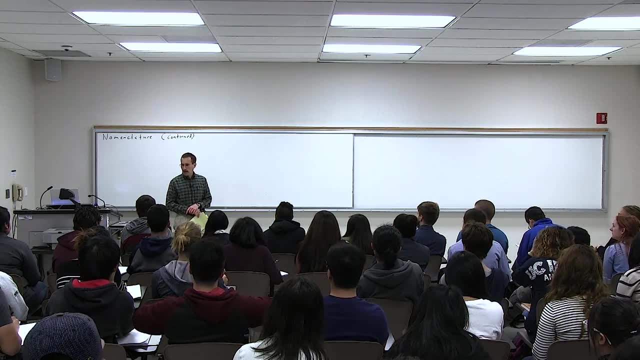 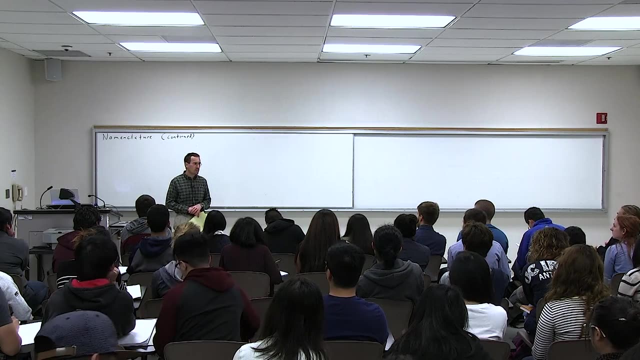 through nomenclature, and the great thing on a lot of that is you can look it up. What I want us to do is to start to see molecules and see molecules beyond the functional groups. with a little bit of alkyl groups spinach thrown on that, you got in sophomore organic chemistry. 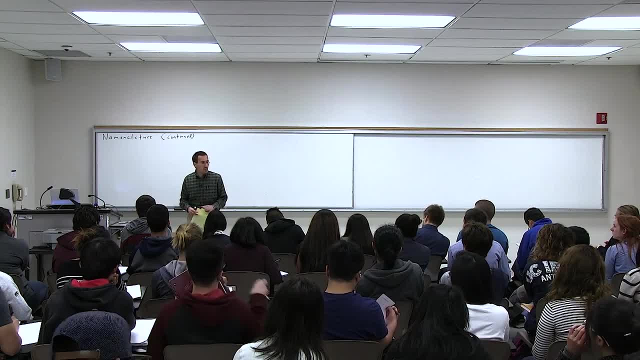 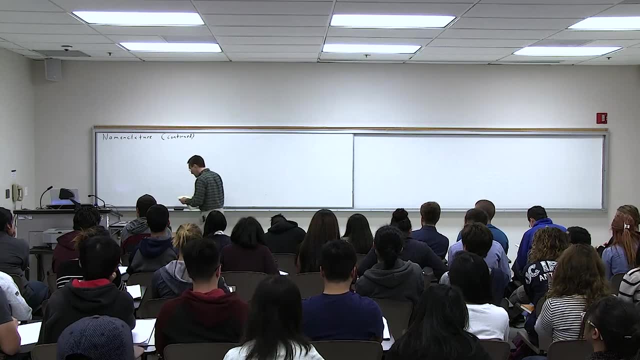 and see some of the beauty of them and some of the complexity, and we're going to try to do that today. And of course, we will see a lot of different classes of molecules as well. I know A lot of different classes of nomenclature. 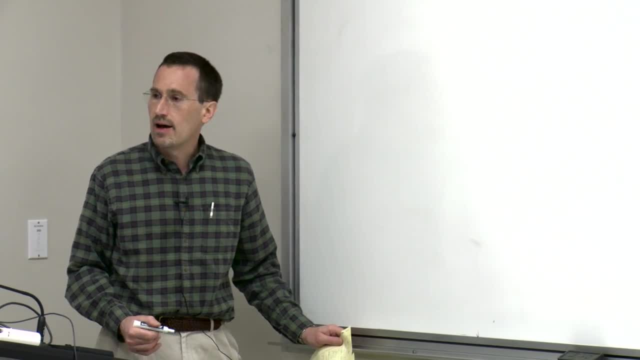 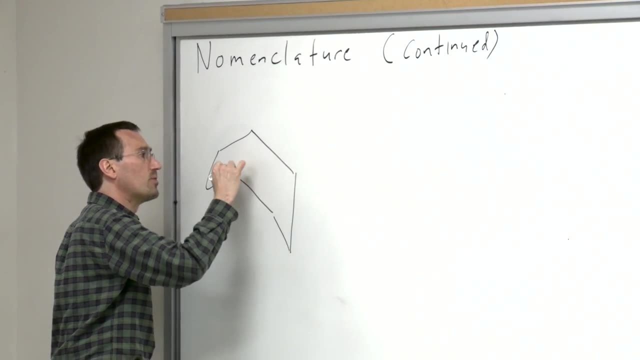 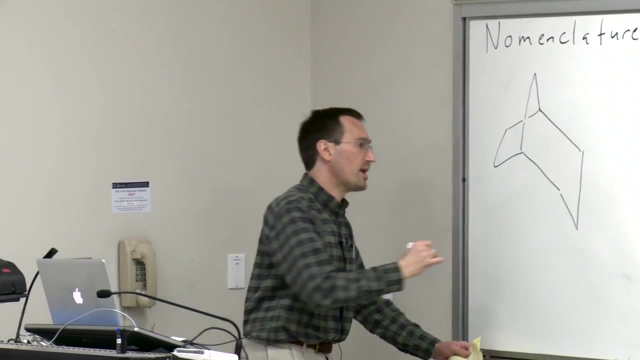 So last time we were talking about bicyclic compounds and bridge bicyclic compounds, and so I think sort of as an archetype, I started with this molecule and we talked a little bit about it: bicyclo-3-2-1 octane. 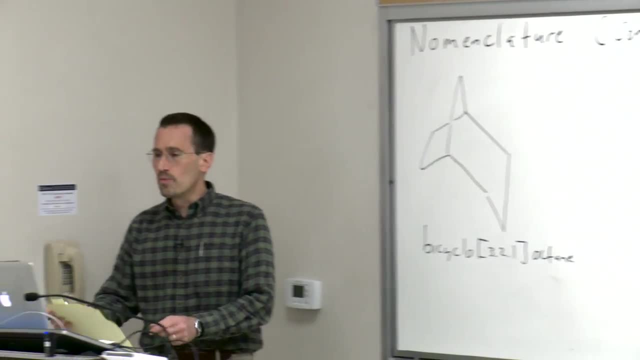 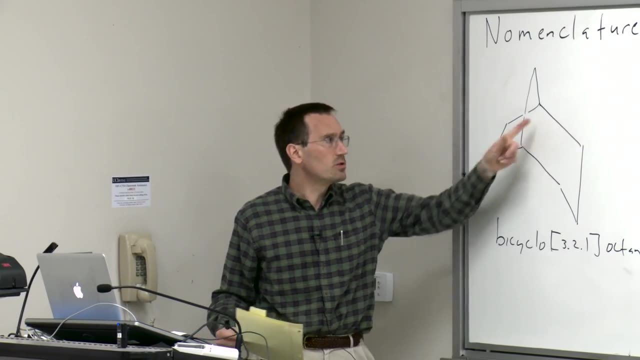 And we talked about the nomenclature a little bit and remember, I said, the basic ideas. we've got bridge heads in the molecule, the two junction points, and you number around the biggest bridge and then the next bridge and then the next bridge. 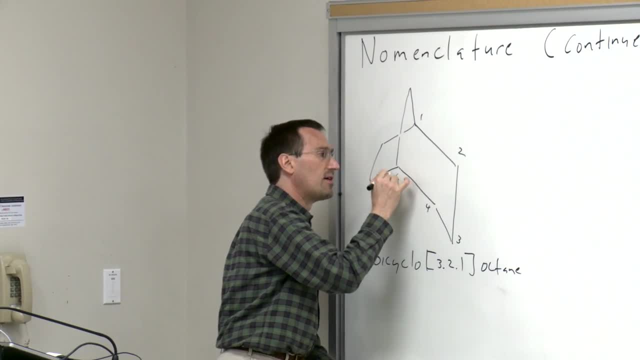 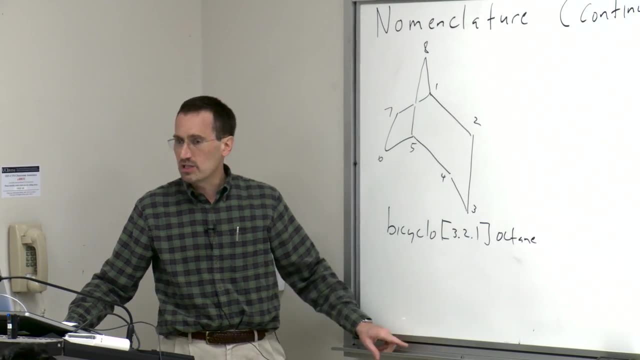 1,, 2,, 3,, 4,, 5,, 6,, 7,, 8,, and these numbers, here ordered from biggest to smallest, represent the 3-atom bridge, The 2-atom bridge and the 1-atom bridge. 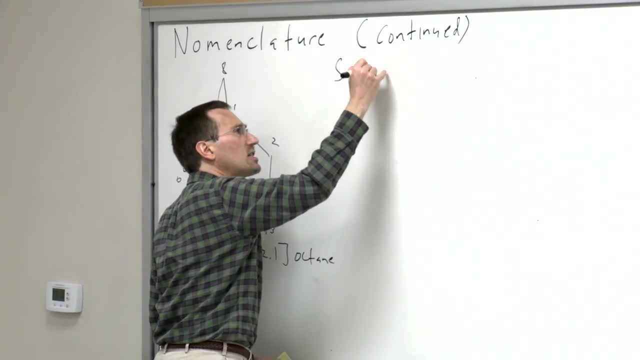 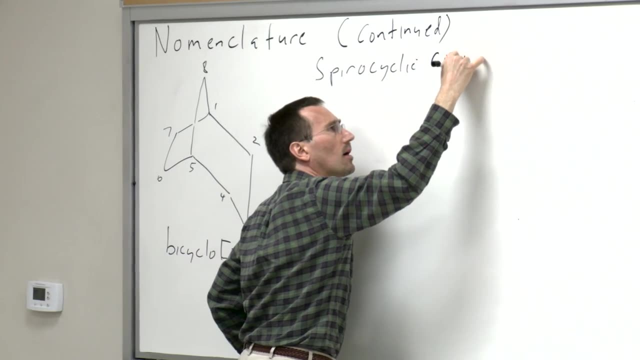 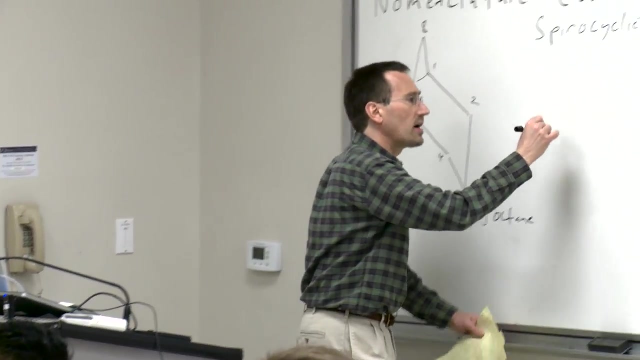 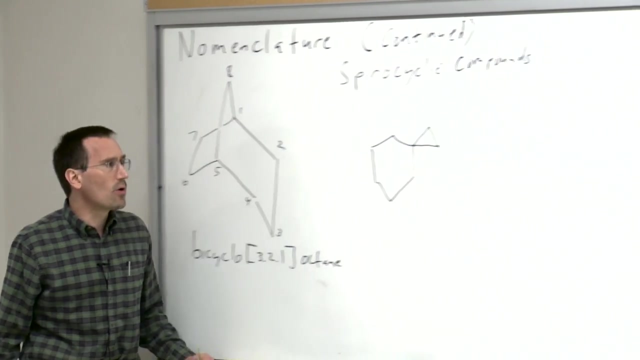 So what I want to do at this point is to juxtapose that nomenclature with that of spirocyclic compounds and also throw in a few other, or at least one other, prefix. So I'm going to give us an isomer of this molecule, molecule that also has two atoms. 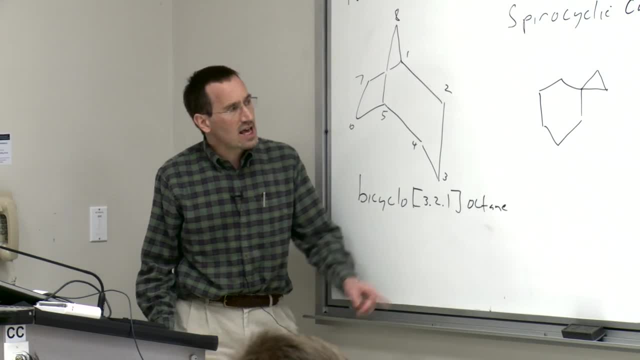 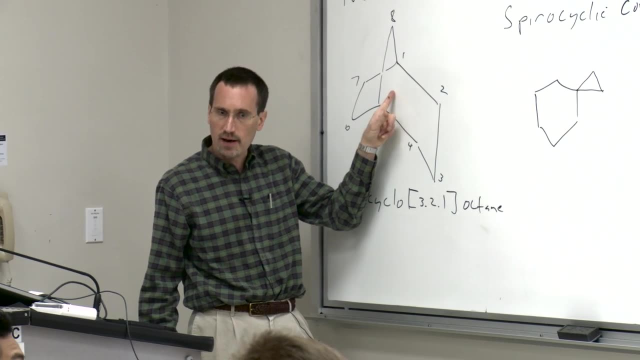 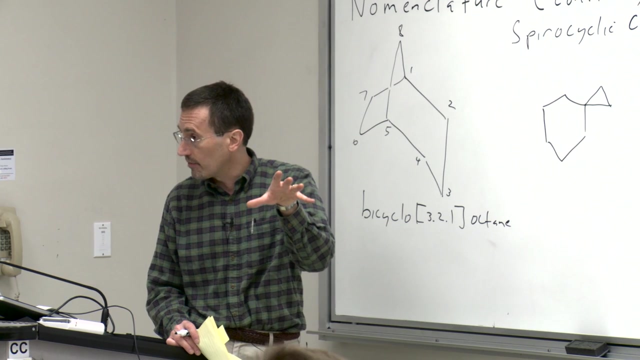 two rings to it, but now, instead of having the rings bridged or fused, so we call this a bridged bicyclic compound. When I showed diaza-undecene diaza-undecene at the very end of last class, we called that a fused bicyclic compound. 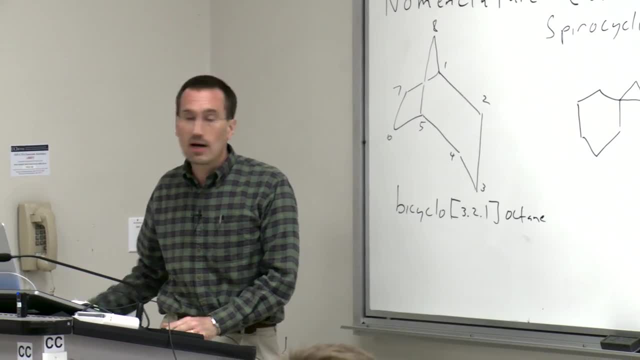 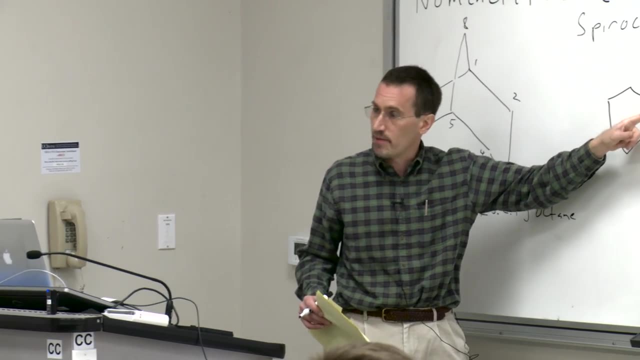 This we call a spirocyclic compound, because you've got sort of a, you've got a quaternary, You've got one ring, one carbon, one quaternary carbon with four substituents on it that joins the two rings. 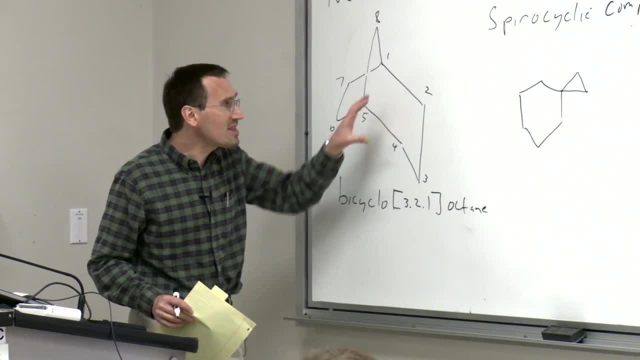 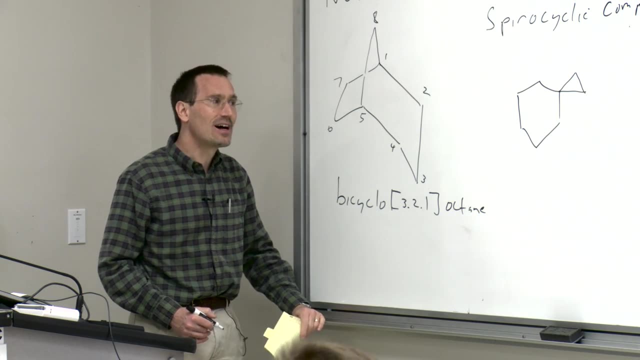 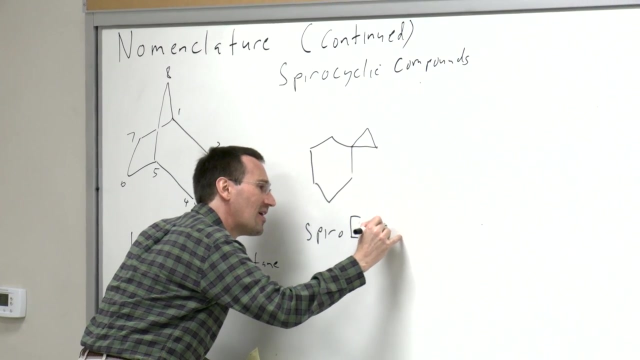 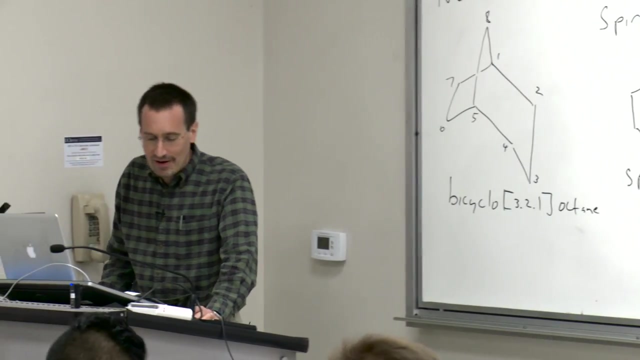 And it's sort of funny, in spirocyclic compounds, Everything that you do in bicyclic compounds you do opposite in spirocyclic compounds. So this compound here is called spiro-2,5-octane, And so we go from small number to big number, small and then big. 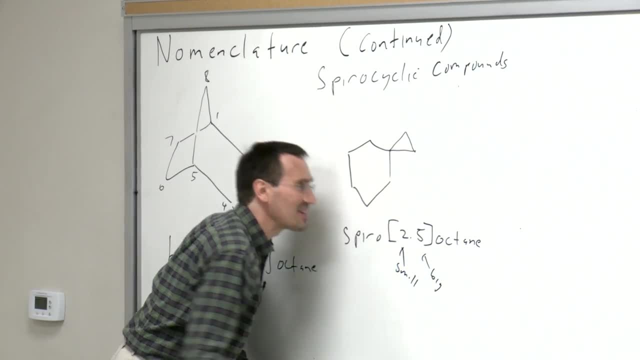 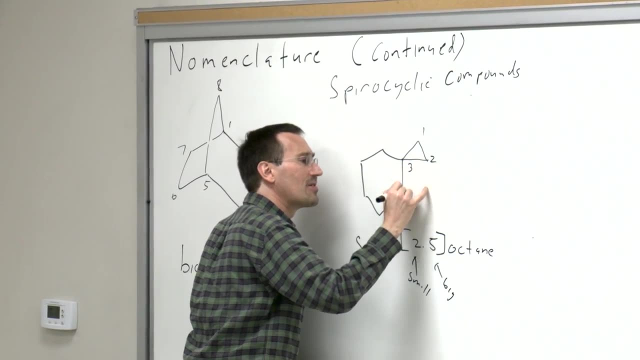 And sometimes you've got to laugh at nomenclature. Some of this is arcane, some of this is funny, but you see it once and you start to say, okay, there's at least a system to it, And then we do everything backwards. 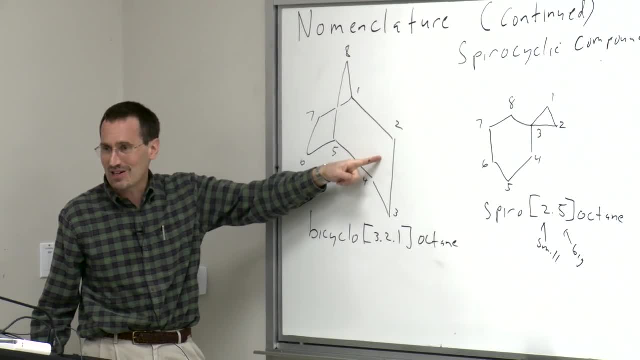 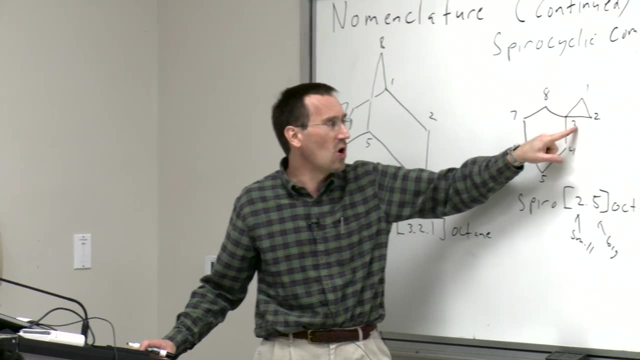 You don't start here. we started at the bridge head and did the big chain. Here we start on the small ring and we number around 1,, 2 for the small, then to the spirocarbon, 3,, 4,, 5,, 6,, 7,, 8.. 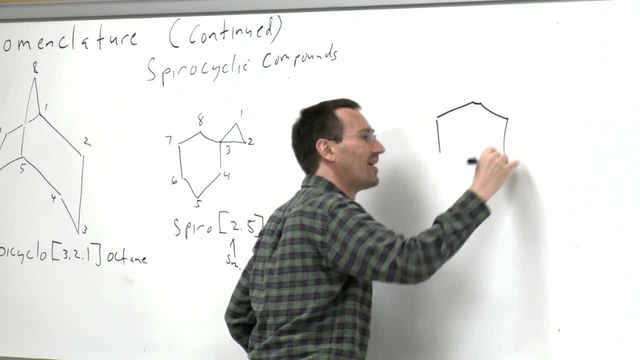 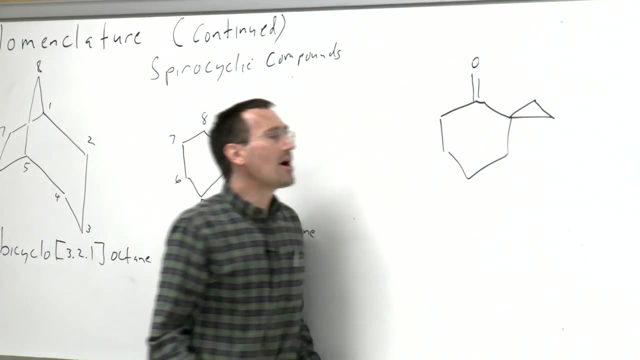 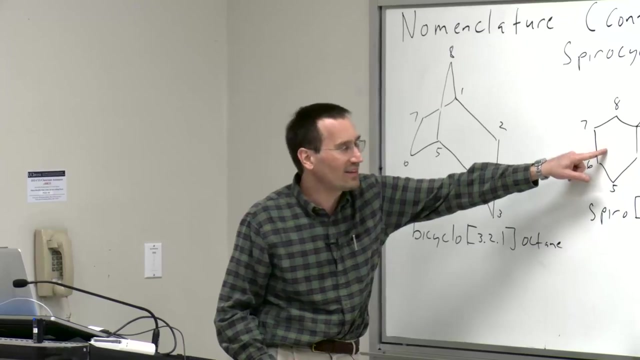 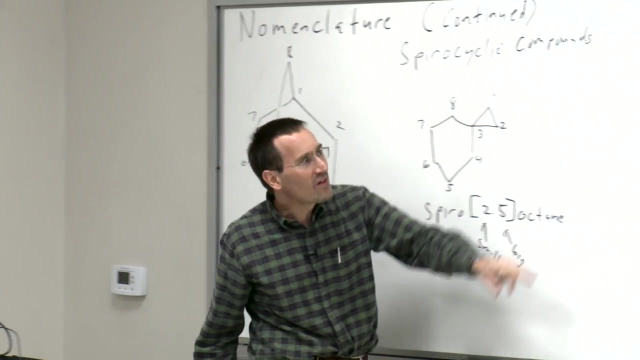 And so if you make a derivative like so, now we're going to name this compound as a derivative of spiro-octane and, more specifically, as a derivative of spiro-2,5-octane. We've got a ketone group, so remember you call like propanone is the ketone. 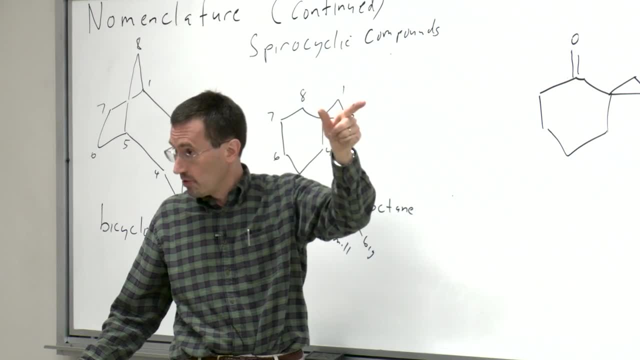 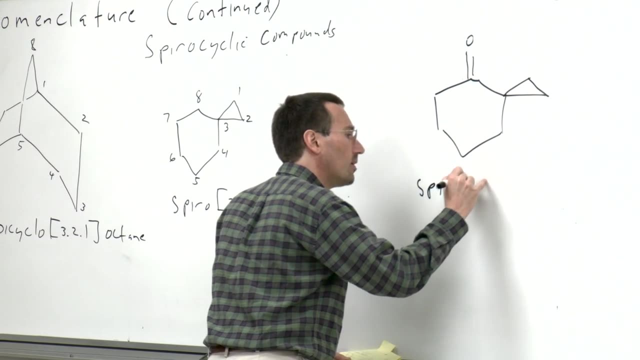 the 3-carbon ketone with the carbonyl at the 2 position of it. So we call this own and it's going to be spiro-2,5-octane-4-octane. Okay, Okay, Okay. 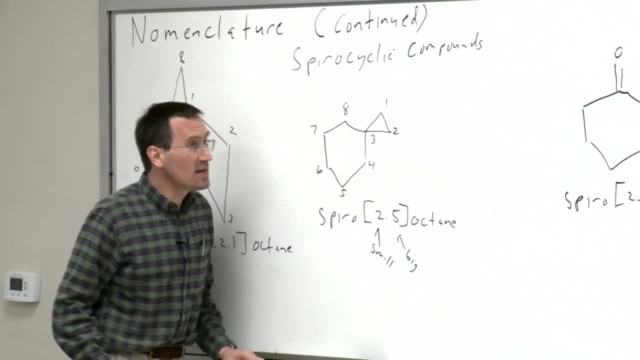 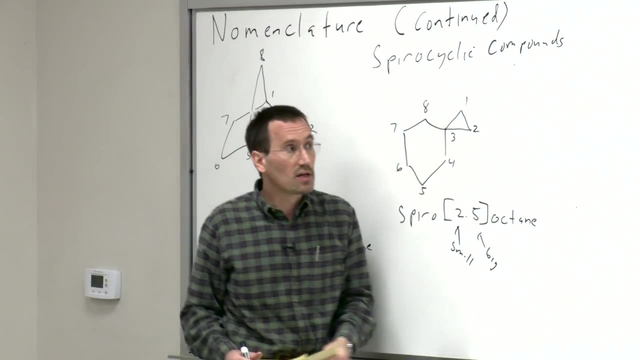 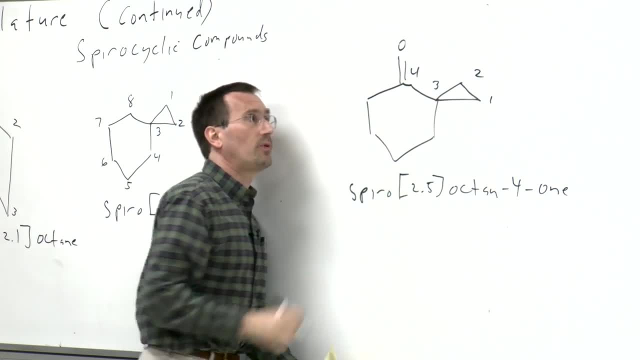 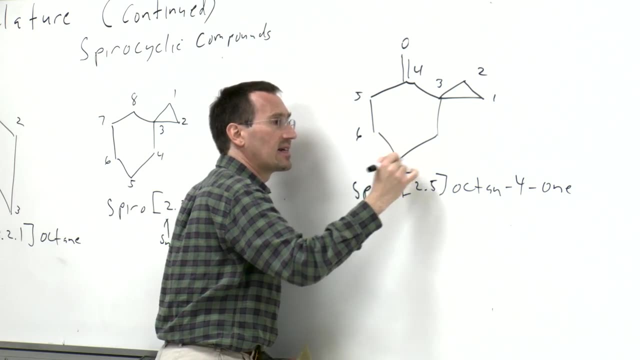 The carbonyl is in the bigger ring, so we're going to place the carbonyl at the lowest number possible. so we just go 1,, 2,, 3,, 4,, 5,, 6,, 7,, 8.. 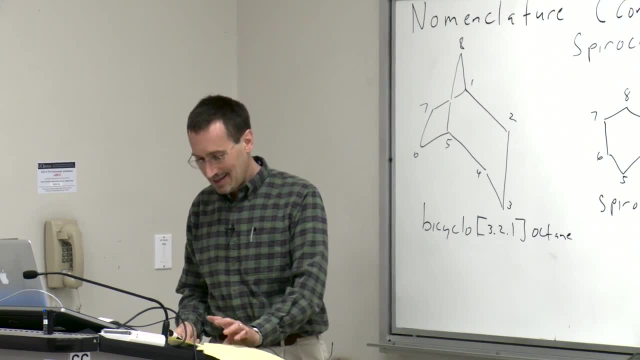 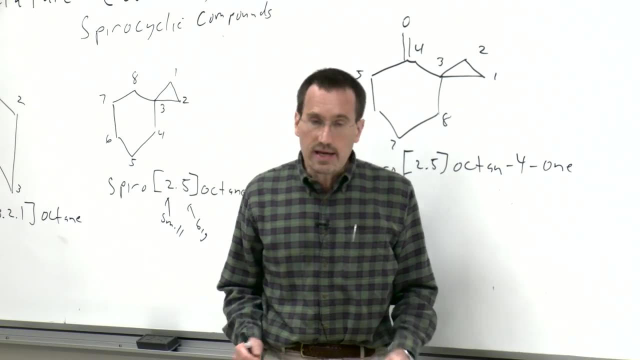 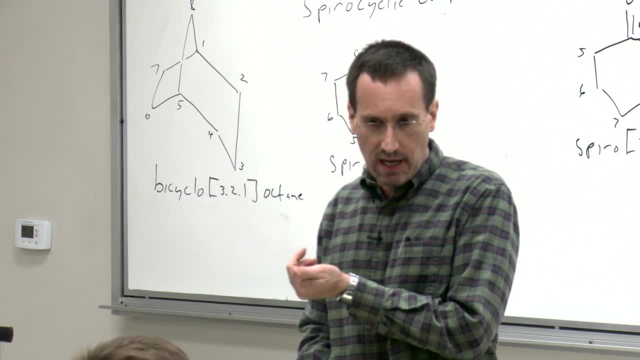 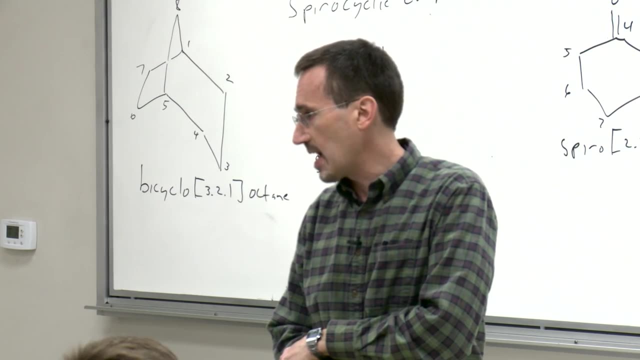 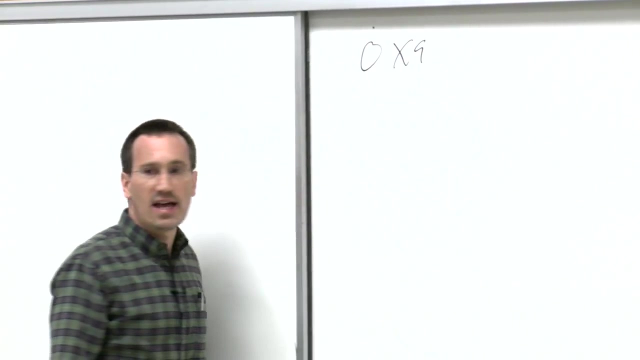 for replacing atoms, and I showed you oxa, asa and thia. These are terms that are actually worth knowing. They roll off organic chemists' tongues And I also cautioned you when I said oxa, that we have an A in the end. 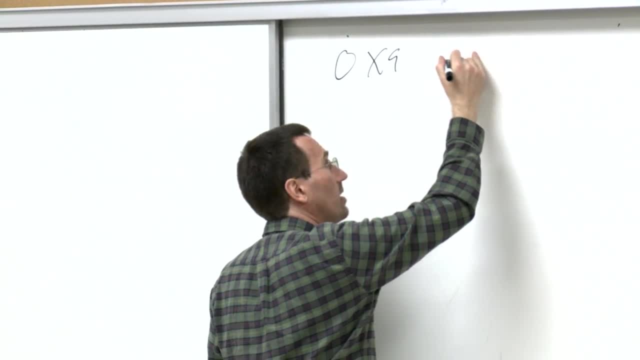 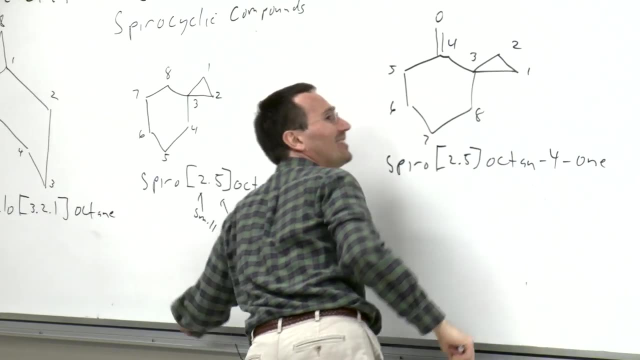 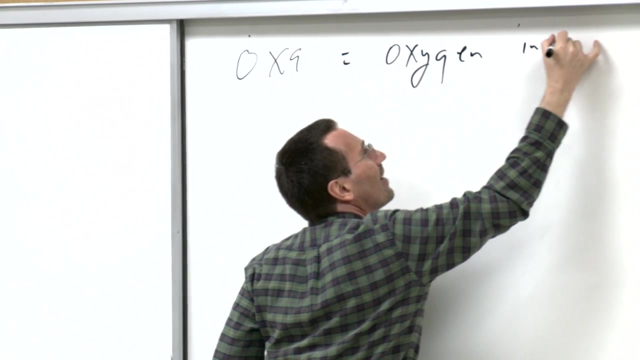 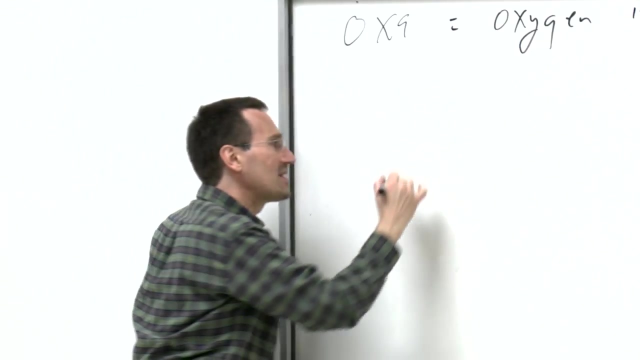 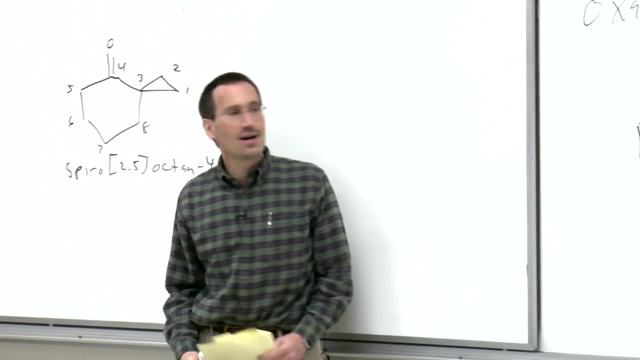 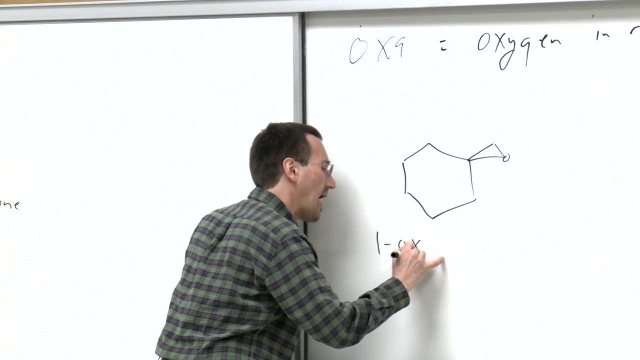 And that it means an oxygen in the ring. Oops, Jeez. So, for example, if we take our spirooctane example and I put an oxygen in the ring Now, we name that oxygen as oxa, So we're going to call it 1-oxa-spiro-2, 5.. 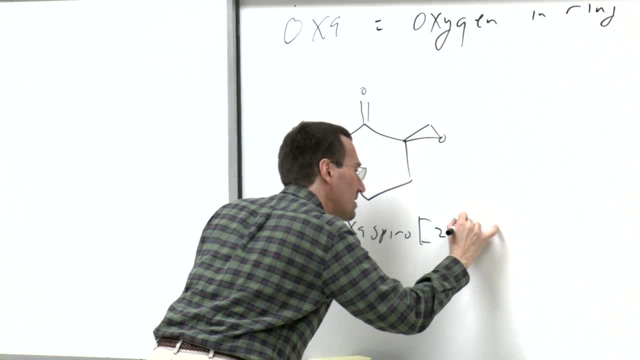 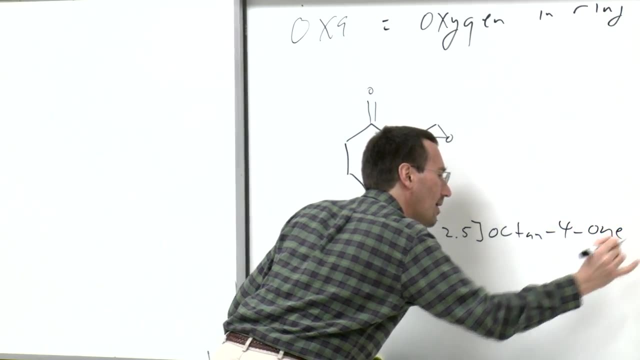 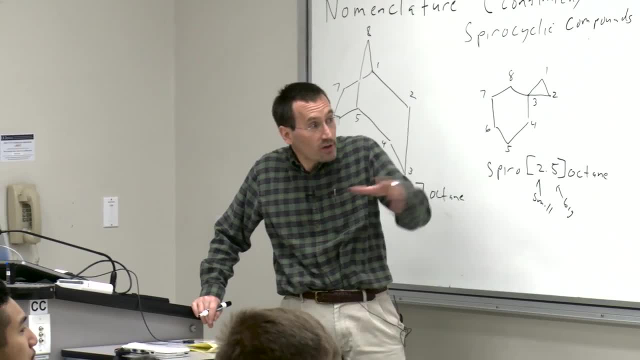 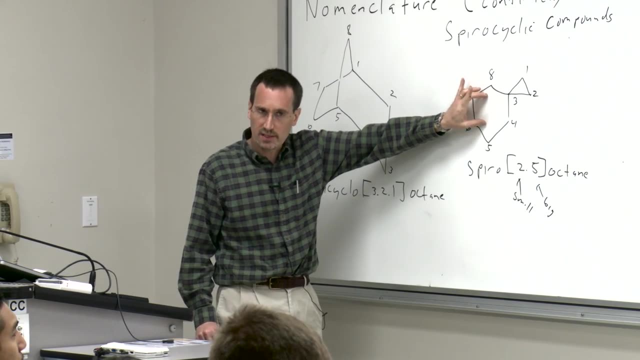 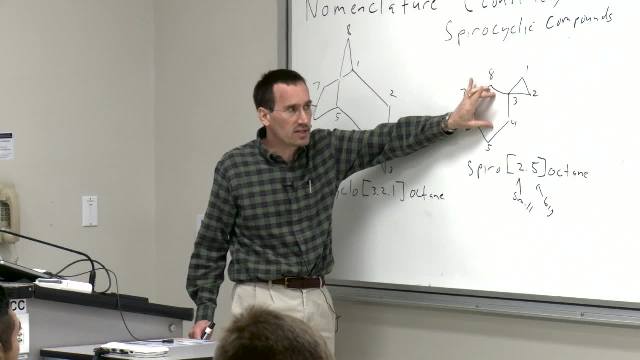 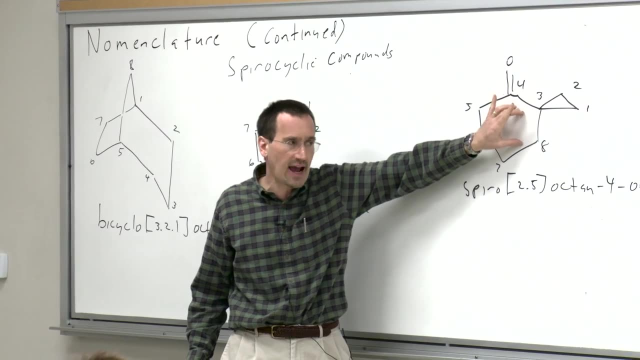 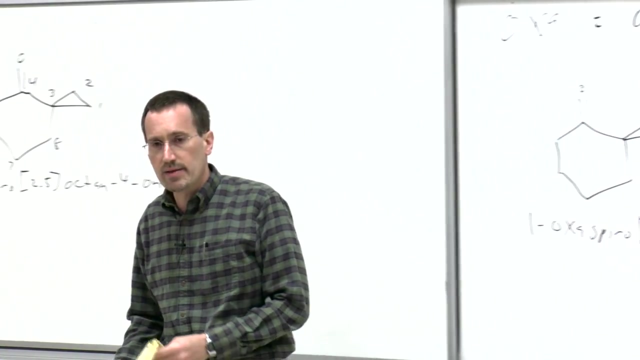 We identified the way we named the parent ring system, We started to modify the parent ring system. When we saw the modifications are tacked on, we continued to modify the parent ring system and we just tack on the modification. Is there a reason why you added the 1 in front of the oxa? 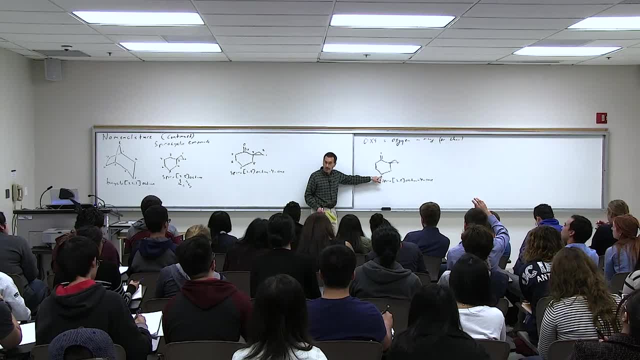 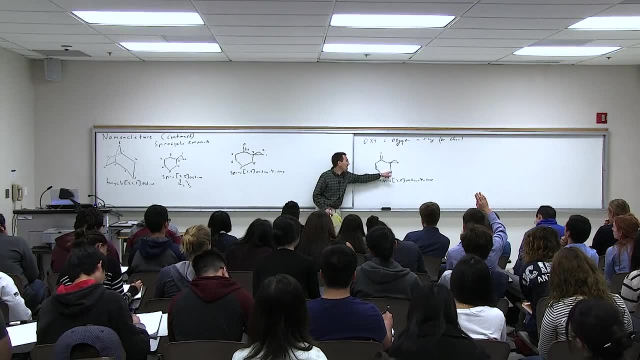 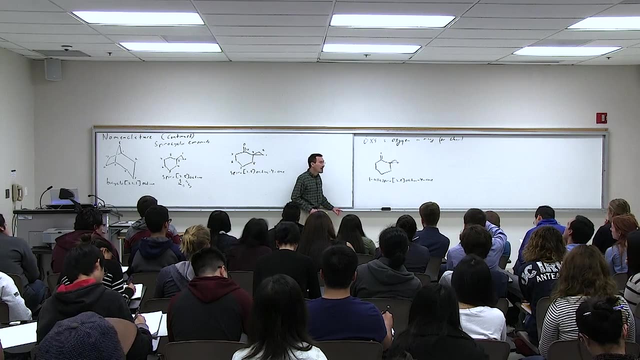 Yeah, because we could have had the oxygen over here, in which case we would have had a different number for it, or we could have had it over here or over here. So yeah, there is. Why is it so often that you only have 7?? 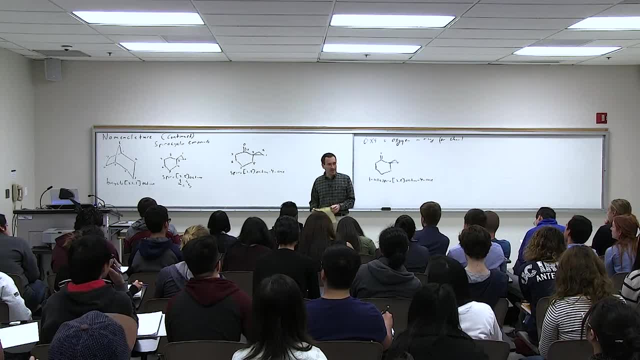 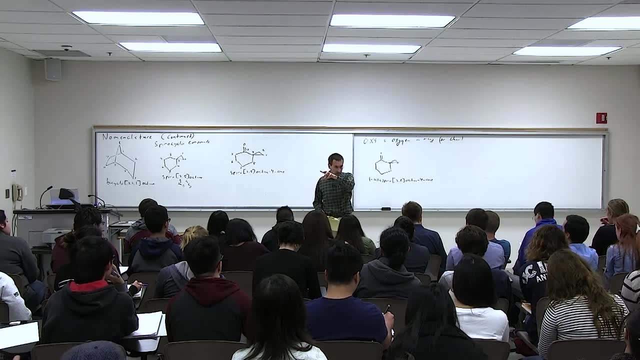 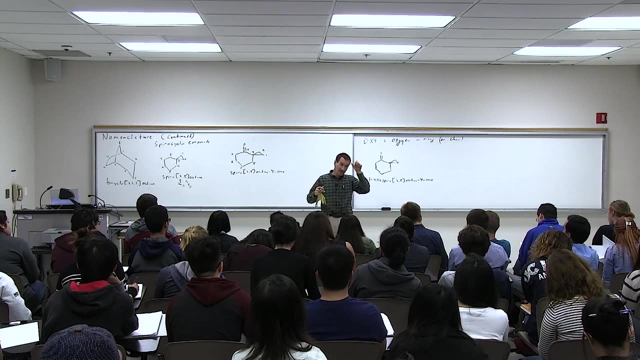 Because the parent- and we saw this last time when we went to the oxa-bicyclo-221-heptene system- it's the parent system, which is that number of atoms- 8 atoms- and then it's replace 1.. 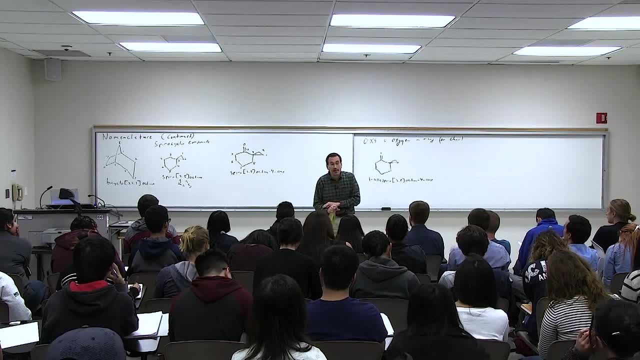 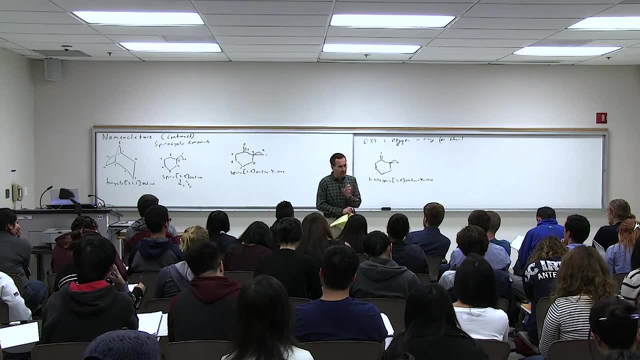 And these are good questions- And the bigger picture here. I'll come to you in a second. the bigger picture here is not necessarily remembering all of the nomenclature, although you're right in the middle of the slide. Yeah, You'll be surprised how much you internalize. 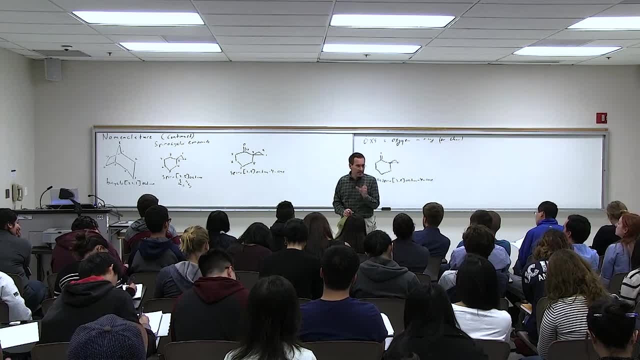 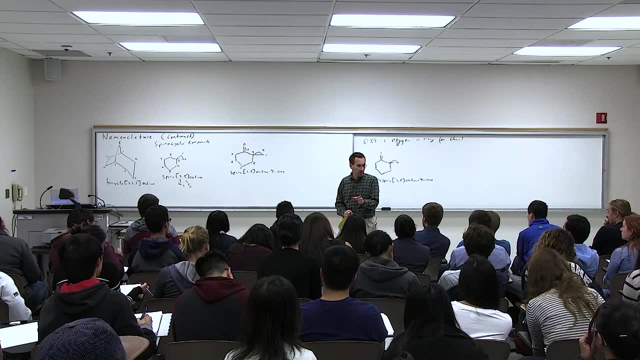 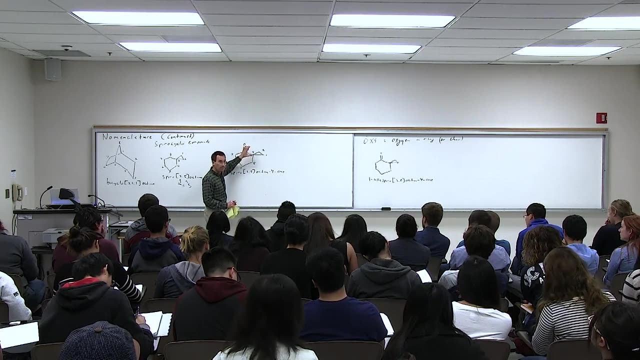 without even trying. The bigger picture is seeing anatomy. It's that you take somebody in the 51A course, in the introductory sophomore course, and they're struggling to see a ketone functional group if you just draw something. That's the level of mastery. 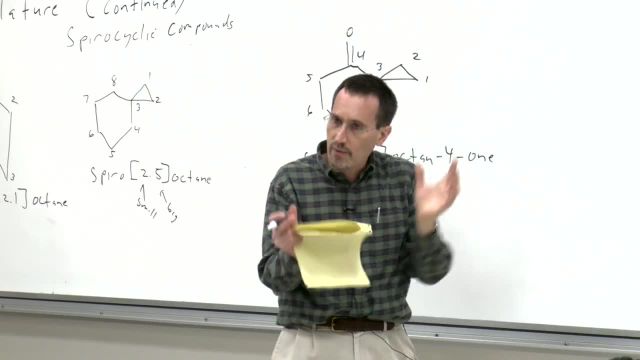 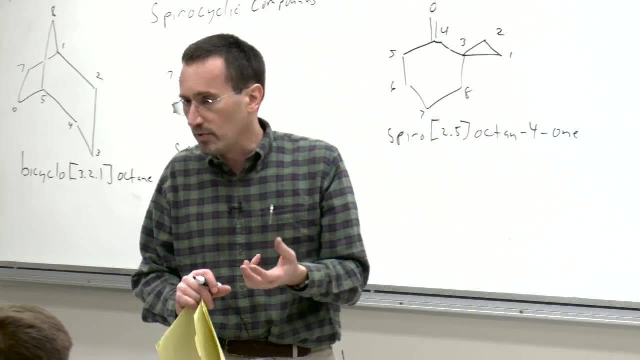 And now we're starting to see this progression of: oh yeah, we've got this ring system. It's built up of this and this, and so when you start to go to really profound molecules like morphine, which is one that I use as an example a lot in teaching- 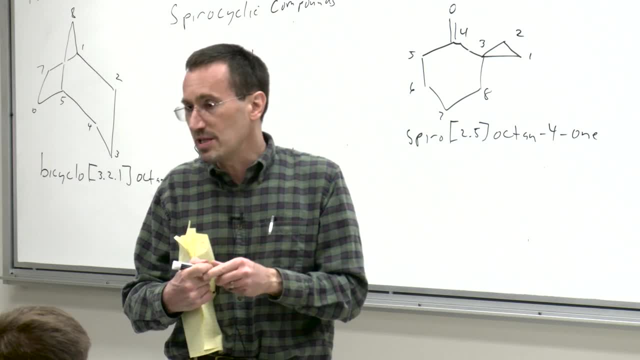 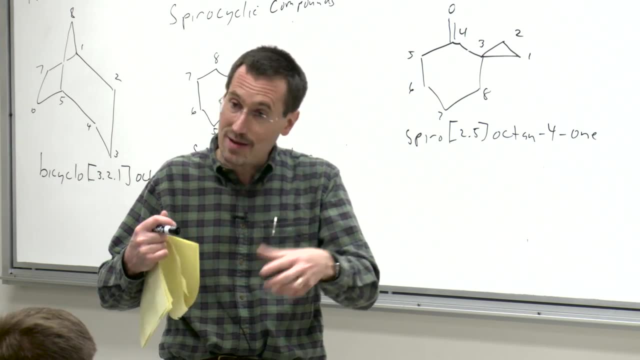 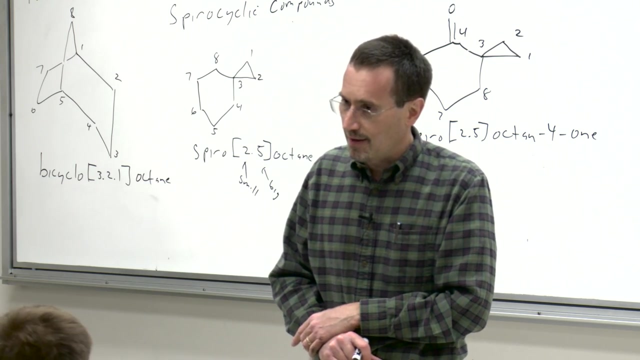 well in teaching molecular modeling course and teaching spectroscopy class being able to see the molecule and its components and its shape all fit into that real inside the head understanding of organic chemistry. So is that the idea of pi 2 y is 2, 5 instead of 1, 5?? 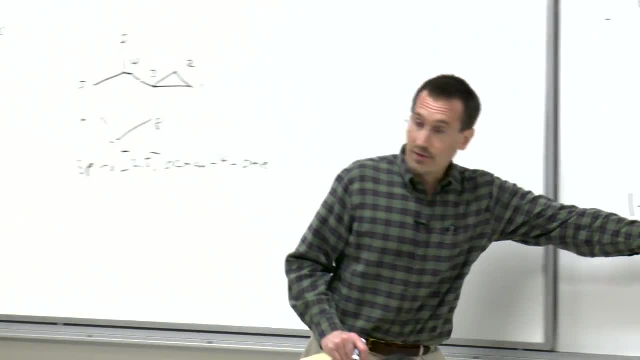 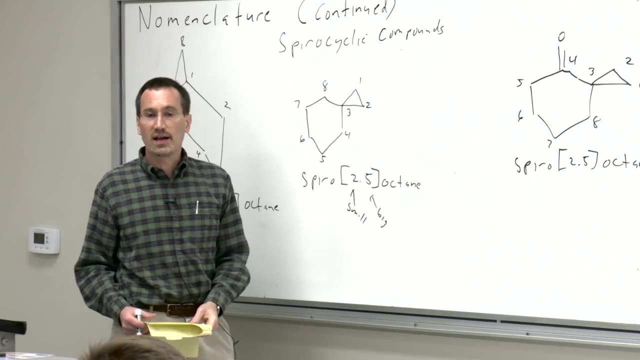 Is it only 1?? Yeah, It's the same idea, absolutely, absolutely. We started with the parent and then we just keep, or the parent and then we just keep, modifying and modifying. Yeah, Wouldn't it be different to happen if both of the carbons? 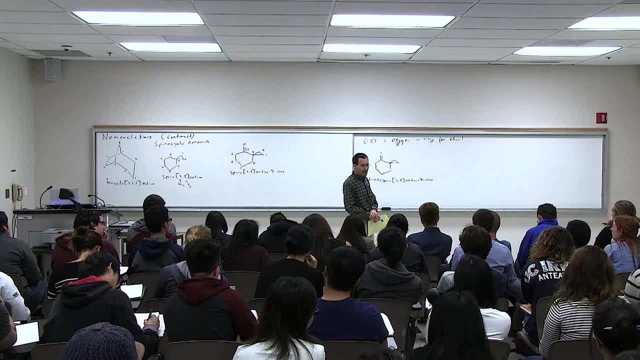 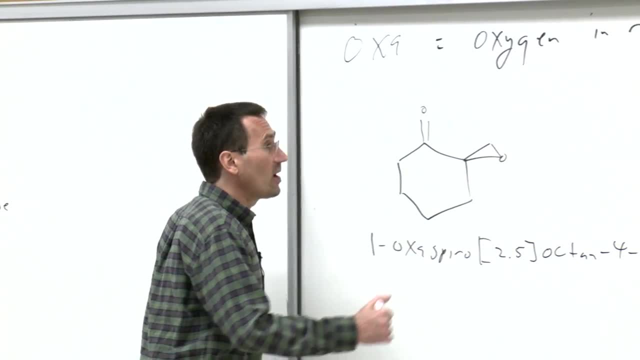 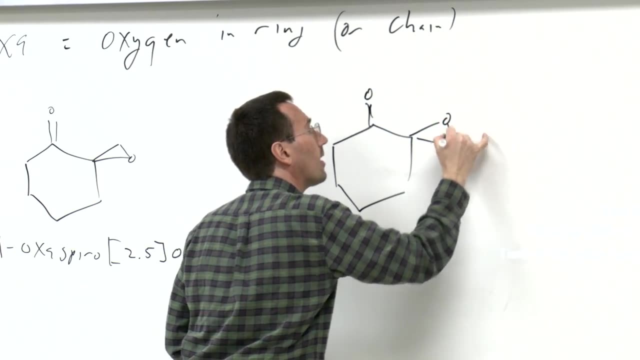 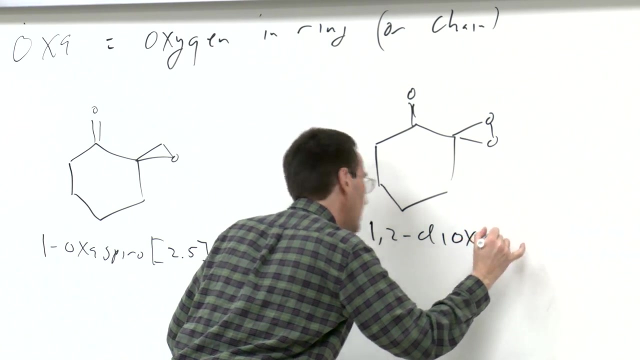 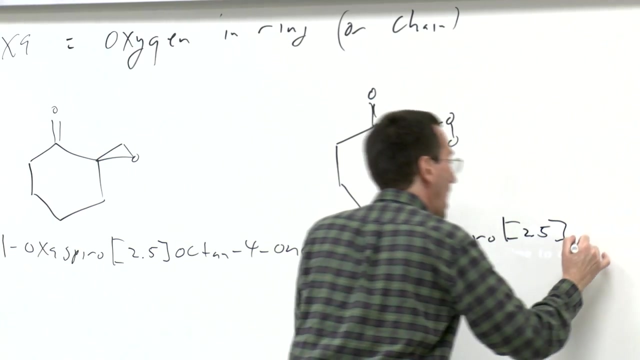 on the three-membered ring were a set of oxygens, because the oxygen should be adjacent. So that's a great question. So then it would be dioxa. So if we went ahead and Did this, it would be 1,, 2, dioxa, spiro, 2, 5-octan-4-one. And again seeing, oh. 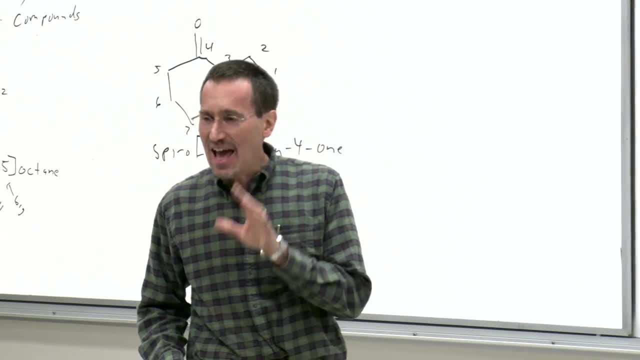 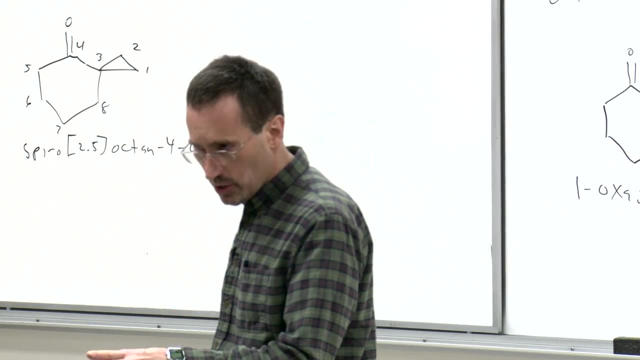 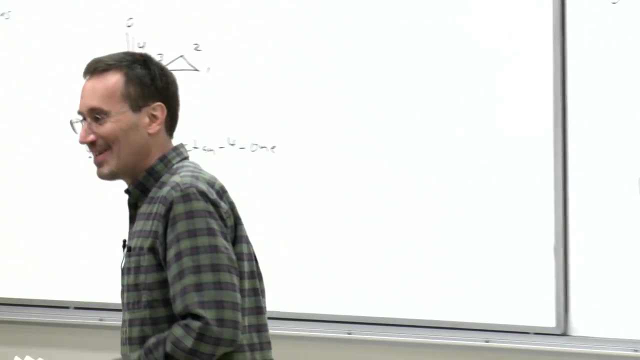 And again, seeing that anatomy and being able to see that anatomy is really profound and that's essential to our thinking. So I'm going to draw a really horrible, horrible molecule based on, based on this question. 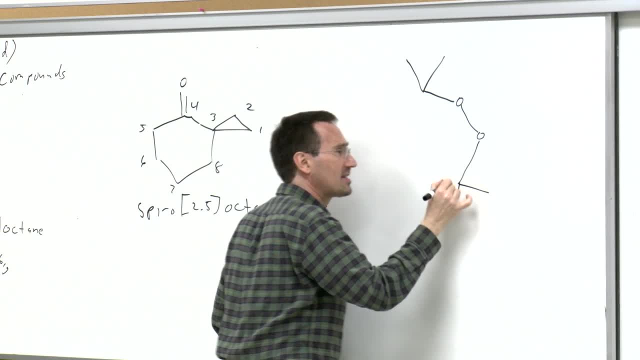 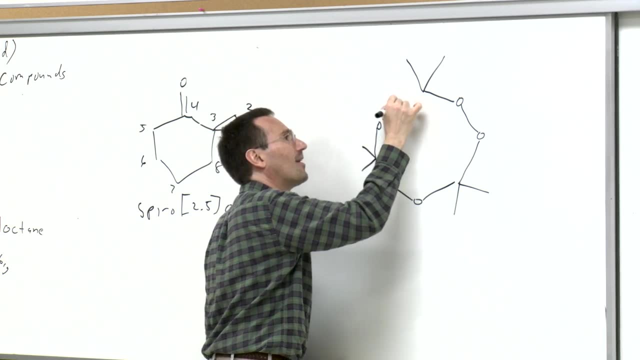 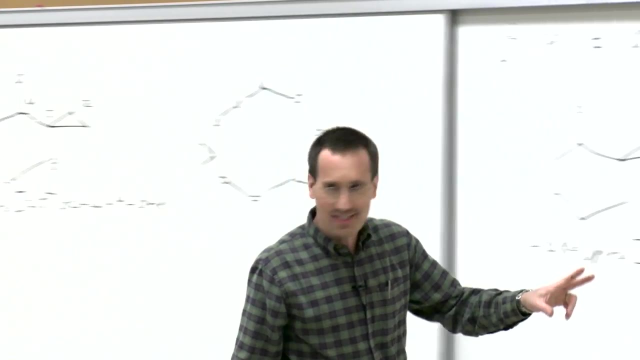 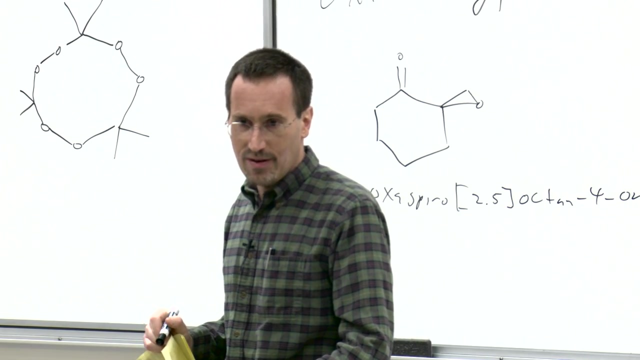 I wasn't planning on drawing this. I'm probably going to get arrested for doing this. All right, does anybody know what this really, really horrible molecule is that has these two oxygens next to it? Yeah, it's explosive. What is this? 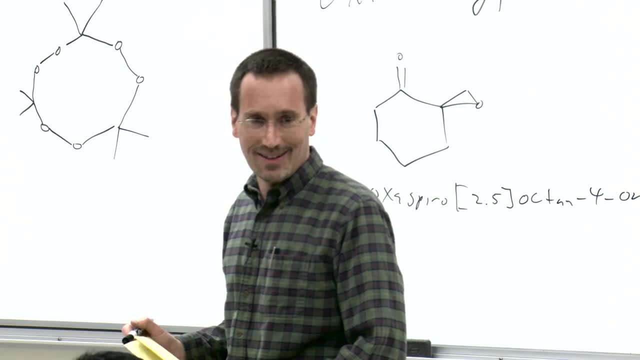 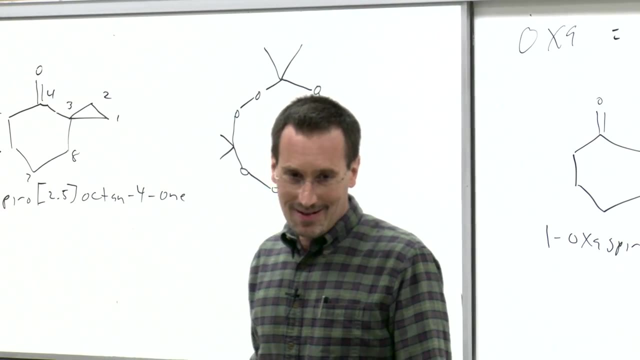 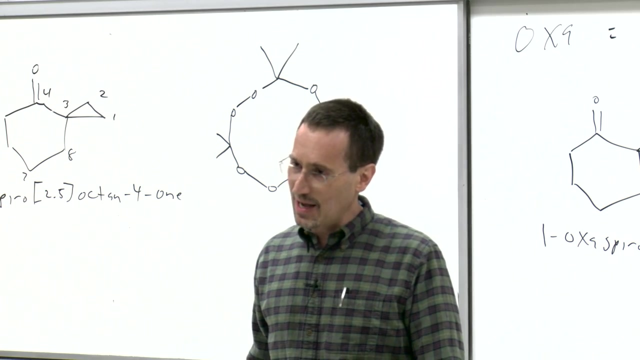 Yeah, What TMS? No, No, TMS from isotope and the you know, hydrogen peroxide. Yeah, it's acetone and hydrogen peroxide. This is the triacetone triperoxide that's going in these suicide vests, you know. 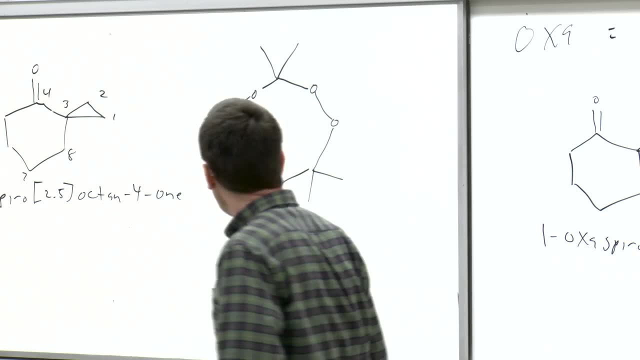 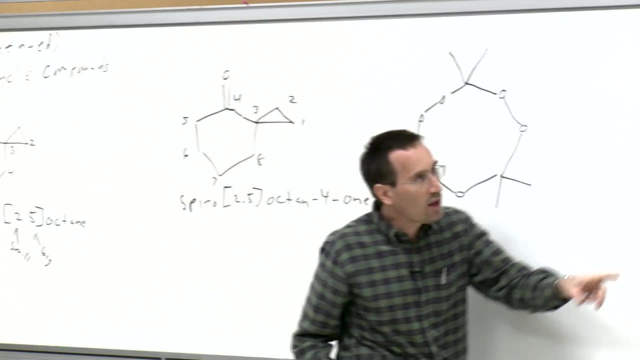 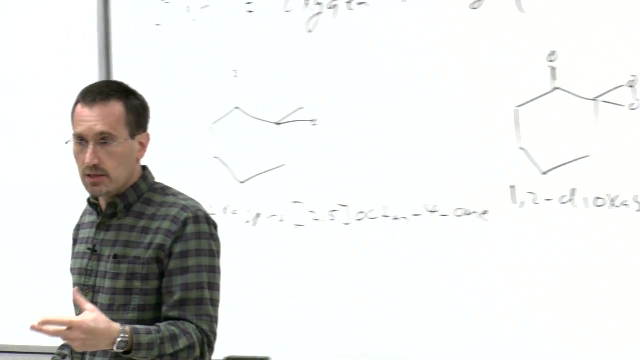 which have been wreaking havoc with terrorists. Now come to take this molecule for anatomy for a second And we start to see a couple of things. First of all, as we saw over here, this is a peroxide linkage. In other words, you can see now as an organic chemist. 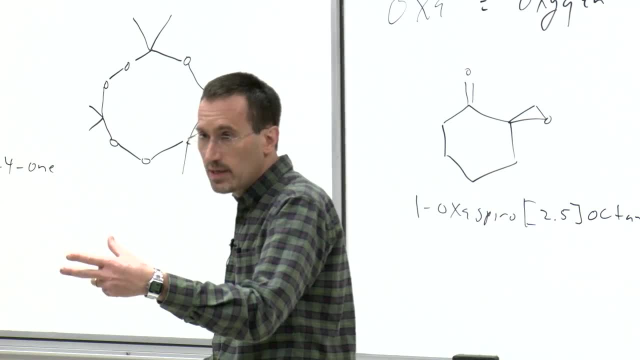 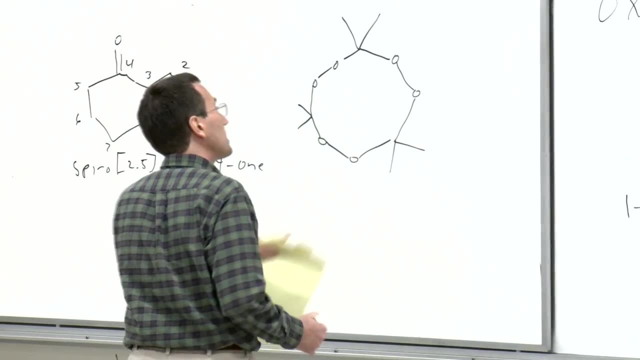 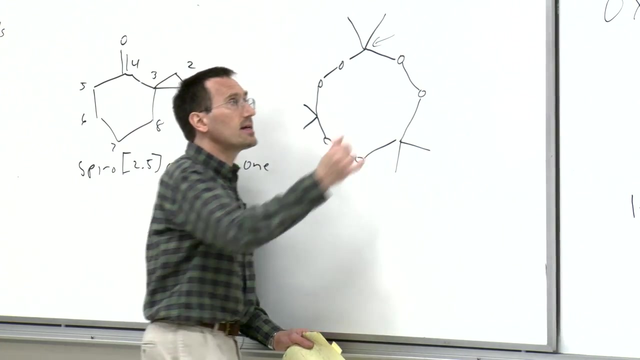 and as somebody who's been steeped in organic chemistry for one year and or you know, three quarters plus two lectures, you can start to see: okay, wait a second, I can understand this functionality. here is an acetal. In other words, you can start to look at this and say: 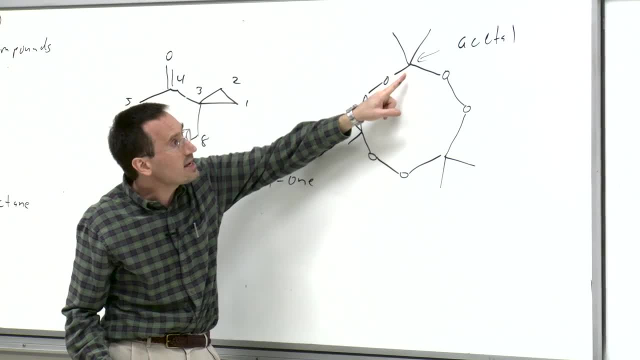 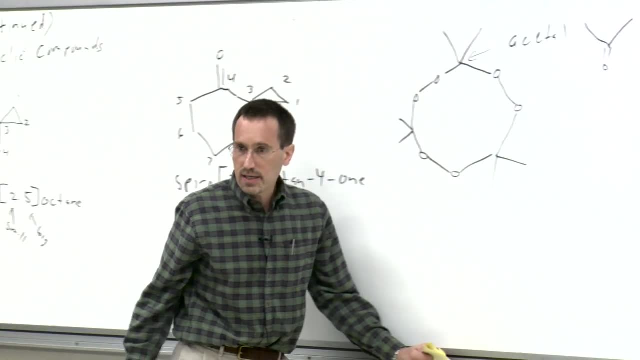 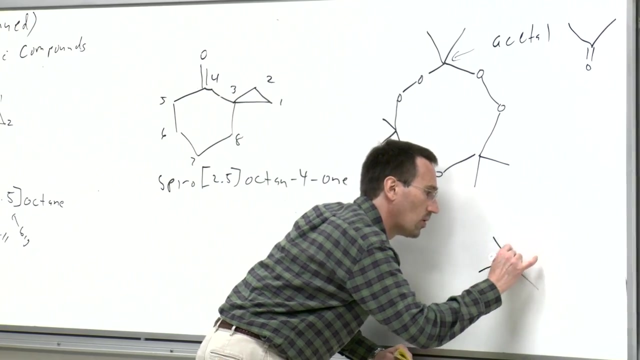 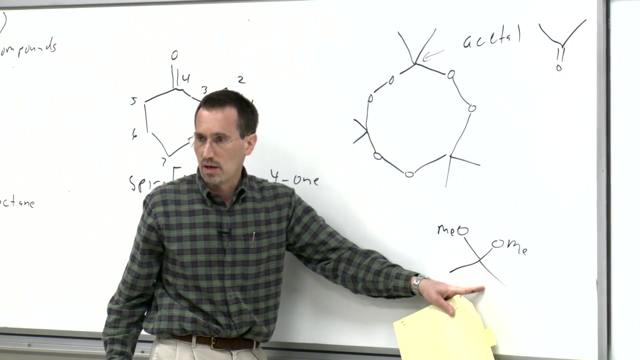 oh wait, a second: The anatomy. The anatomy of this molecule is an acetal of acetone and it comes here. It's an acetal right. If you have this molecule, this is an acetal of acetone and methanol right. 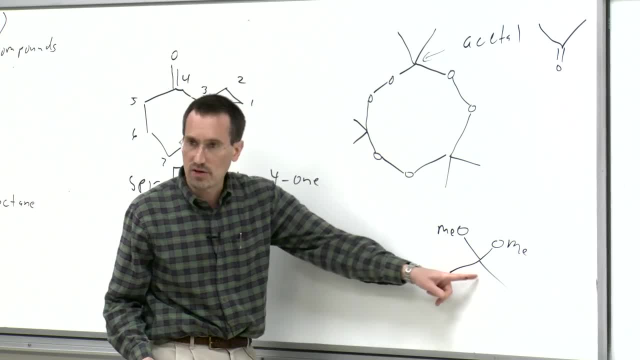 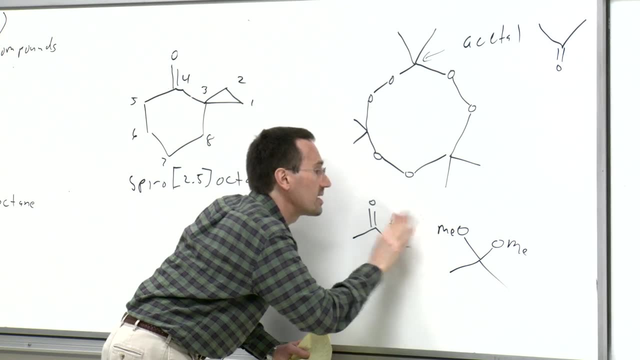 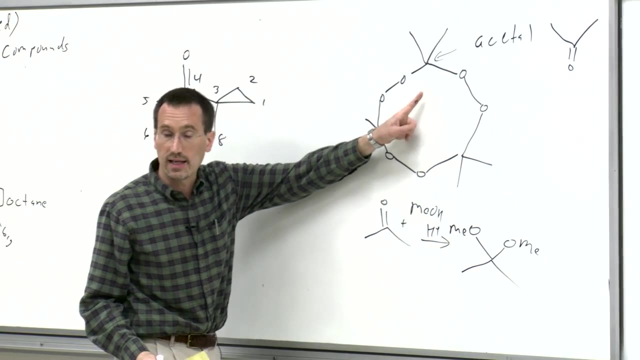 And you learned, you made that, you formed that by methanol plus acetone. I'll write it in the same way. I'll write it as M-E-O-H with acid catalyst, And so you can start to say: oh wait a second. 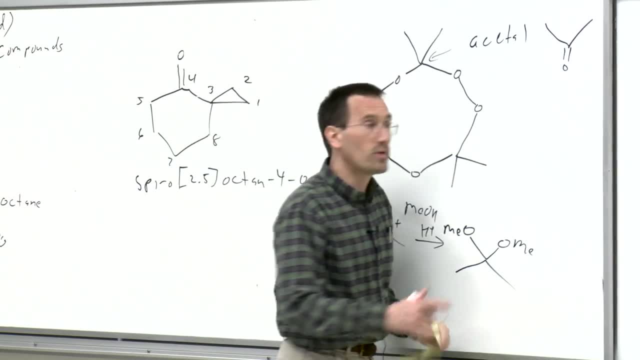 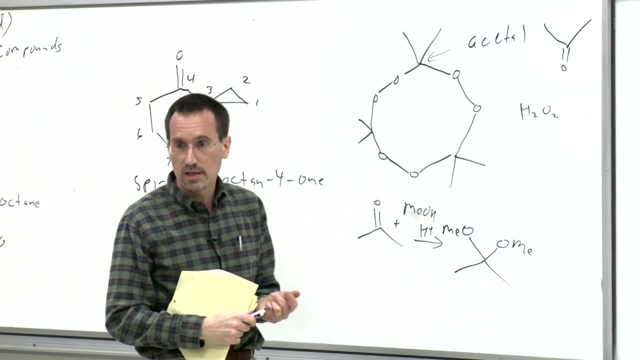 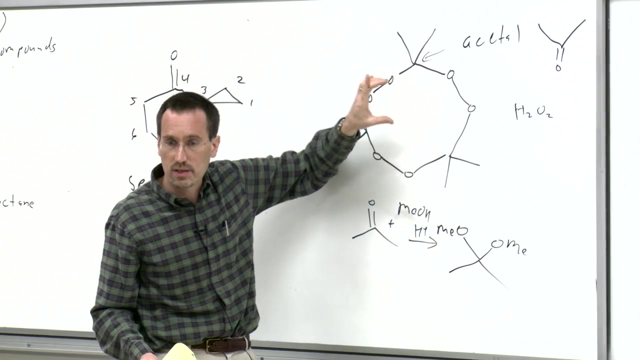 This is an acetal of acetone and hydrogen peroxide, And that's what makes this really scary is, basically, you can get these ingredients in a hardware store and a drug store, And so this is very accessible. But being able to look at this molecule 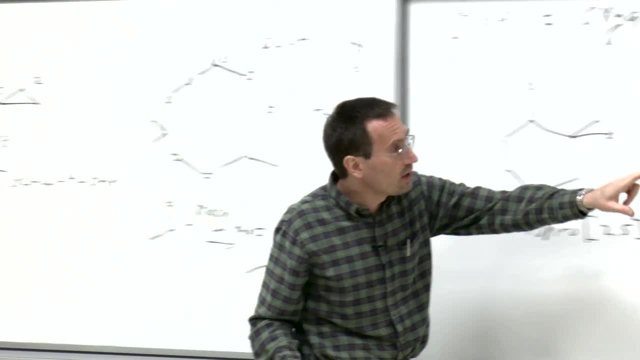 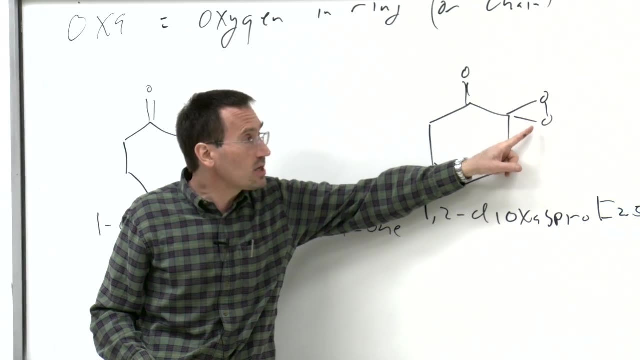 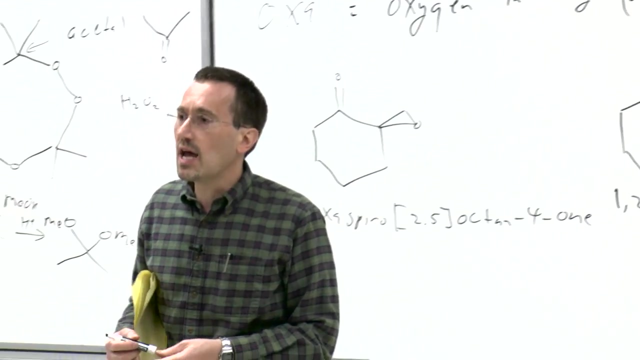 and assimilate the anatomy. being able to look at this molecule and assimilate the anatomy is what we're talking about right now, And reagents like this get used as oxidizing agents in organic chemistry. And when we come to chapter, I think it's six- 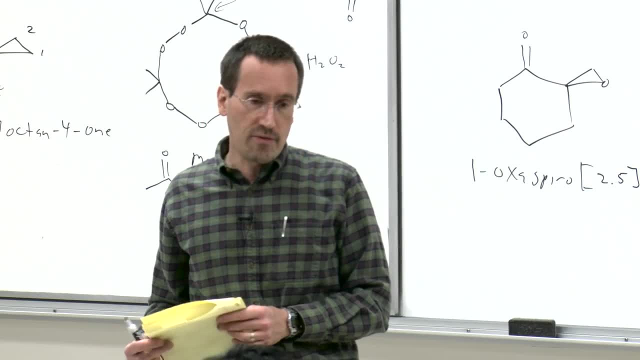 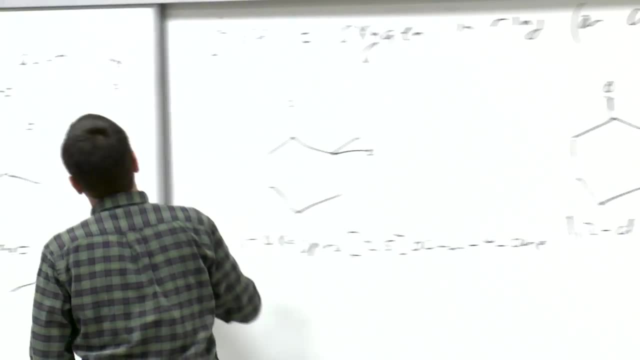 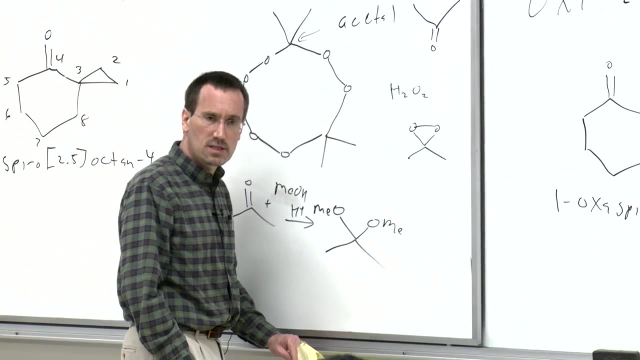 on functional group transformation, you'll learn about various reagents. I don't know if we're going to cover the. I think it's just the acetone. I think it's the monoacetone peroxide. Sebastian, do you remember the oxidizing agent from synthesis? 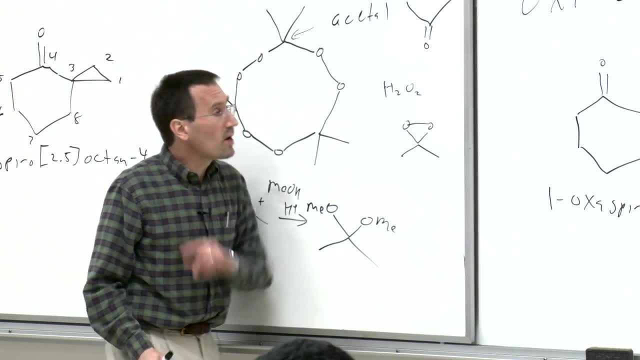 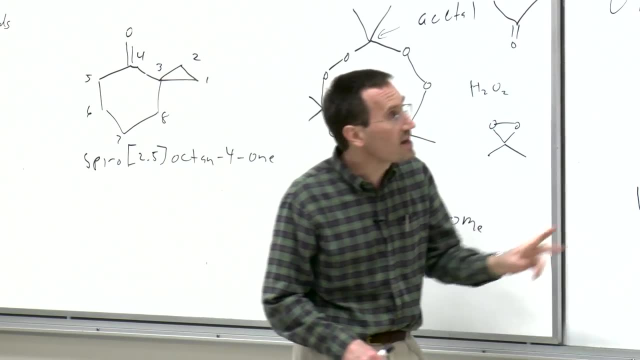 I think it's this one. Anyway, basically, we'll start to see. But yeah, so we start to understand that anatomy and then these reagents make sense. So I want to finish up with what I was juxtaposing here, finish up this little segment. 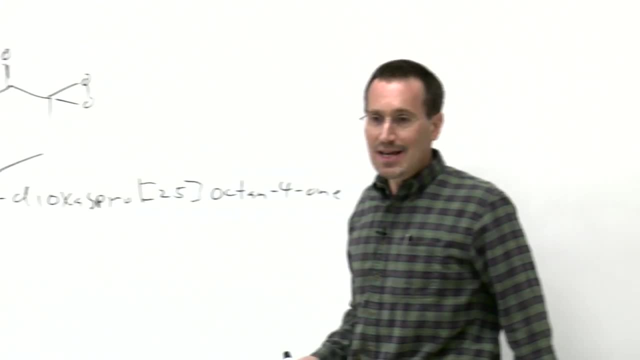 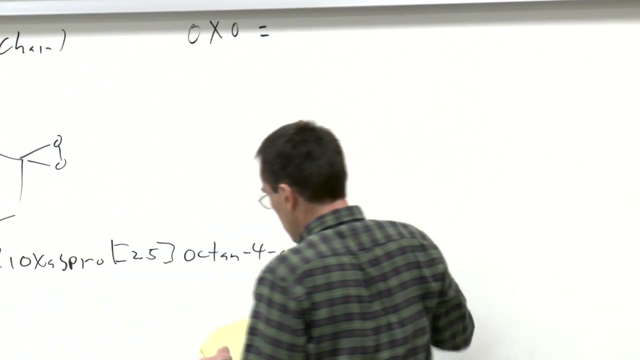 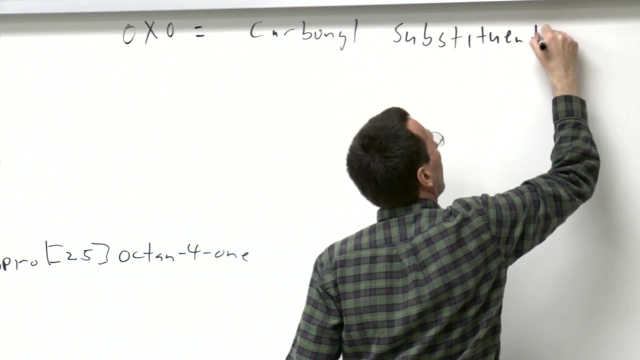 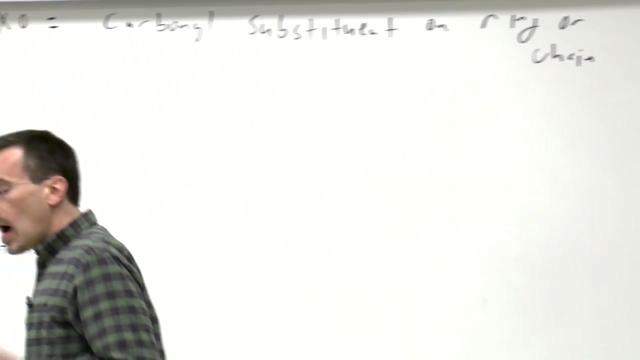 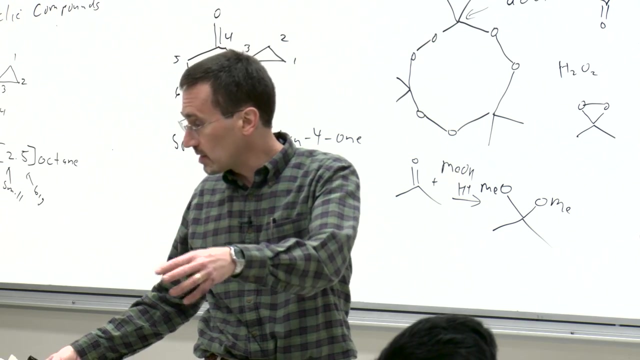 So I cautioned that oxa is oxygen in ring. Oxo is equal to a carbonyl substituent on a ring or chain when you've got a higher priority substituent. So remember I said it goes by oxidation states. You've got alkane at the lowest oxidation state. 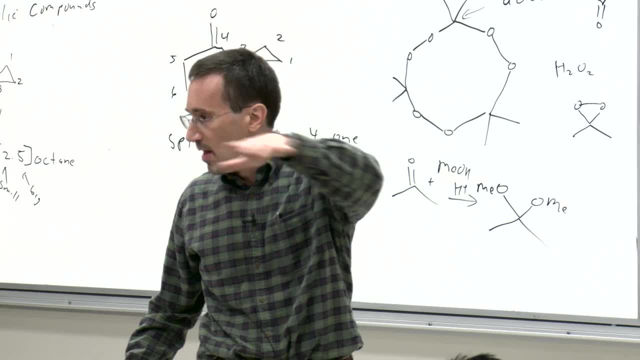 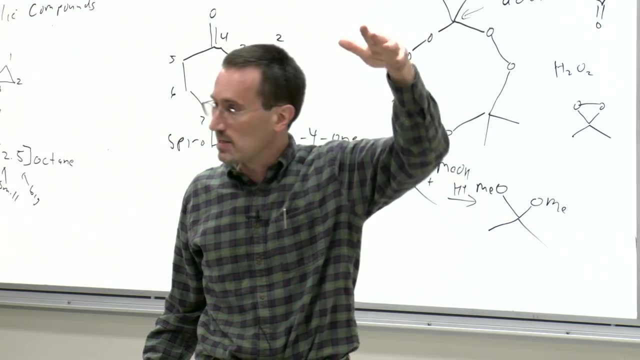 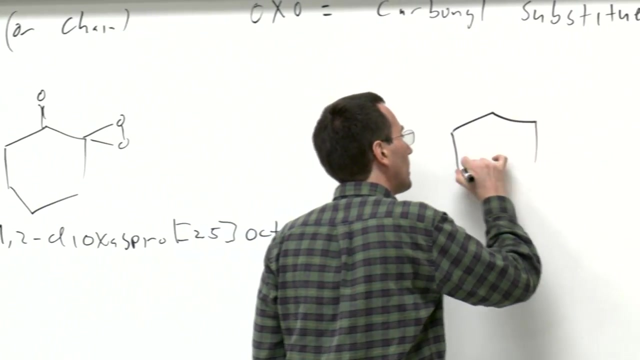 Then you've got the alcohol ether oxidation. Then you've got the ketone aldehyde oxidation state, Finally the carboxylic acid oxidation state. in dictating names, So just to fill things out here and perhaps drive you crazy, or at least drive home a point, I'm going to go ahead. 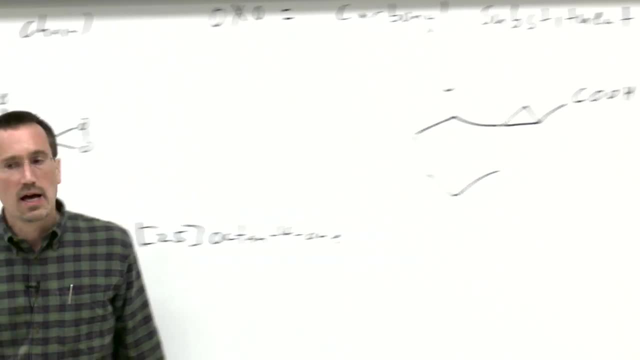 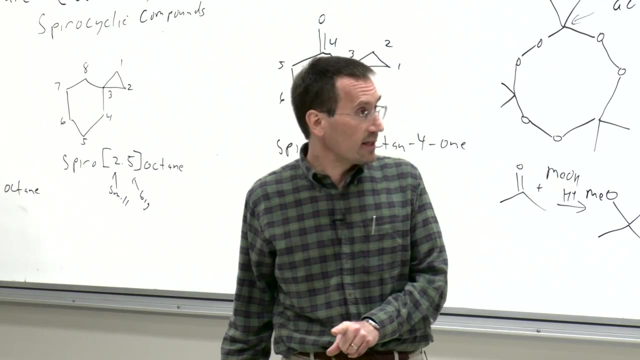 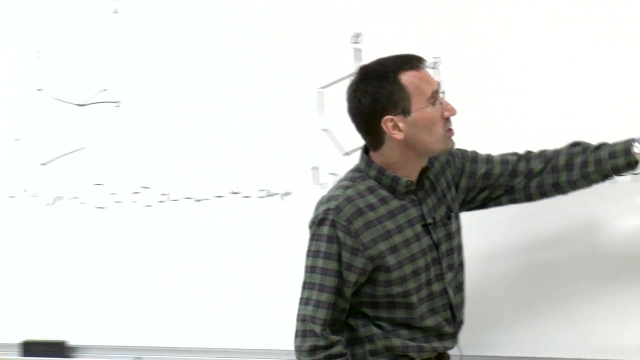 and this is actually really similar to an example in your textbook- and draw out this molecule- And at this point we're naming this molecule as the carboxylic acid- And so it becomes an oxo-spiro-octane carboxylic acid. 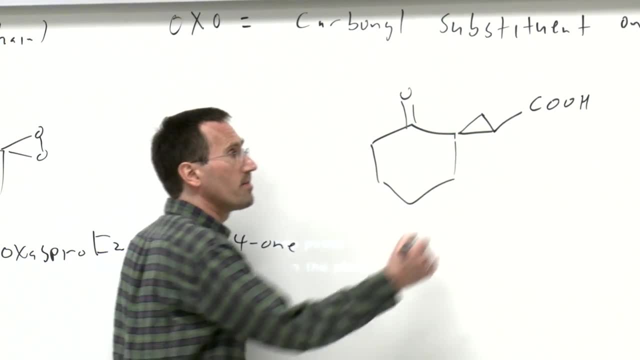 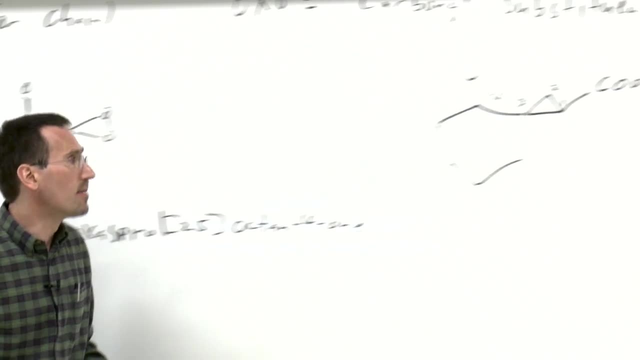 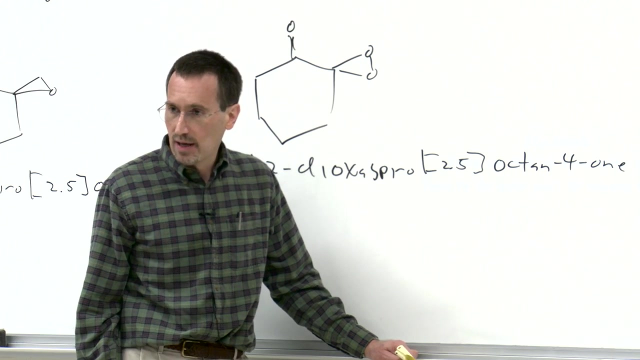 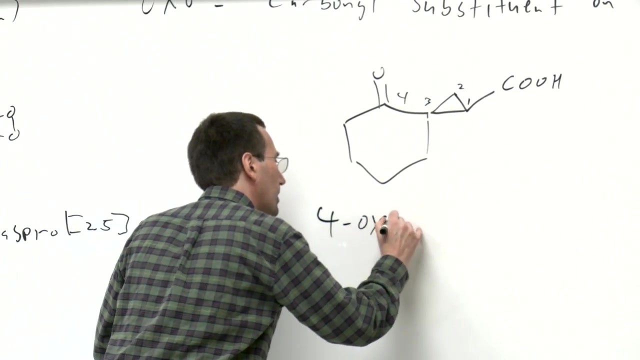 and all of the numbering that we did before, basically putting the lowest number on the smallest chain and putting the lowest number on the substituent and then numbering around as beyond that, to give the functional groups the lowest possible number, And so this molecule becomes 4-oxo. notice: we're using oxo. 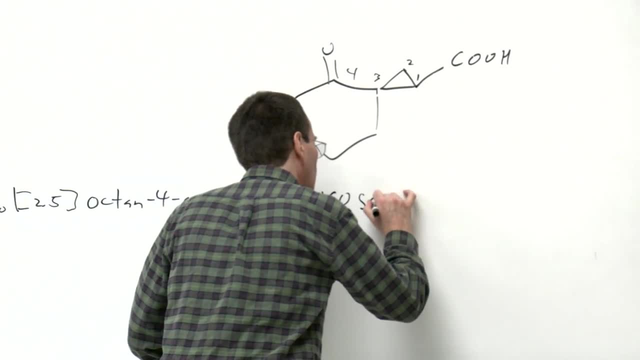 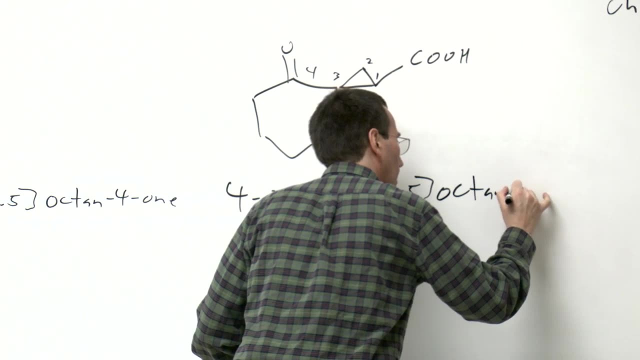 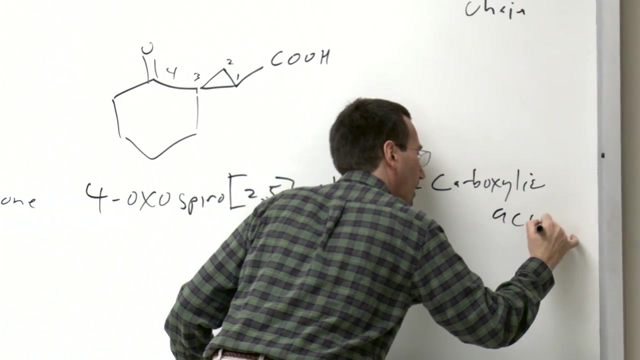 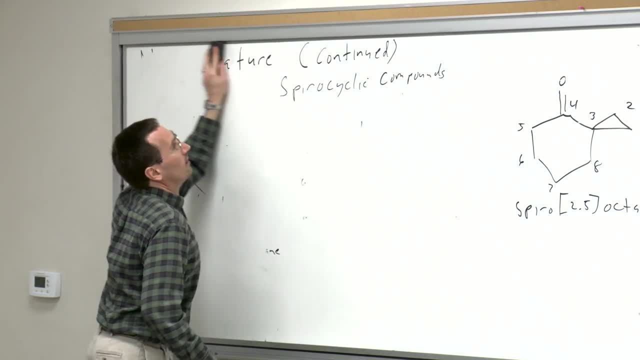 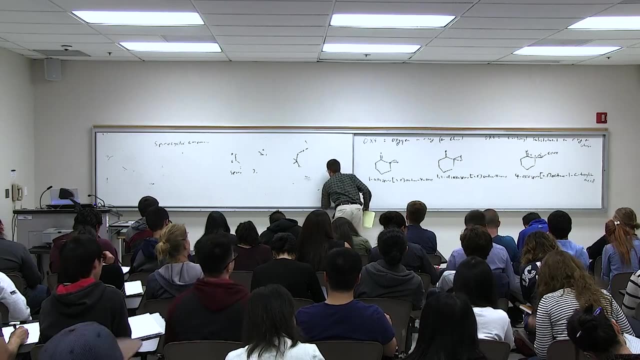 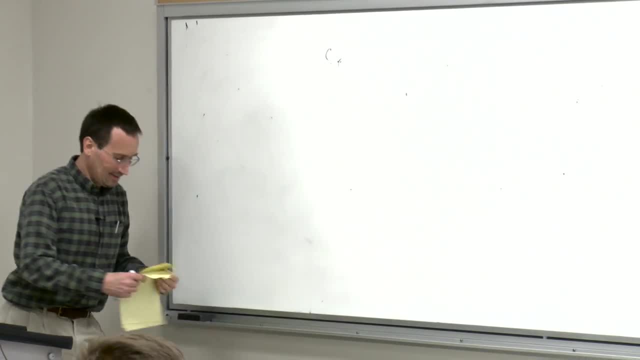 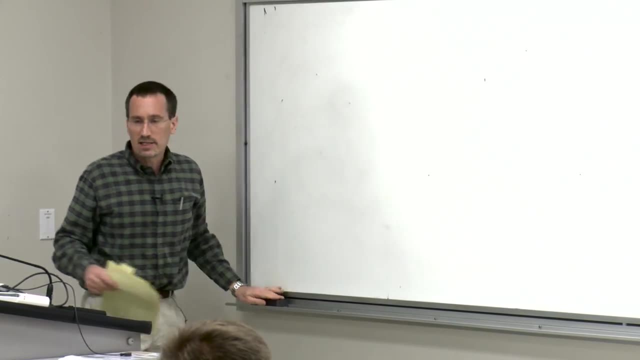 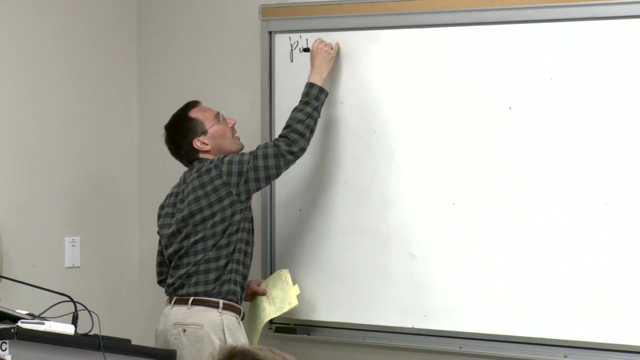 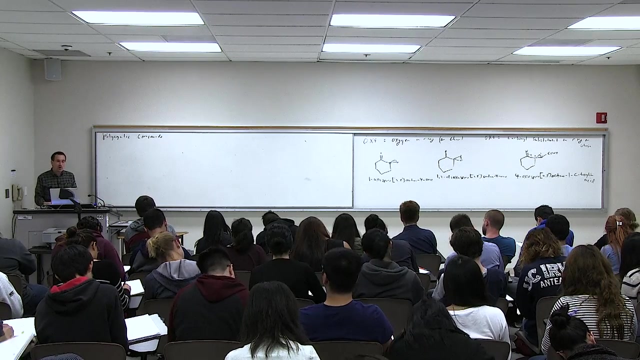 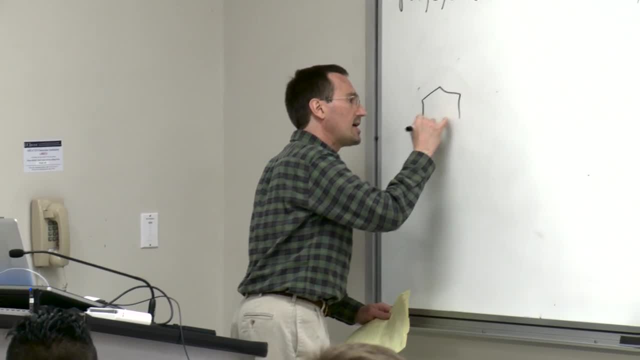 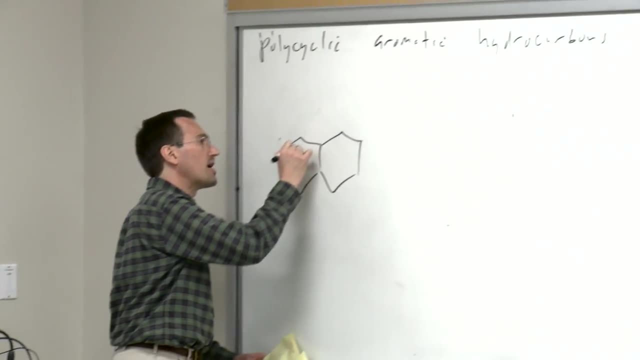 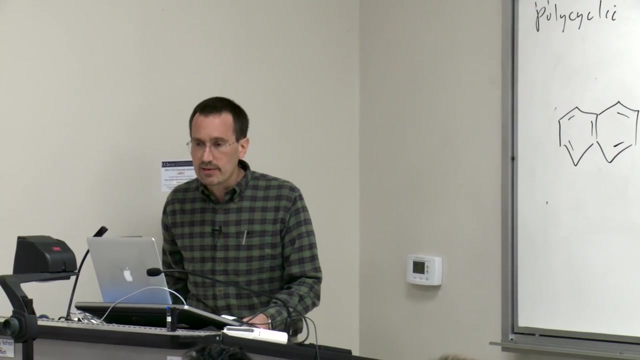 basically taking coal from under the ground, heating the heck out of it without air and boiling off the volatile compounds, And so as you get, you know, so you get benzene and toluene and bigger and bigger compounds. So we've got one compound here. 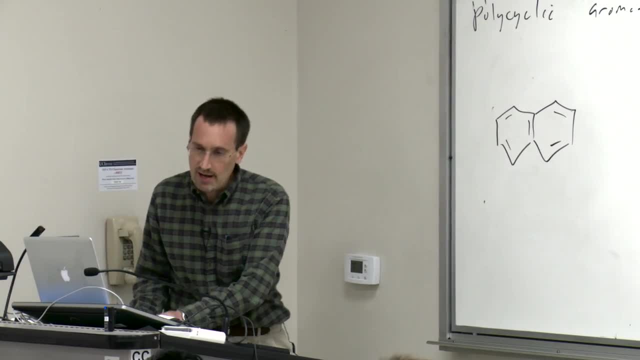 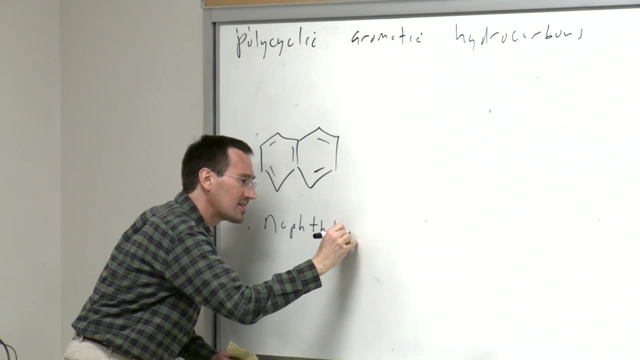 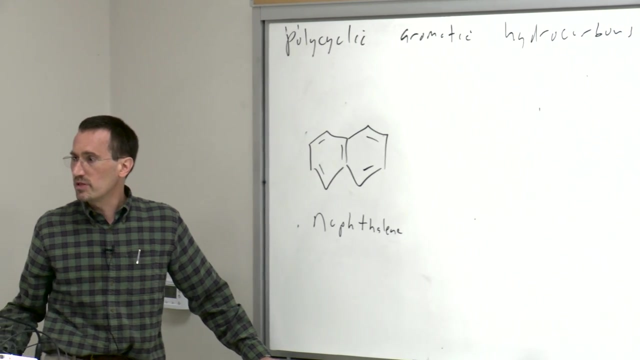 Anyone know the name of this compound- Naphthalene. right, You know where you can find naphthalene, Kind of. I heard somebody say it Muffles. So it's one of the two compounds that's widely used to pack up the compounds. 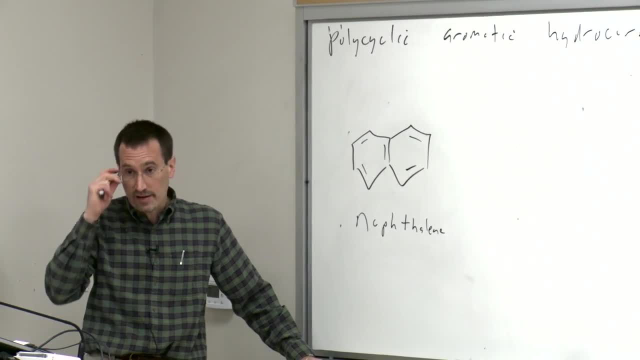 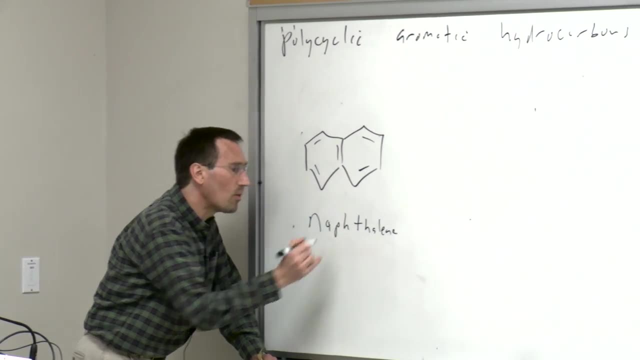 So it's one of the two compounds that's widely used to pack clothes to prevent moths- or more specifically the caterpillars, the larvae- from eating particularly woolen clothes. So what I think I want to do with naphthalene is use this as a starting point. 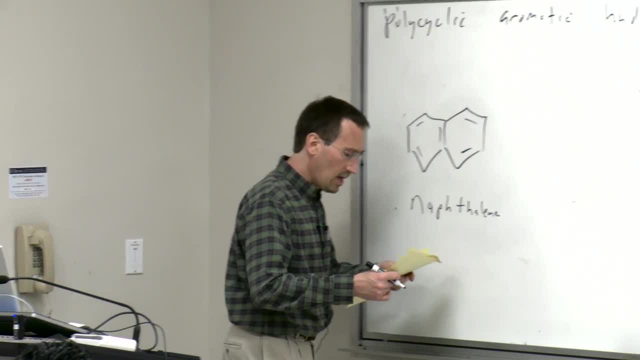 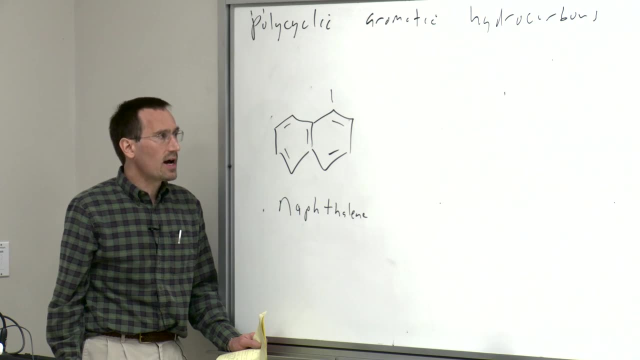 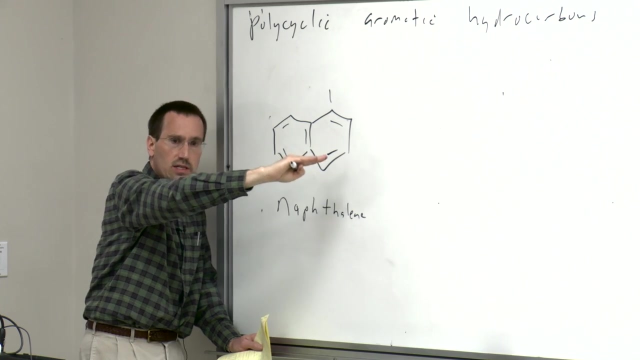 to talk a little bit about numbering and then take us further through. So okay, so you number aromatic hydrocarbons, polycyclic aromatic hydrocarbons, starting in the upper right-hand ring as drawn, And generally you draw them horizontally to put as many rings horizontal as possible. 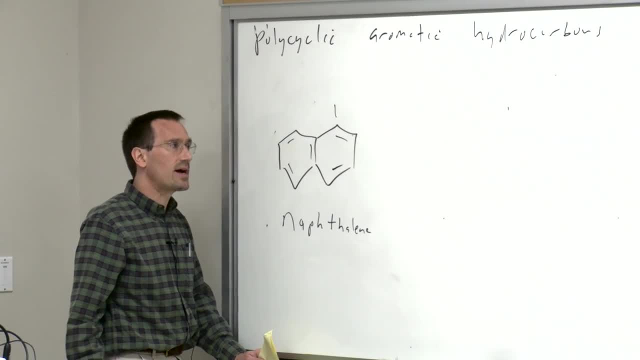 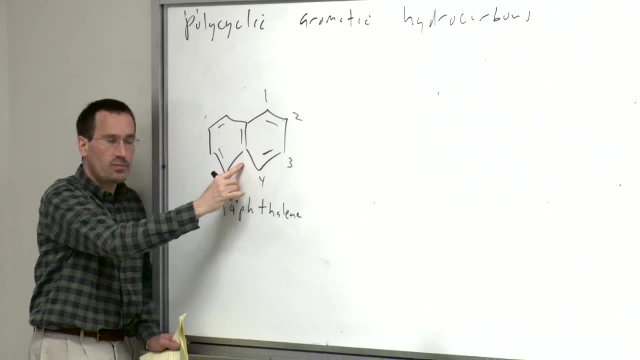 And then, beyond that, try to put as many rings in the upper right-hand corner as possible, And so you start in the upper right and you go around, You skip the ring fusion. So you go one, two, three, four, five, six, seven, eight. 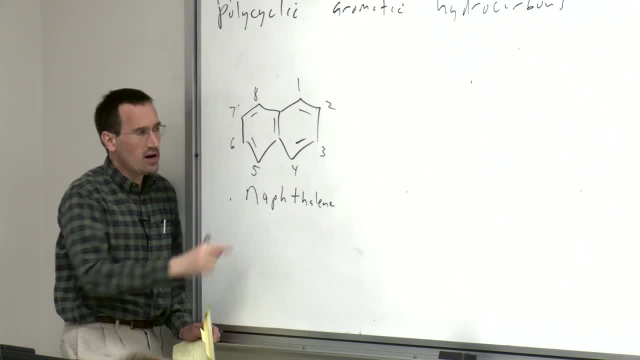 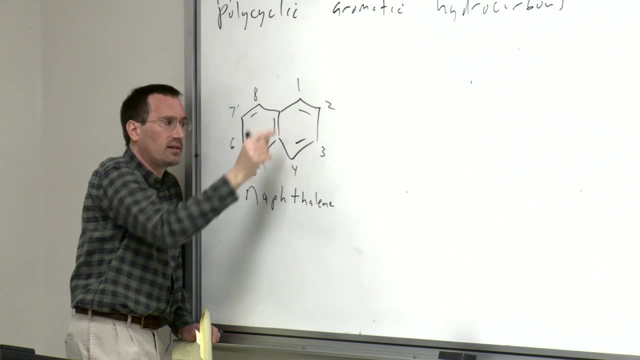 And then the ring fusions sort of get a lower priority because there's nothing happening. In other words, I could make- you know, I could make- 2-chloronaphthalene or 1-chloronaphthalene, But as soon as I put a chlorine on this carbon which is fully valent, 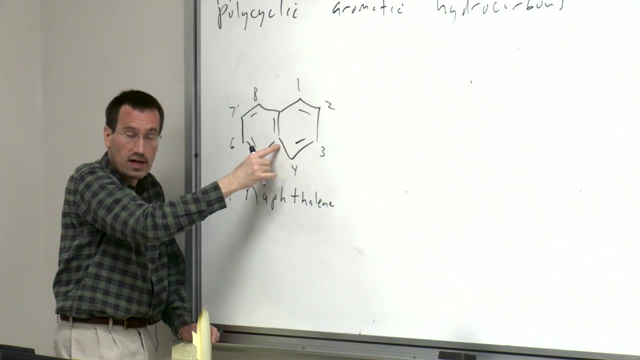 in other words, I can replace a hydrogen here, but then I break unsaturation So I can't make a, say, chloronaphthalene at this position. It becomes a hydronap, you know, chlorohydronaphthalene. 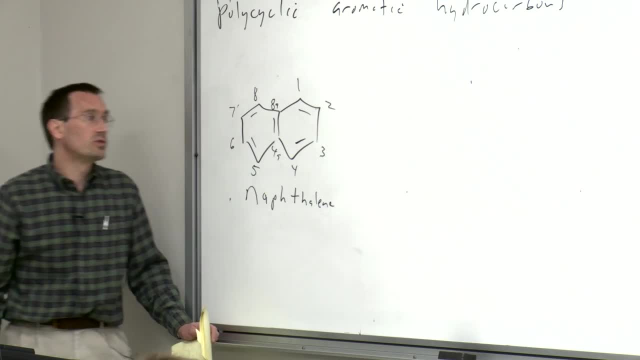 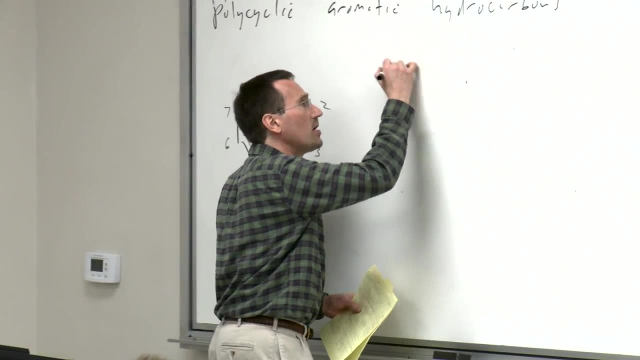 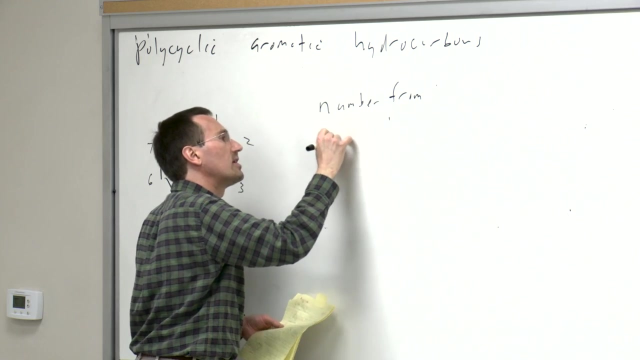 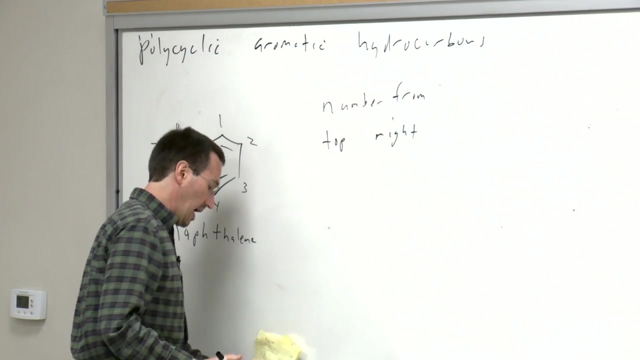 So we give a lower numbering system and we call those 4a and 8a. So I'm going to write here and sort of jot number from top right so you have it in your notes as drawn and I'll show you. as I said, it's tried to draw as many rings as possible. 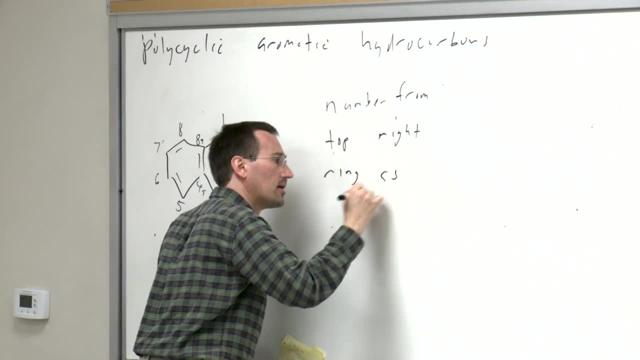 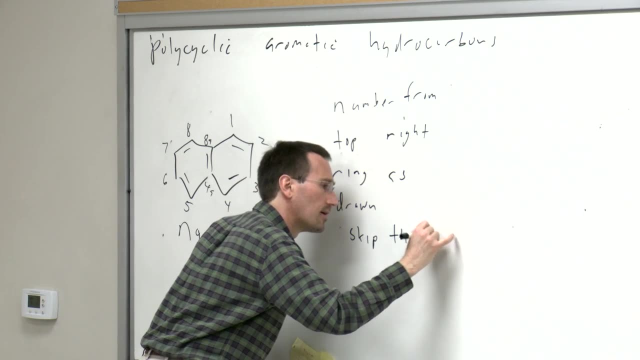 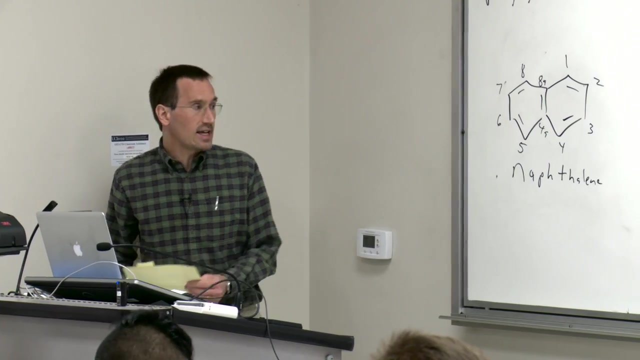 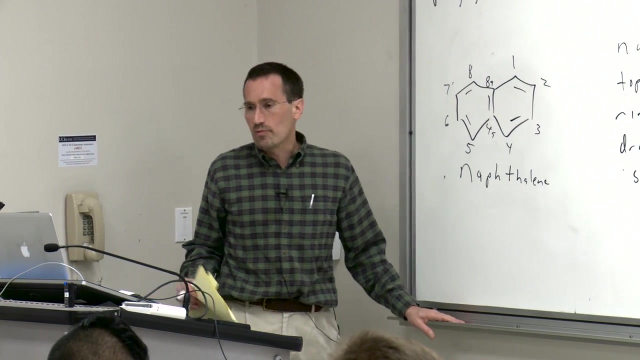 Top right ring as drawn and skip the junction, Just like we did with naphthalene. I guess I'll say: you know, junctions, fusions, whatever. All right, There are three that probably roll off my tongue very easily as an organic chemist. 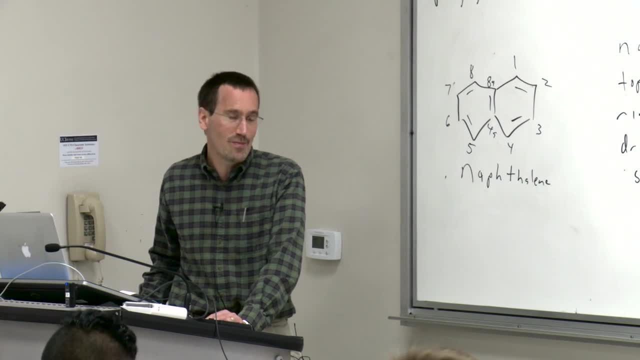 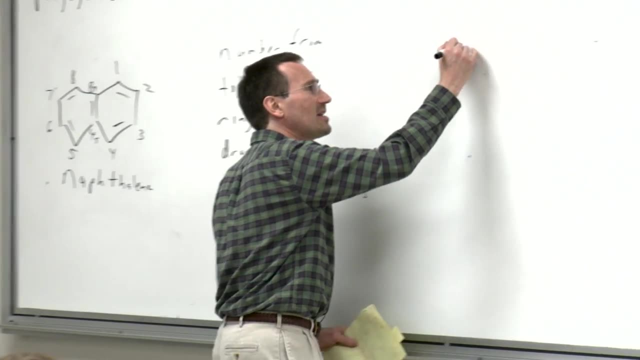 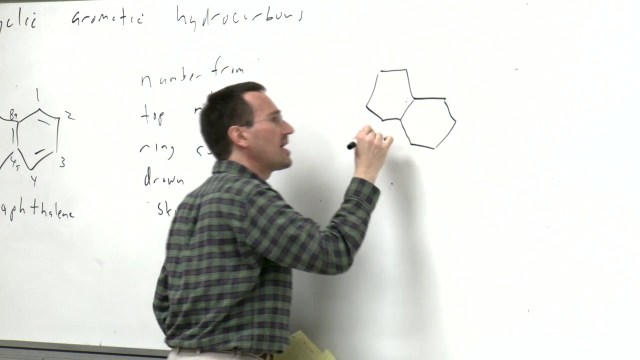 I probably embarrassingly, have a better name memory for molecules name than people's names and my memory for molecules names isn't that great, But there's a number. There are things as an organic chemist that you just see so much again and again that you know. 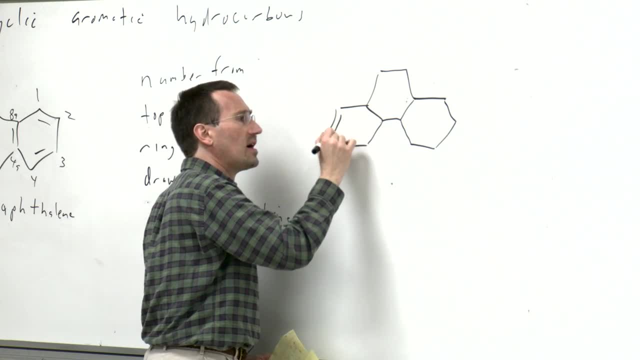 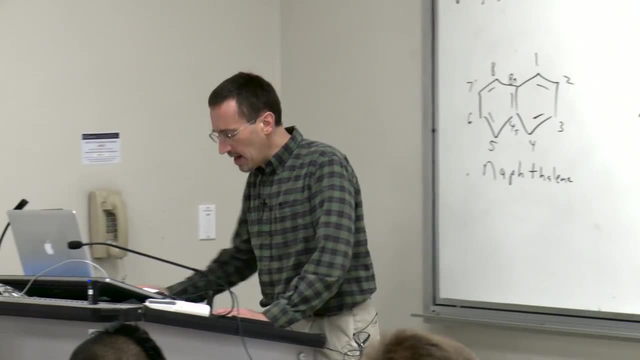 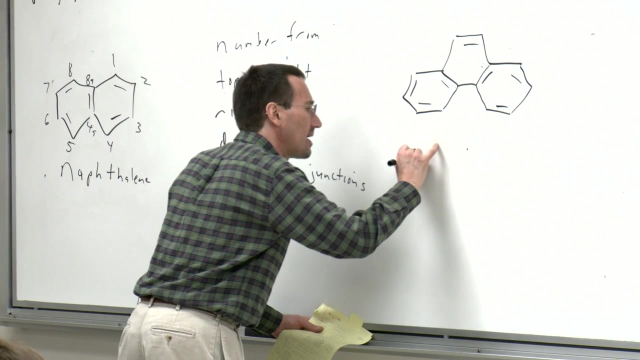 as I said before, they sort of become part of you if you use them or think about them on occasion, And so I'll show you two more polycyclic molecules that I don't know. I mean, I couldn't imagine not being a practicing organic chemist and knowing their names. 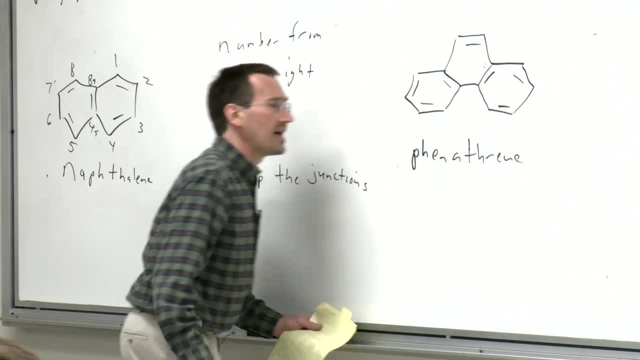 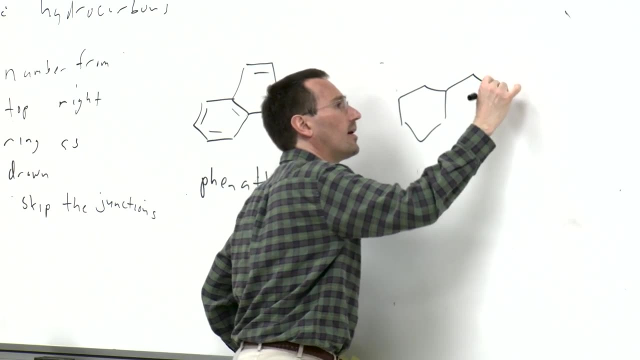 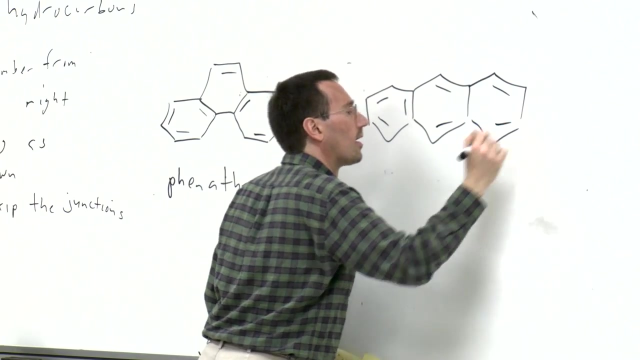 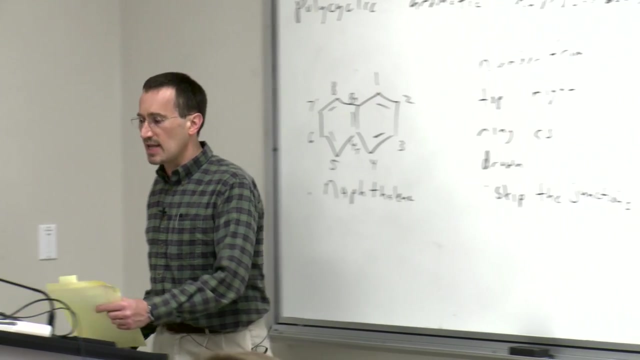 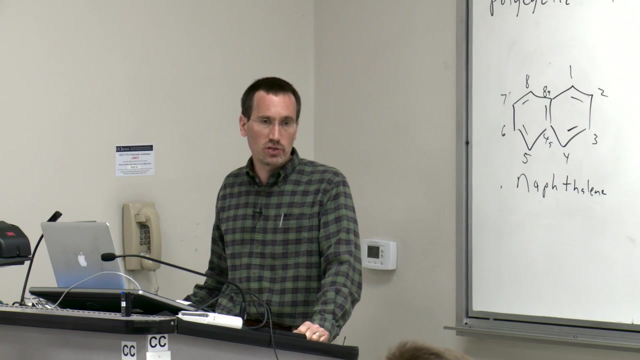 Phenanthrene, Phenanthrene And anthracene, And so all of these molecules are fully unsaturated. In other words, no carbon has- every carbon has, you know- just double bonds to it or at most one hydrogen to it. 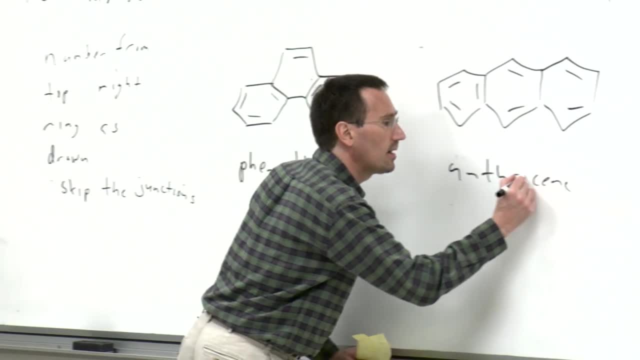 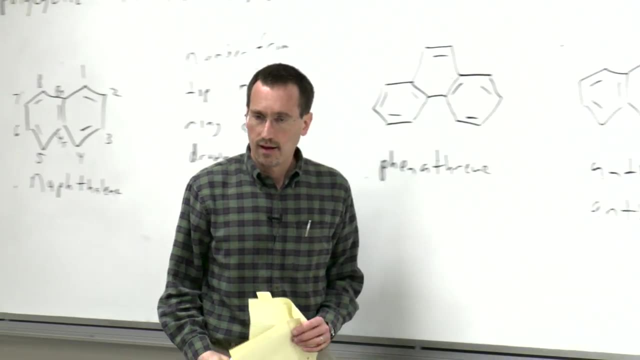 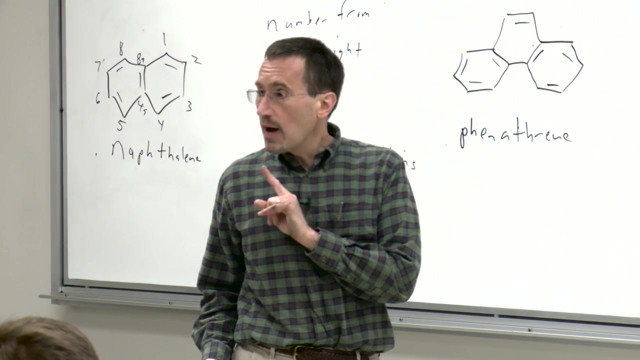 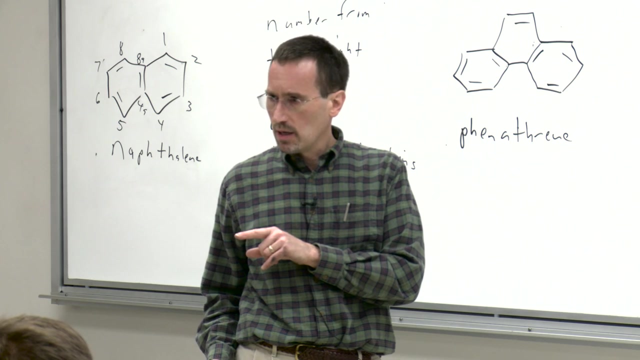 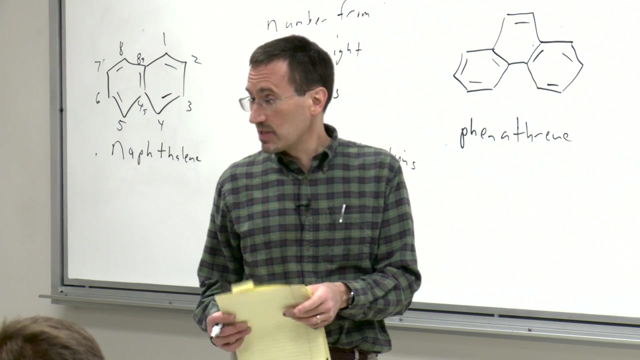 Anyone recognize the name anthracene? Anthrax. To my knowledge, no connection, Maybe I don't know. But another one: Anybody recognize it? Anthracite coal. There's a hard coal that has a name. I think it's called anthracite. 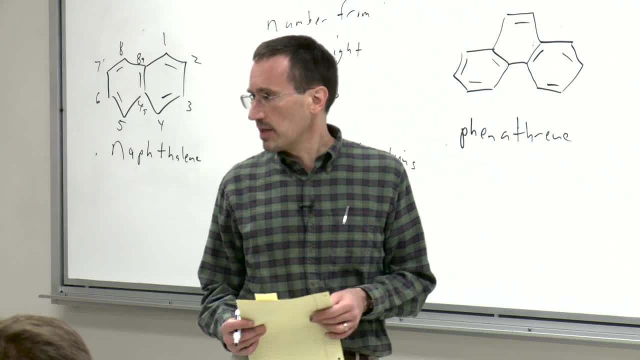 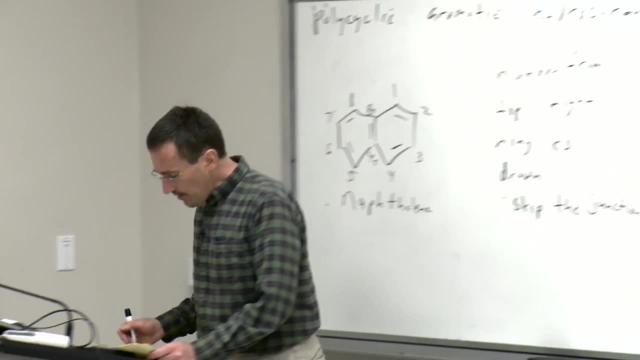 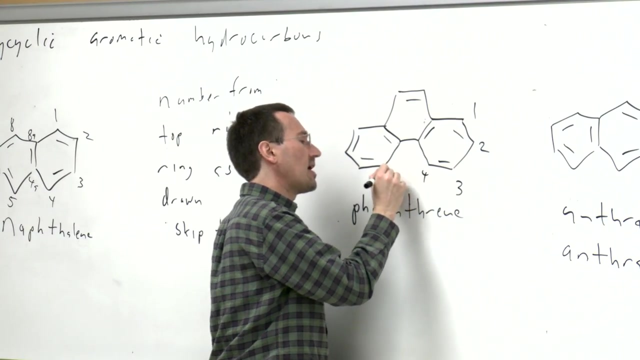 And it basically, you know, given that these are all originally isolated by heating the heck out of coal without air, it's not completely surprising. So keeping the same principles here, I'll just show you here for the numbering of them. This is going to come back in a moment. 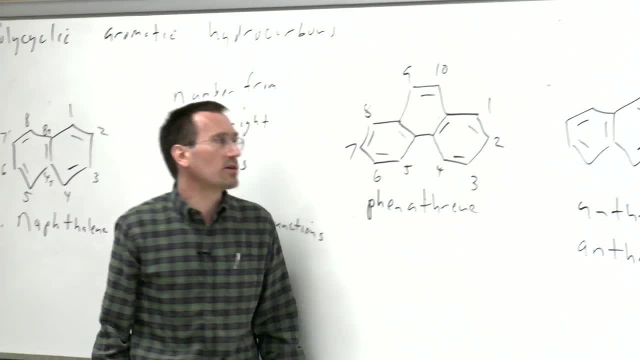 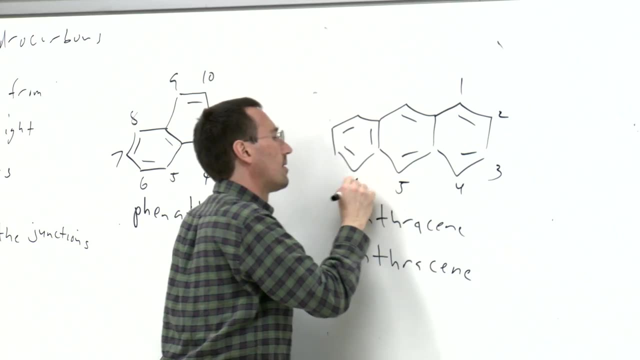 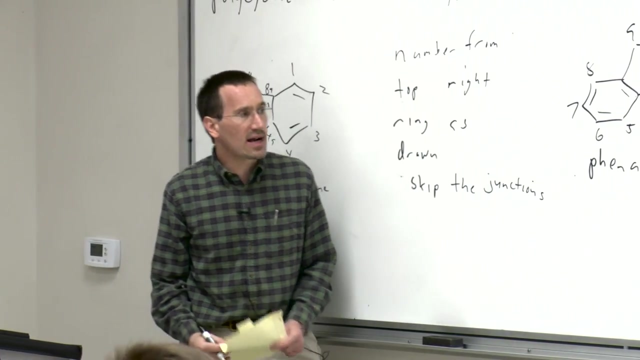 As I said, I want to give an example that relates to this. It relates to cancer. So here's our numbering here. Here's our numbering here. So 5, 10 dihydroxy anthracene would have a hydroxy group at this position. 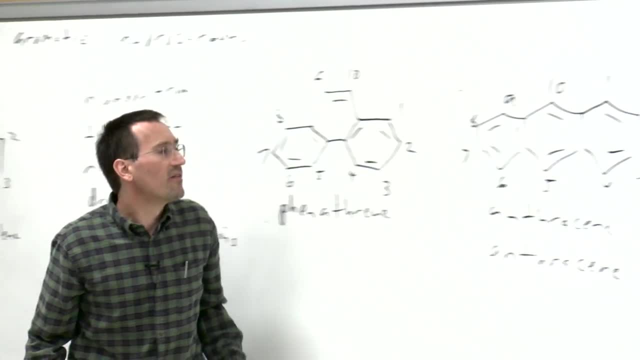 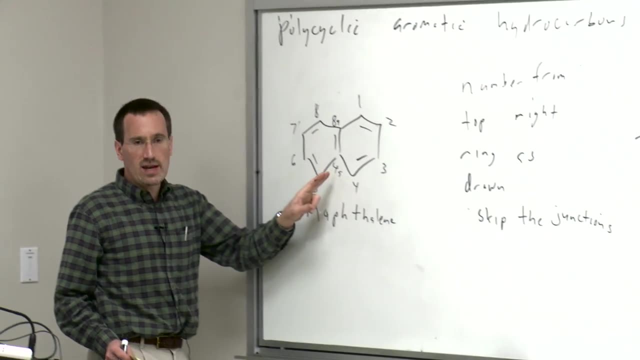 and a hydroxy group at this position, Or 5,, 5, 10 anthracene diol, you could call it. All right. The other thing: we talked a little bit and I sort of threw in as an aside numbering these non-substitutable positions. 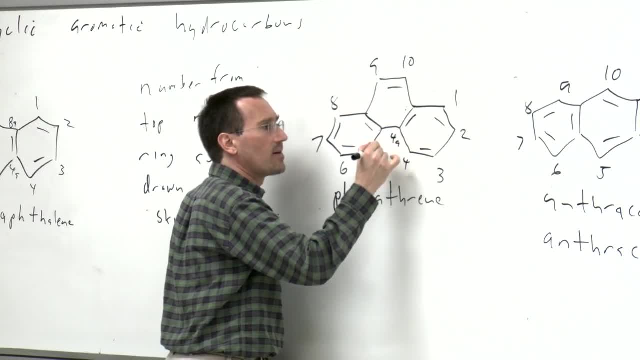 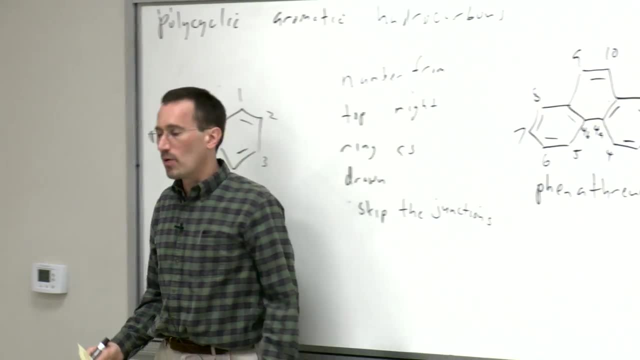 So beyond A you get B. So if you really care about it, this junction here becomes 4A, This one becomes 4B, And then there's, you know, 8A, and so on and so forth. Not super important, but something that's sort of cool and arcane. 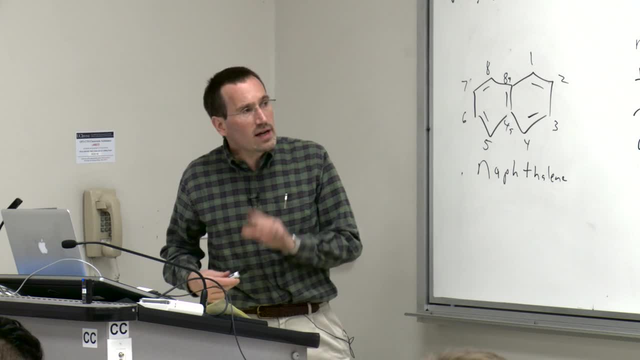 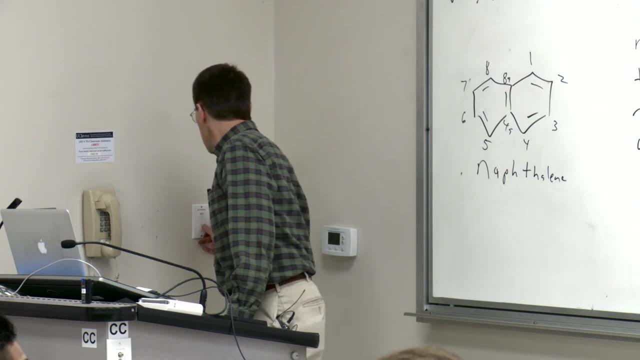 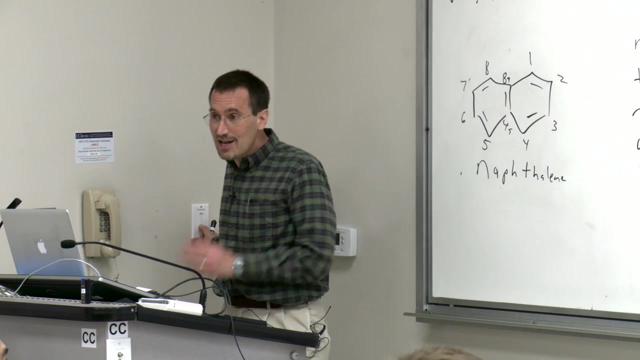 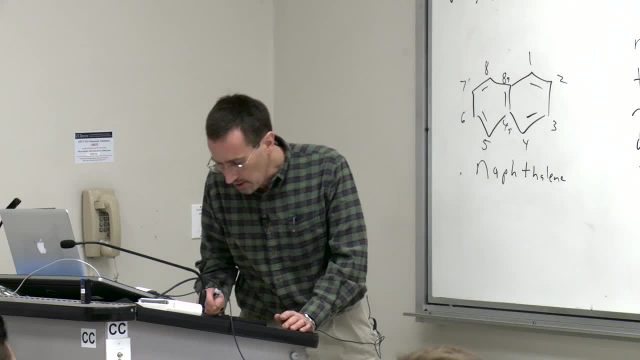 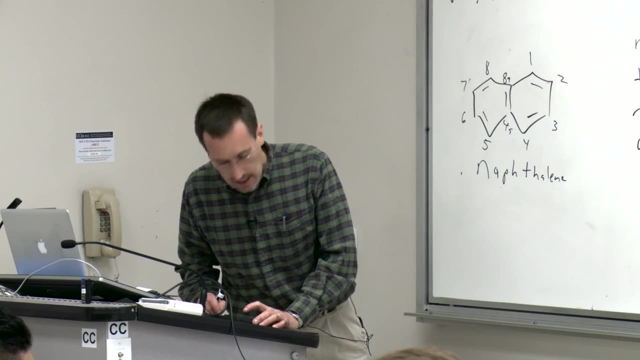 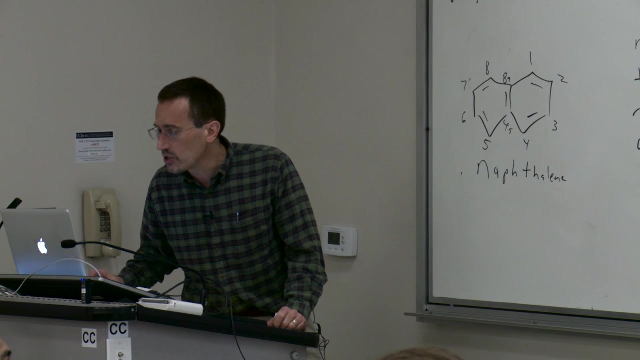 And, as I said, these are going to some of these, not everyone is going to become internal for you, And what I guess I'd also want to add is a little bit of stress is good. I mean, it makes you learn stuff and makes you say, oh, 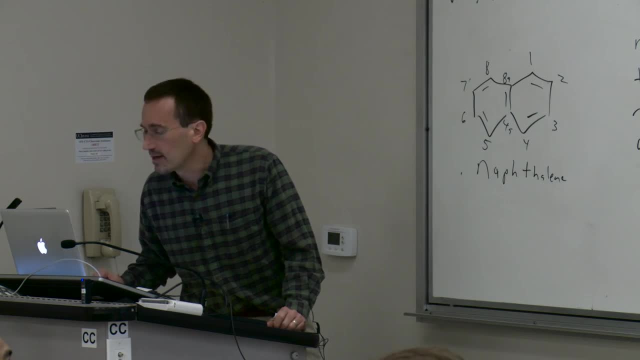 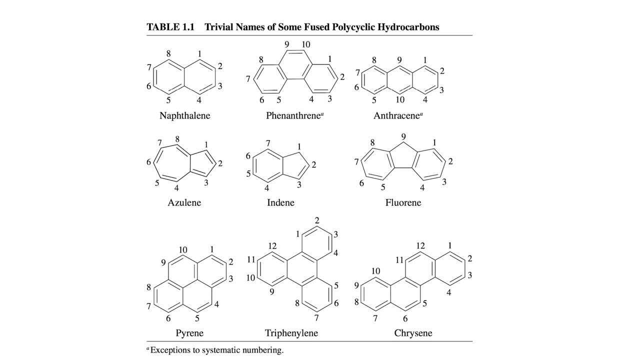 I really have to pay attention. But too much stress is bad because it just means you're going crazy here. So I mean you know right now, work the problems. You're going to read the book, You're going to internalize a lot of it. 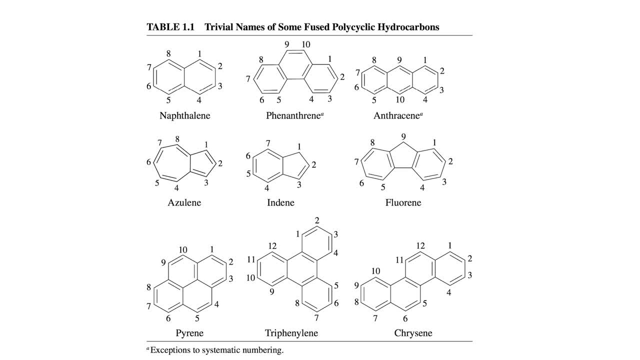 It is my plan, if we end up with anything that has names on it in the exam and I probably will pull something basically to share with you the tables that you printed out on the exam. So you know, here's common names and these are: 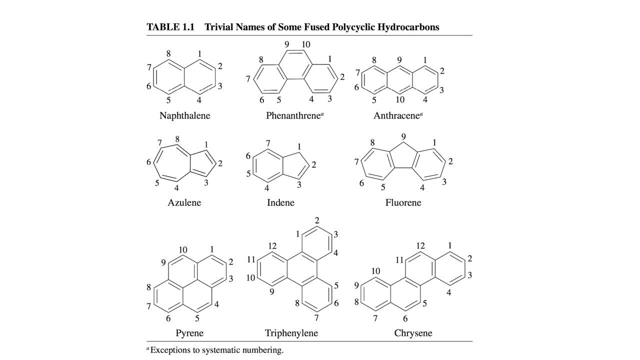 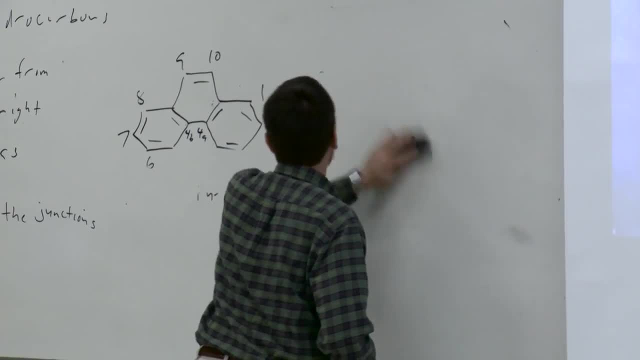 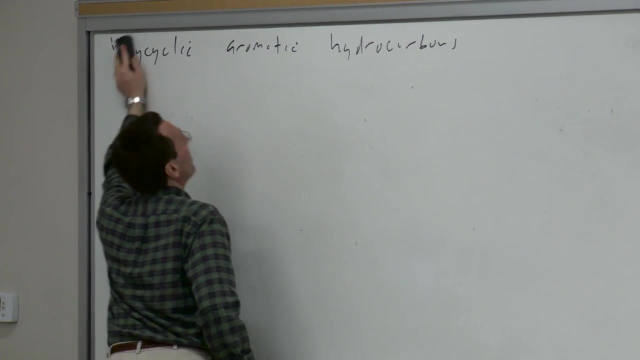 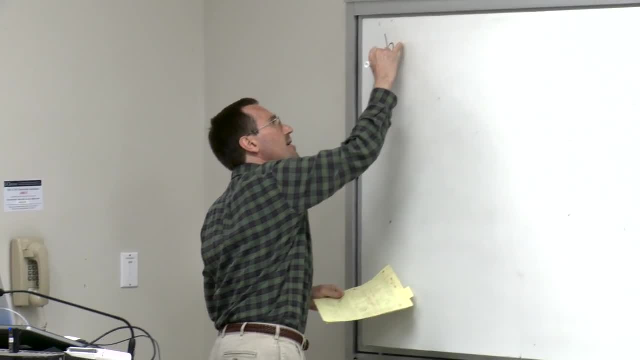 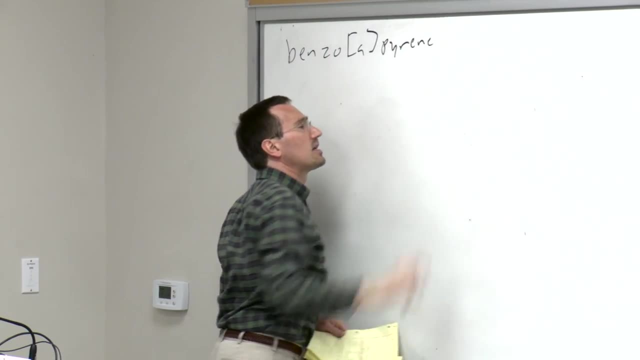 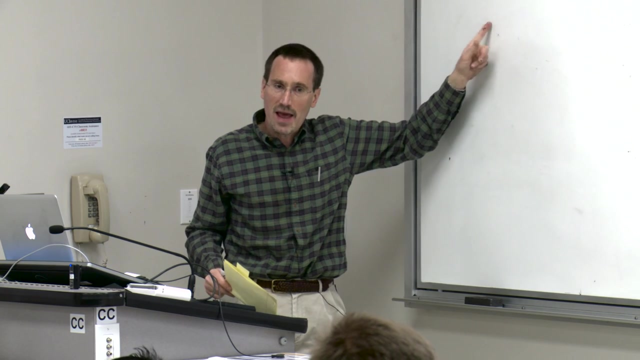 All right. So let's look at that one as an example. benzoapyrine- and this gets us into one more example of nomenclature. All right, benzoapyrine is really bad stuff. You heat the heck out of almost any carbonaceous material. 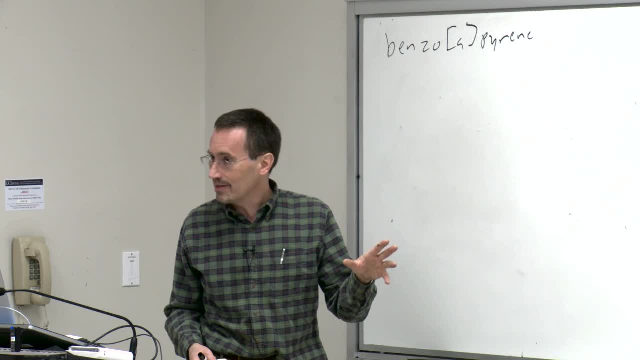 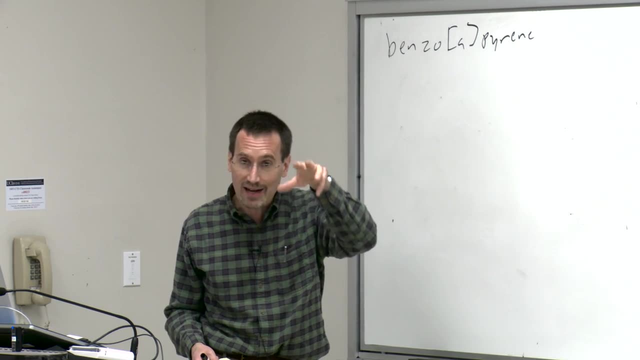 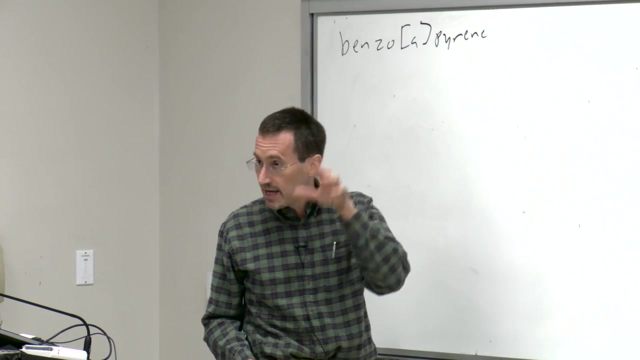 and you get polycyclic aromatic hydrocarbons. That's what's happening in coal. It's been under the ground for hundreds of millions of years with pressure and heat. You're starting with all sorts of carbon molecules from plants and I don't know what dinosaurs, heating and pressing. 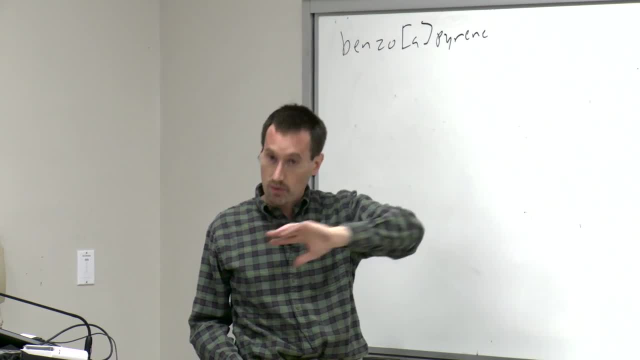 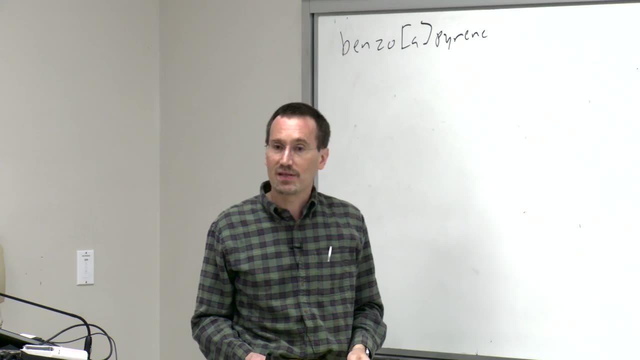 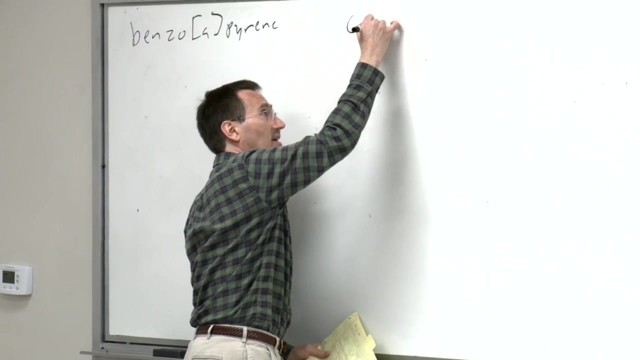 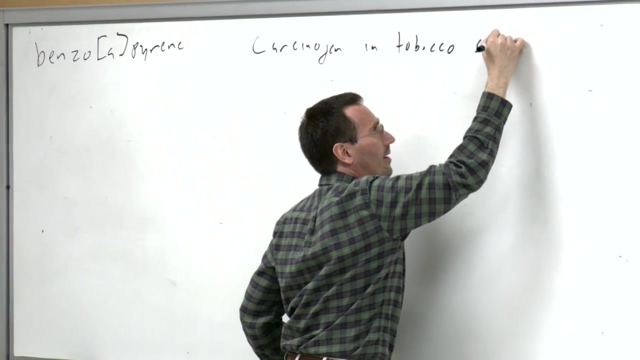 on it for hundreds of millions of years and you get graphite and pieces of graphite smaller and smaller, like anthracene and naphthalene. Okay, benzoapyrine, heat the heck out of here. It's a carcinogen in tobacco smoke and it goes right. 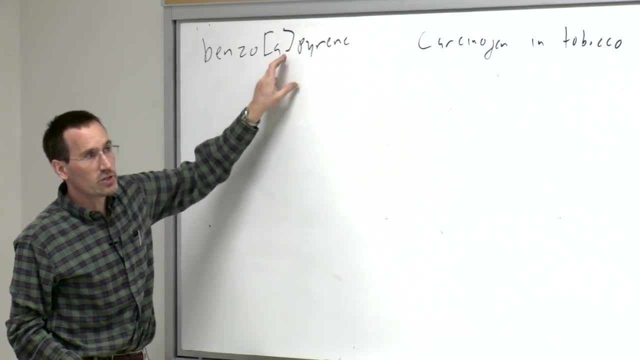 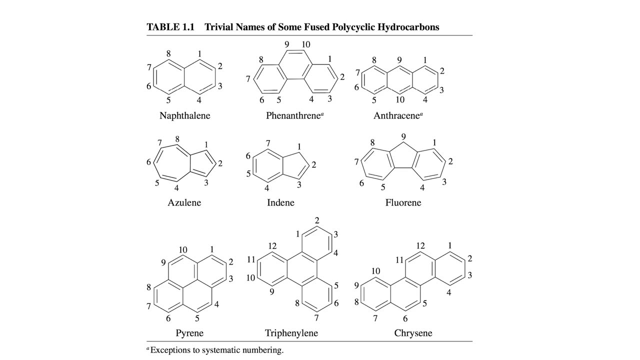 into your lungs. so I want to talk about the nomenclature here. So okay, we've got pyrene. There's a bunch- There's about 35 polycyclic molecules that have common polycyclic aromatics, that have common names. so I want to show you what benzoapyrine is. 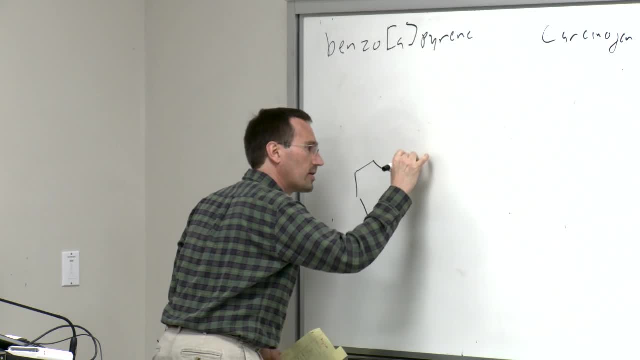 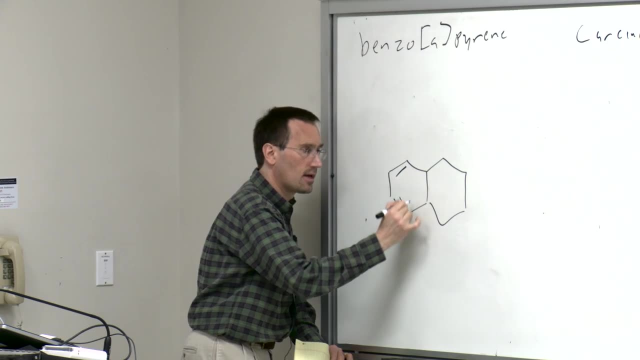 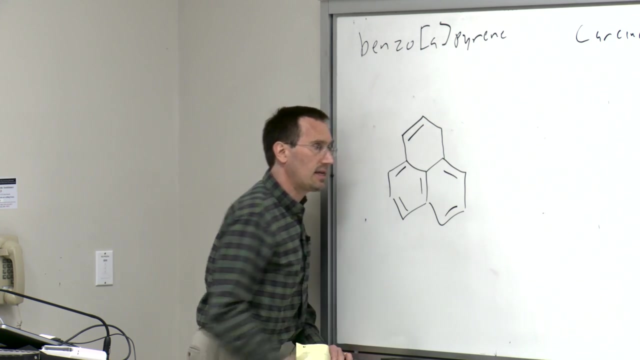 All right, so let's draw a pyrene. You can copy it there or you can copy it from me. I'm going to start and draw naphthalene. I'm going to add a ring to naphthalene. Here's something cool. 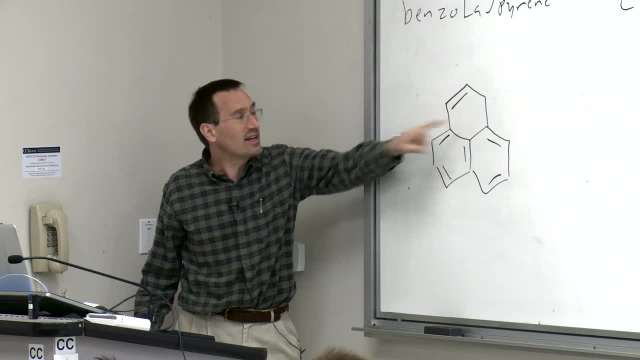 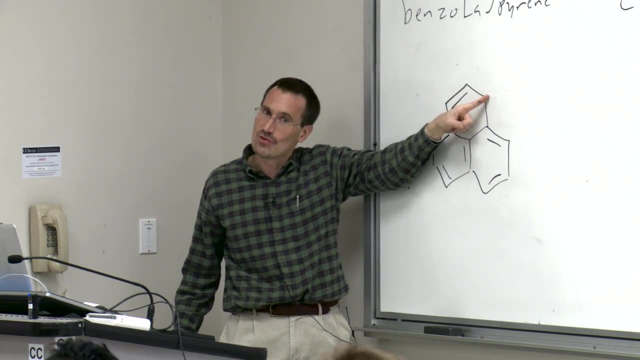 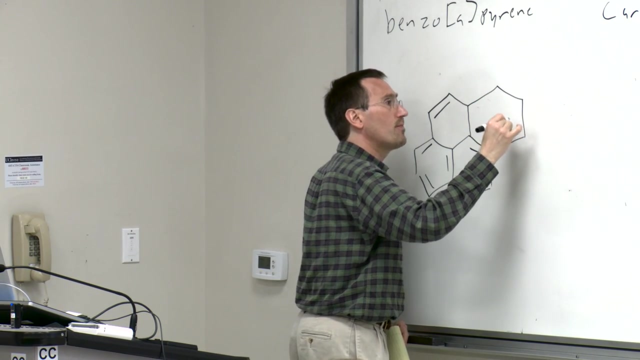 I can't add just one ring to naphthalene and keep a fully unsaturated compound. You notice, I've put in my double bonds And I've run out of room for double bonds here. But you put in one more ring and you're up to a point. 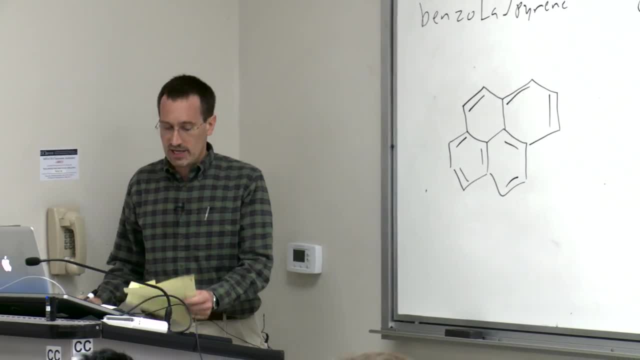 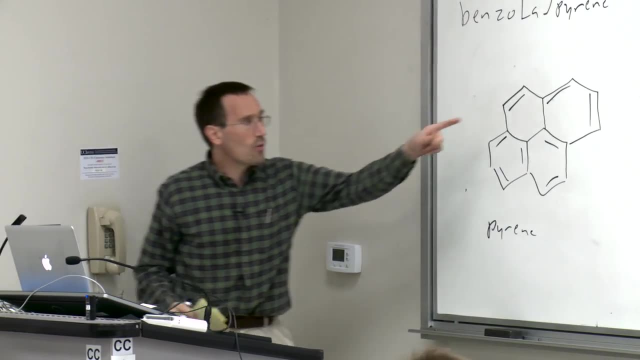 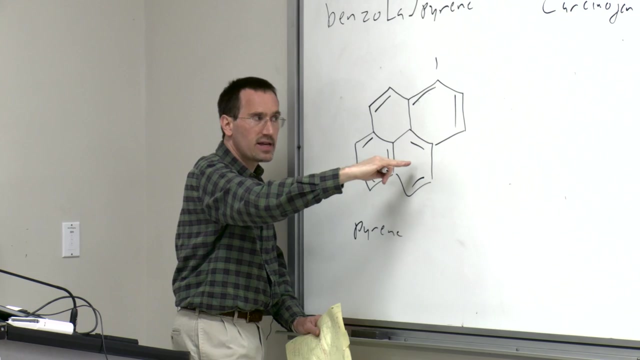 where you can go ahead and have a fully unsaturated compound. So this is pyrene. We're going to number around as drawn and you see that you have it here. So, basically, as drawn, we've drawn horizontal rings as many as possible. 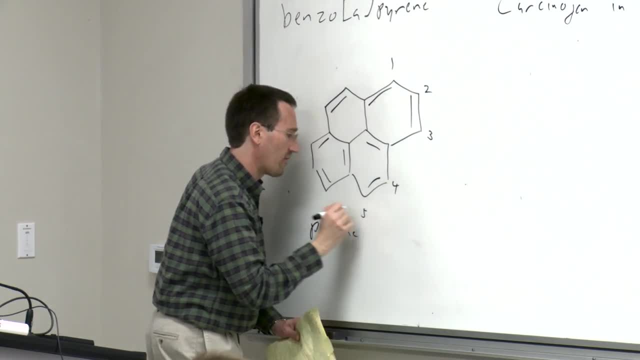 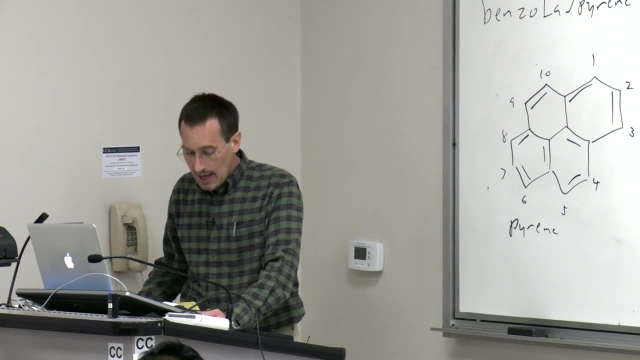 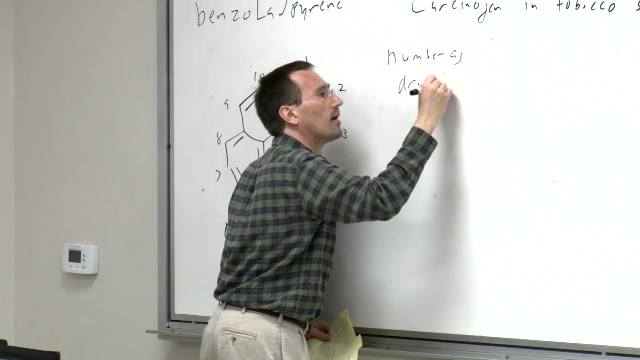 We'll start in the upper right: 1,, 2,, 3,, 4,, 5,, 6,, 7,, 8,, 9, 10.. It's right there on your screen as well Now. so I'll say: number is drawn from the upper right. 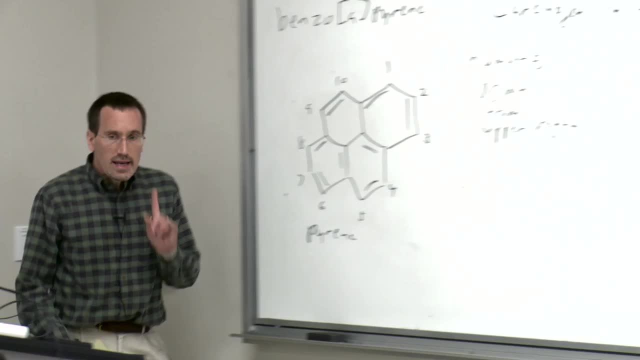 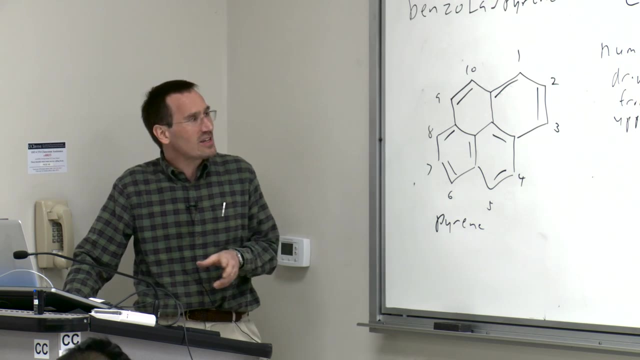 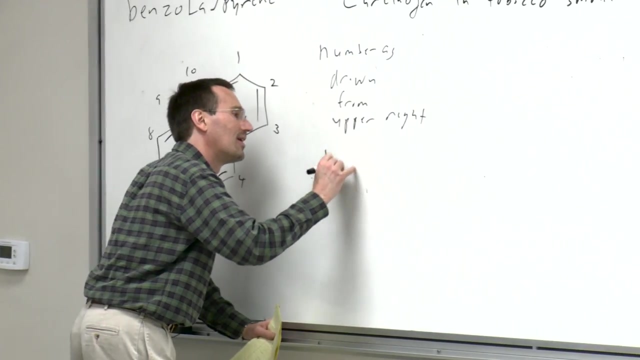 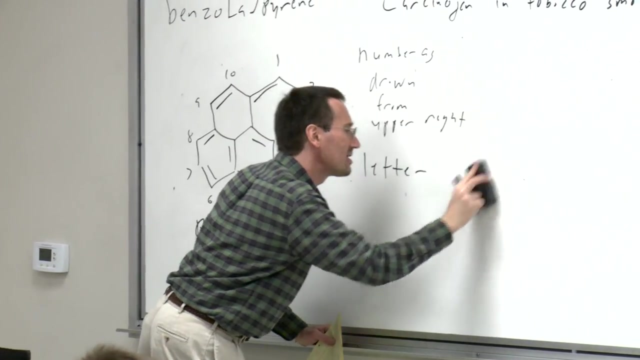 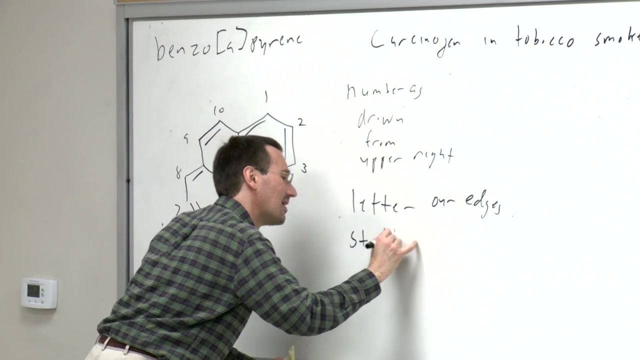 Now the next piece of arcane business- in nomenclature It's all sort of cool And freaky at the same time- is we're going to letter starting with 1 to 2.. I'll say: letter our edges, starting with 1 to 2 and doing all. 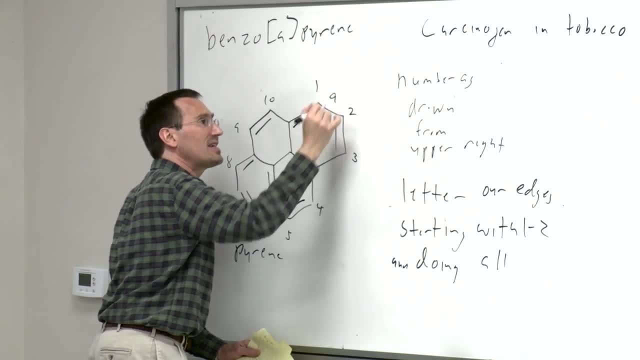 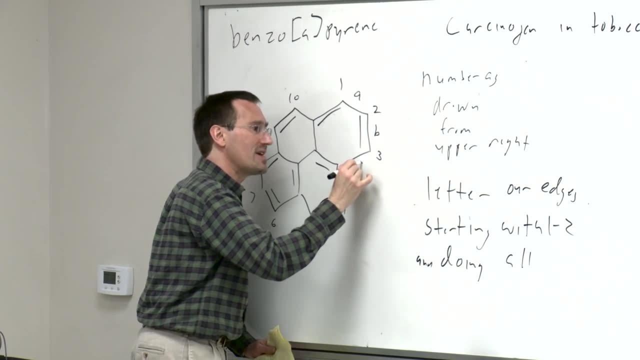 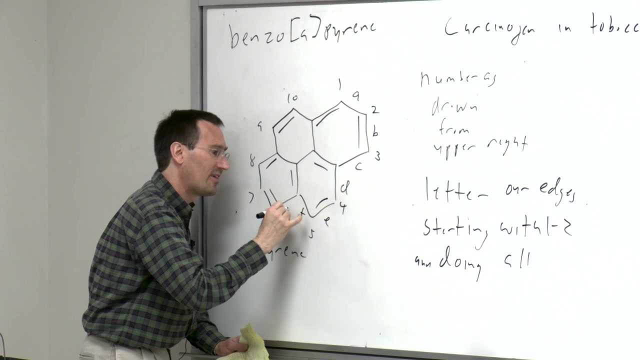 So, in other words, we'll letter this edge A. That's good, because I said we have benzo A pyrene. This edge B, This edge C. we're going to continue around right to position 3A, D, E, F, G, H, I, J, K, L, M, N. 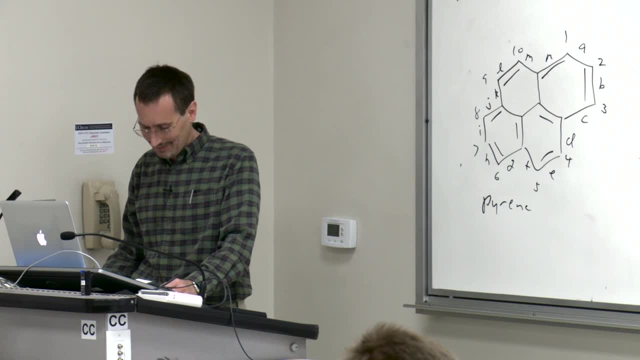 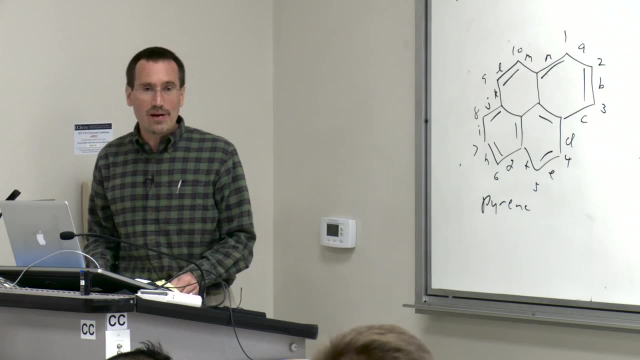 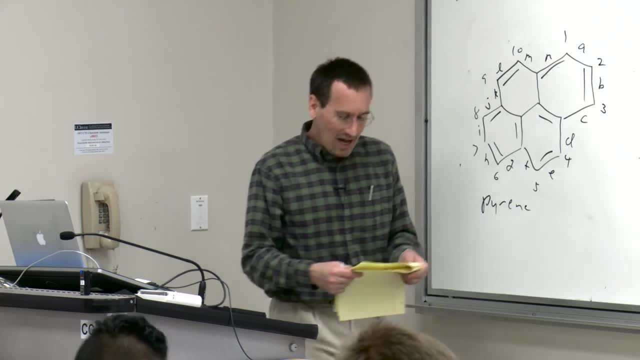 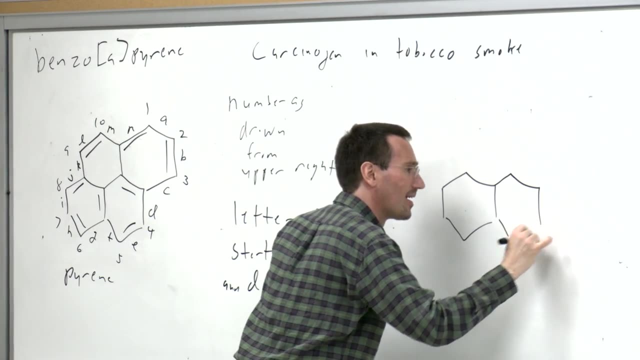 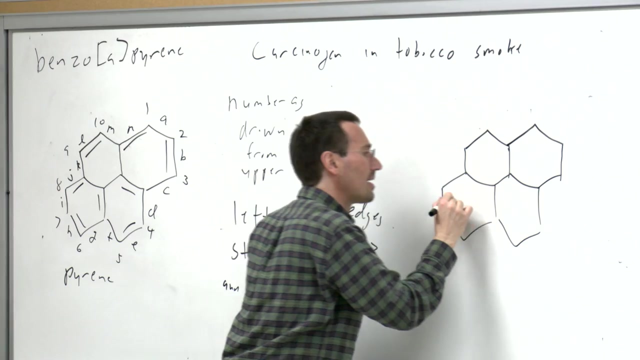 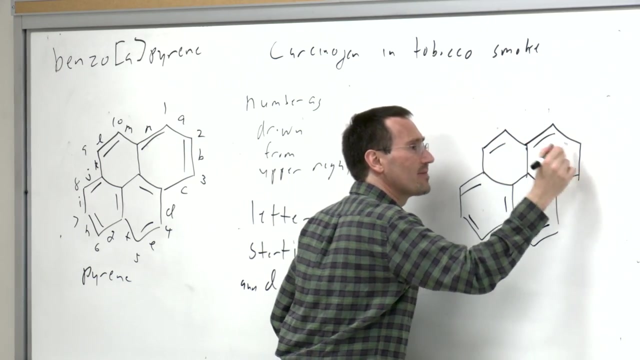 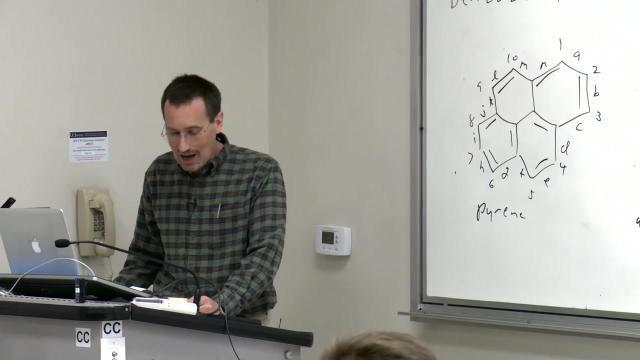 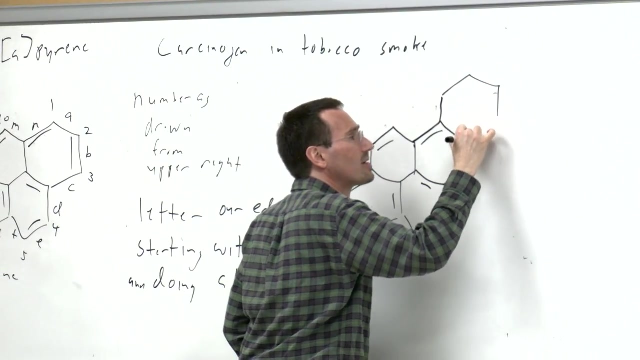 Then we're just going to fuse another benzene onto the A ring. So I'm going to redraw a pyrene, And part of this is an exercise in us just spending a few moments to see the anatomy. here We're going to add a benzene ring onto the A ring or onto the A edge. 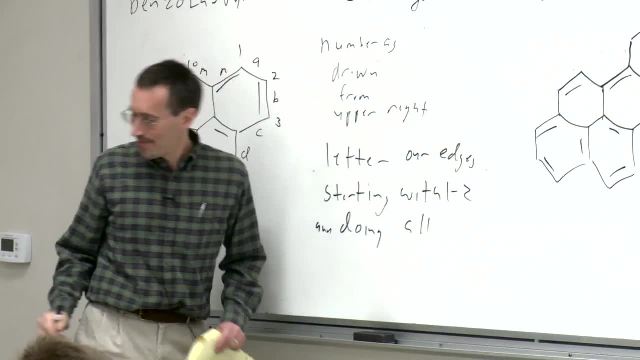 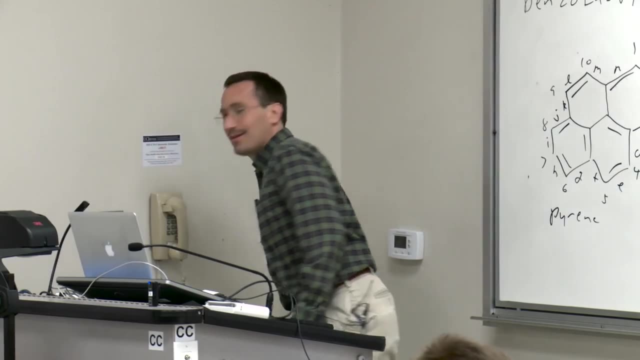 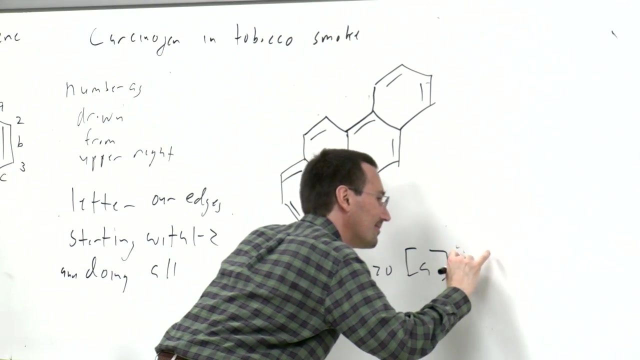 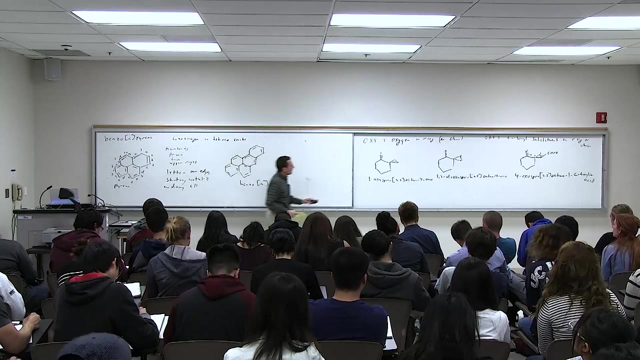 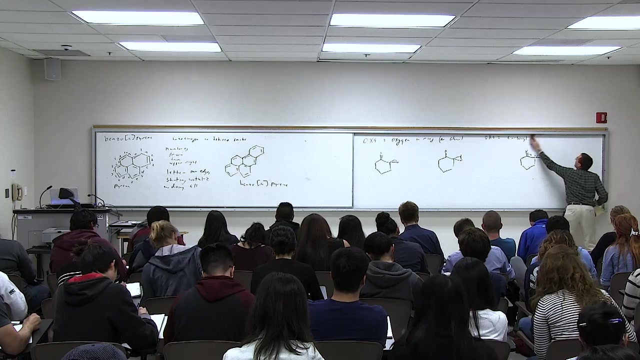 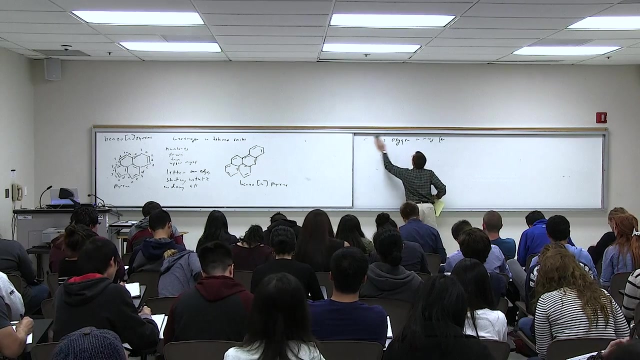 And so that's benzo A pyrene. Let's see. Give that a go see if what happens here find out. I did that. It's got a little bit offreezel on it. actionable wave in common, All right. 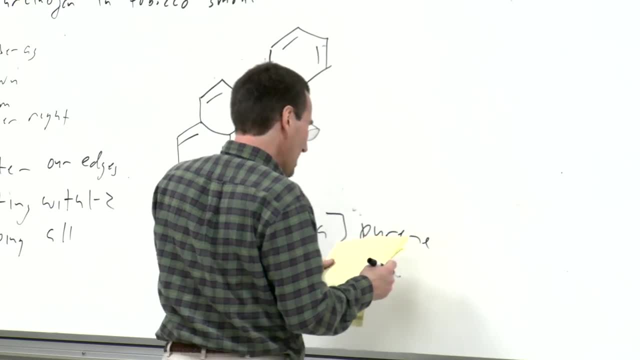 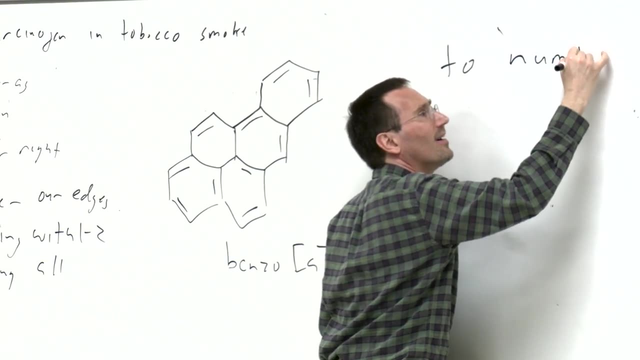 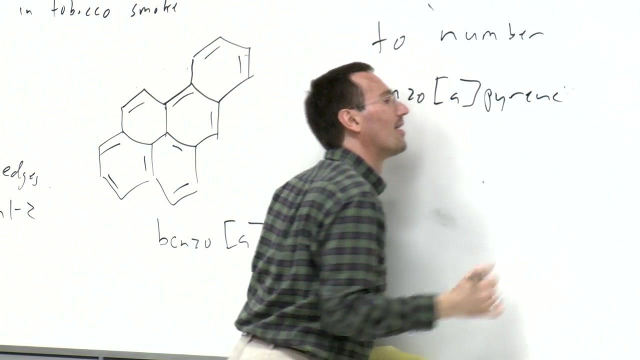 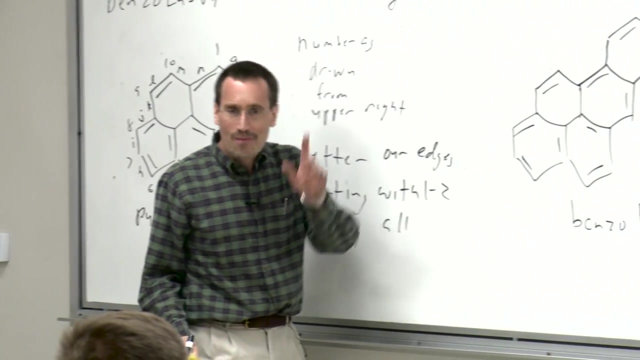 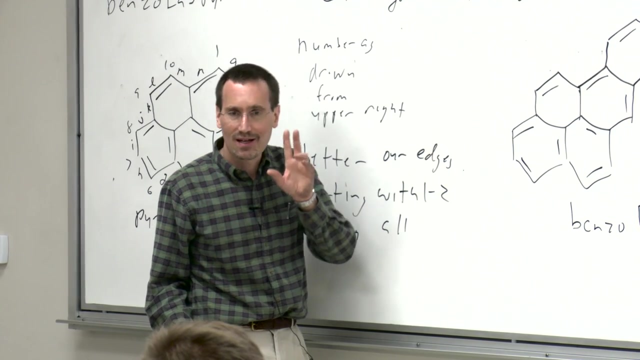 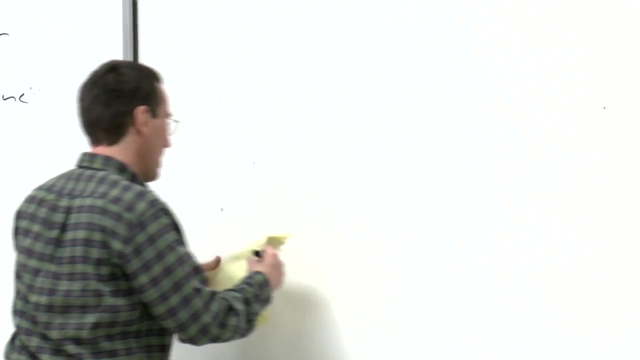 So now what's going on? Oh, we go from one to another. Okay, so then for numbering. now you reorient, And it's this principle of maximum number of fused rings, horizontal, And then we start numbering from the upper right-hand ring. 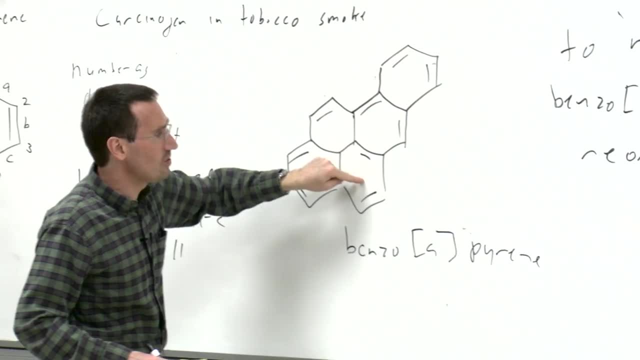 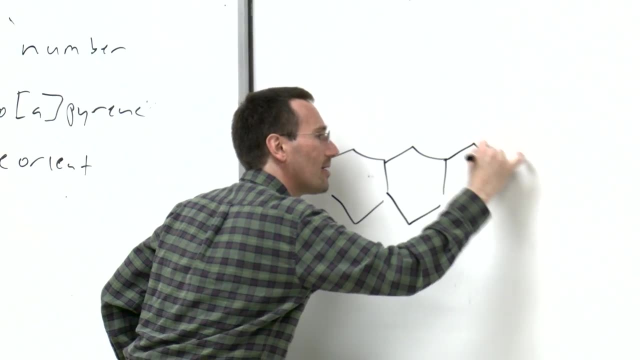 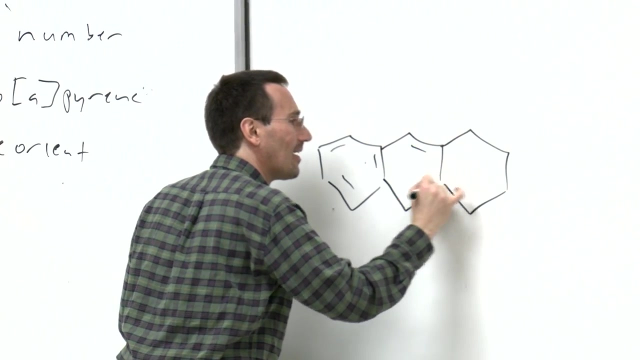 So maximum number of rings: 1,, 2, 3.. So, just like anthracene, we're going to do 1,, 2, 3.. I'm coming here to an even nastier carcinogen, And then we're going to take the remaining two rings. 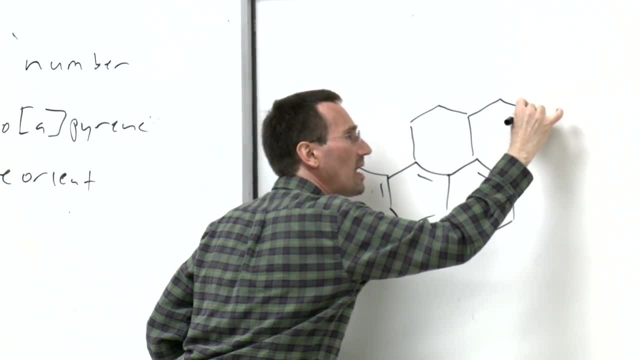 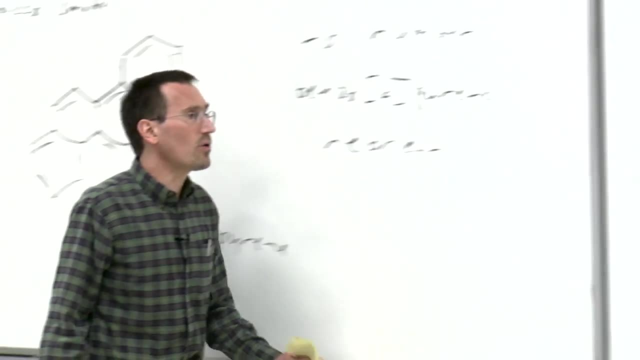 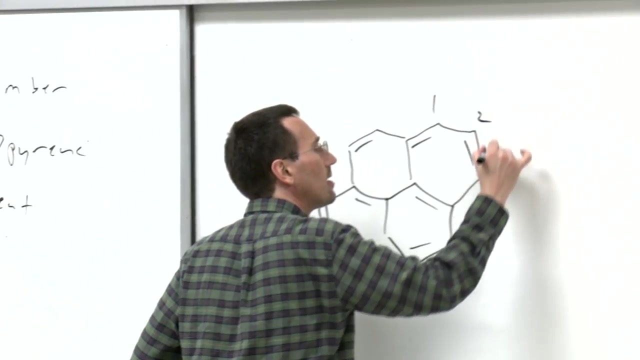 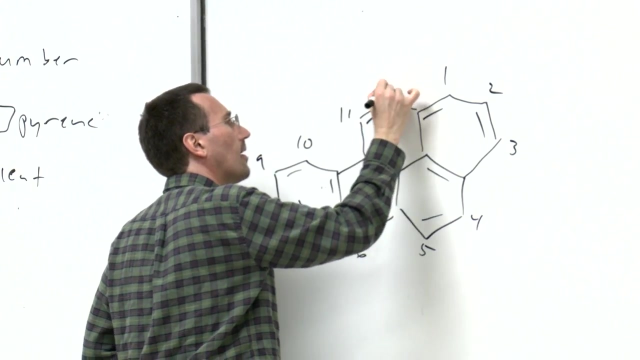 and stick them up in the upper right-hand corner. So all I've done is flip and rotate our molecule around. So that's how we orient it for numbering. And then we number from the upper right-hand ring. And that's how you number your benzo, A pyrine. 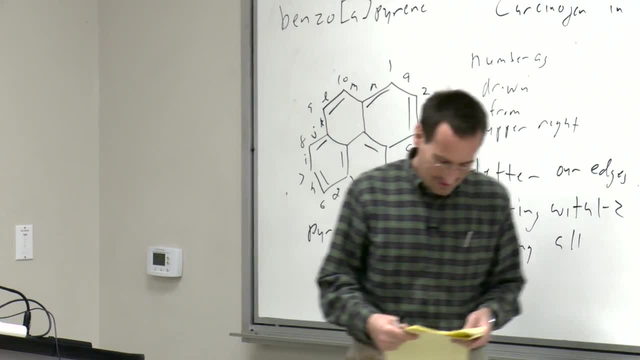 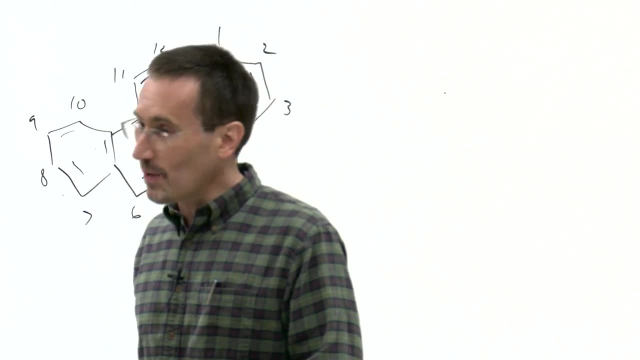 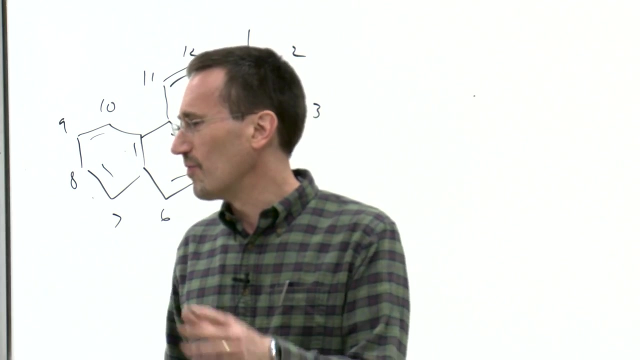 All right well, benzo A pyrine, as I said, is what you breathe in when you're one of the many carcinogens. when you breathe in hamburger smoke, I think it also tobacco smoke. I think it also forms in burned meats. 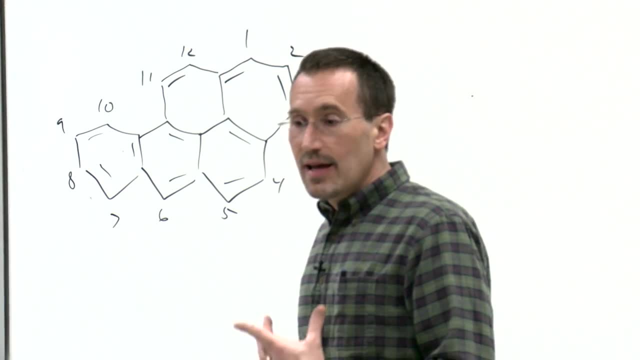 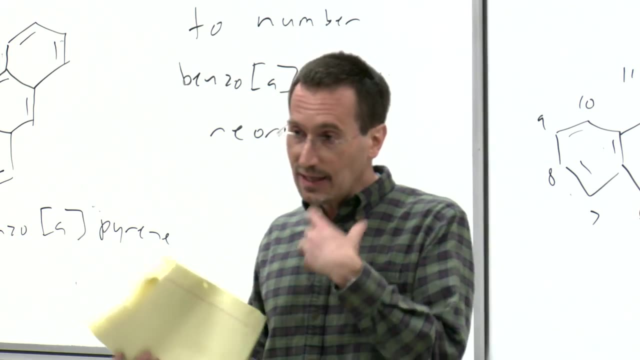 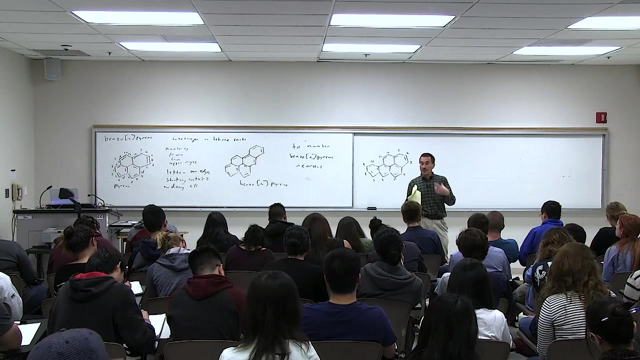 But your lungs are really vulnerable to cancer. Now your body takes big greasy, greasy objects, big greasy molecules, And it can't process them, It can't carry them, It can't excrete them when they are so greasy. 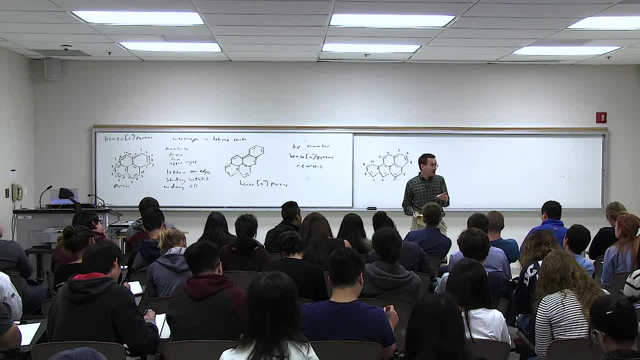 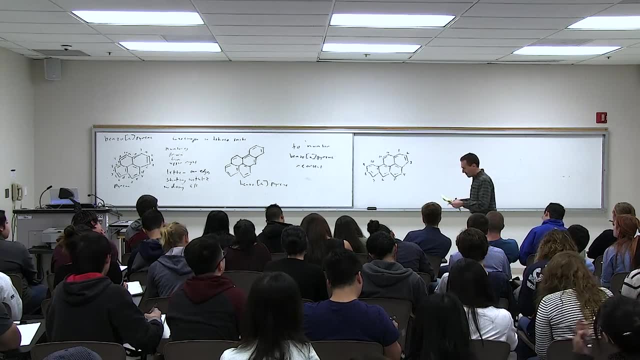 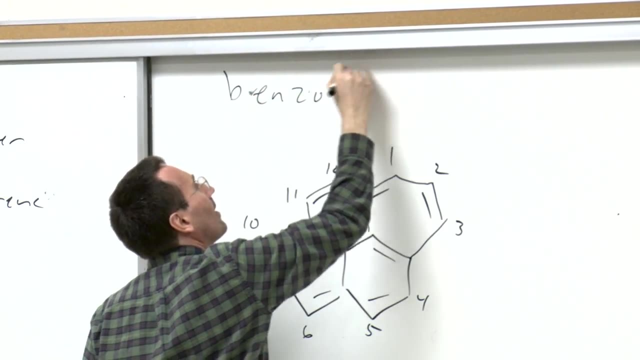 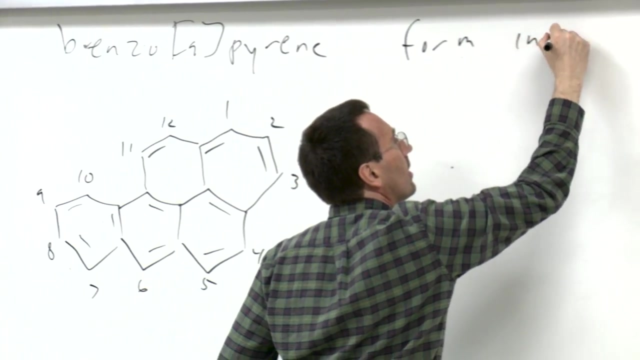 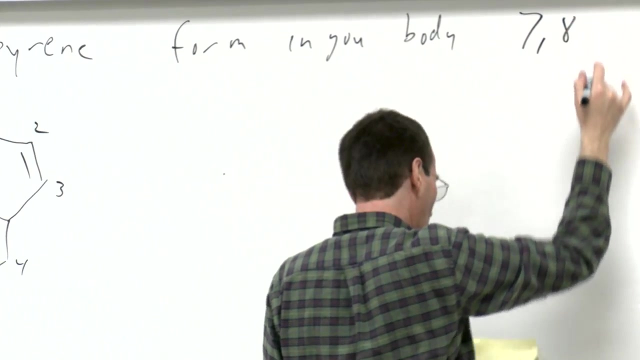 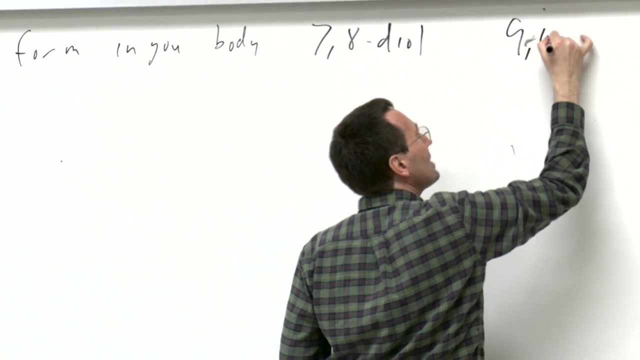 So your body does what it does to process big greasy molecules. It oxidizes them with an enzyme called cytochrome P450.. And so benzo A pyrine, It's an enzyme that forms in your body, the 7,8-diol-9,10-epoxide. 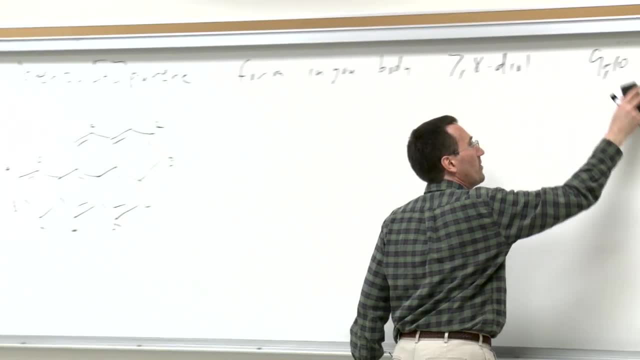 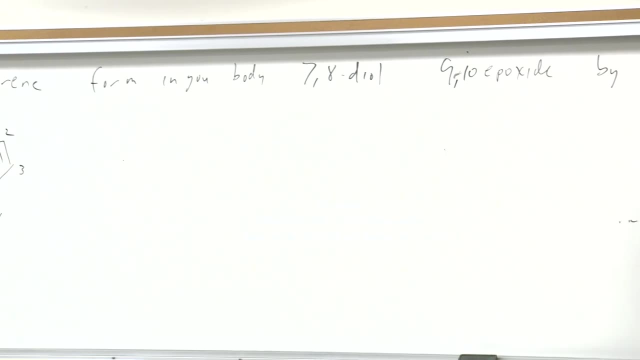 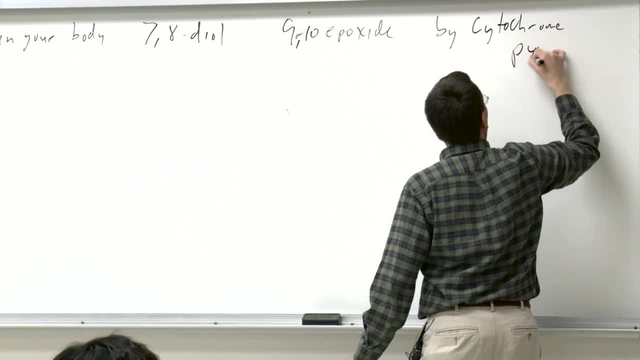 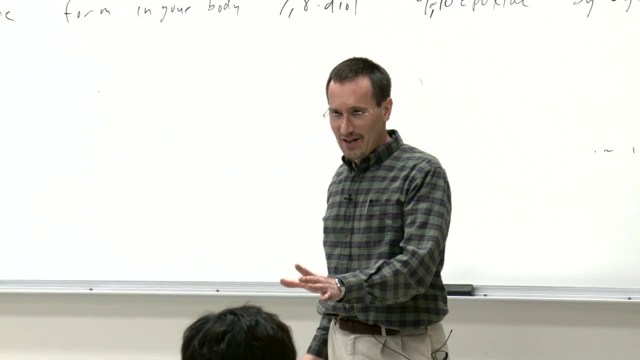 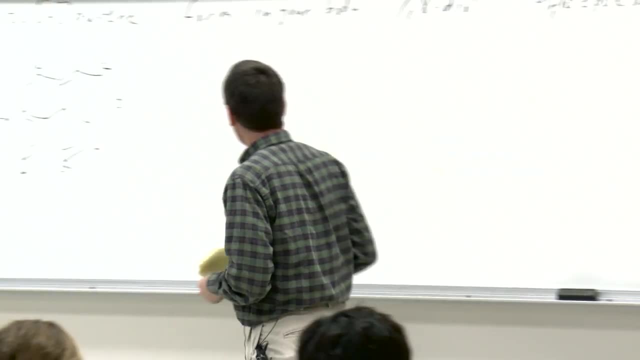 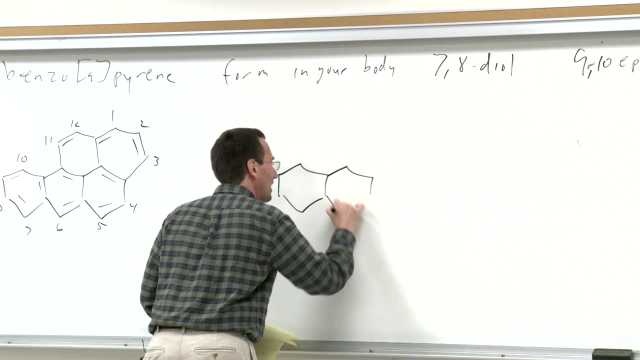 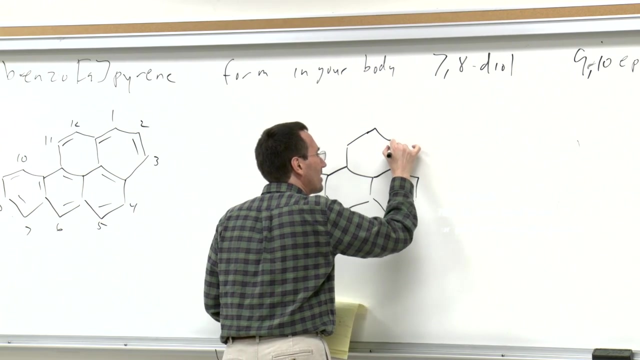 It oxidizes them with a heme-containing enzyme, And so we're going to draw that molecule kill now. and so now we know the secret of nomenclature and I actually, until I read this book, never quite knew how one got there, and it's sort of like, oh cool, now I know this little arcane. 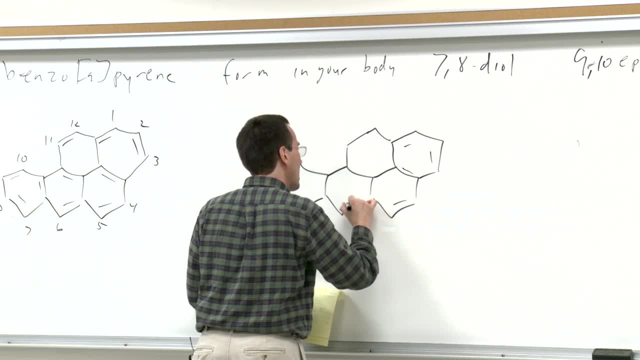 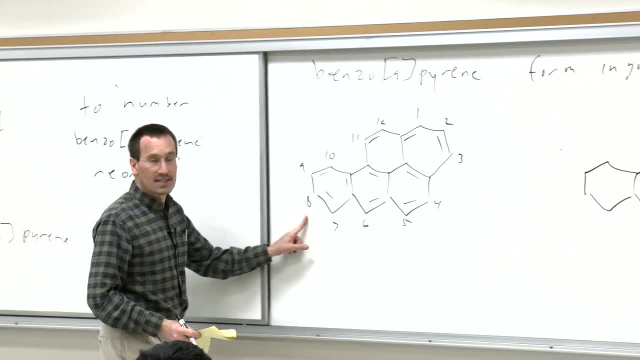 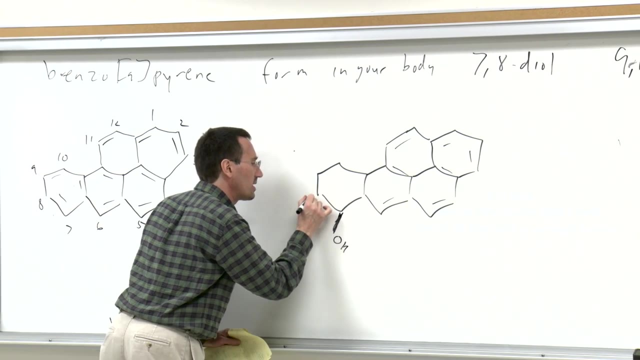 piece of knowledge, and so we're just going to number around, as we have done, and we'll come to this ring which we said seven, eight die. all I'm going to draw. there are a couple of diastereomers that conform actually to two enantiomers. I'm just going to draw one of them. I'm specifically not. 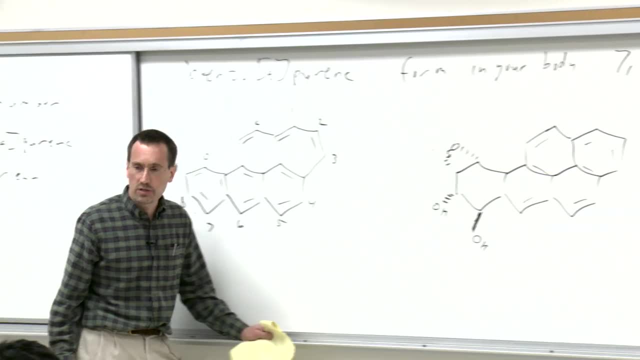 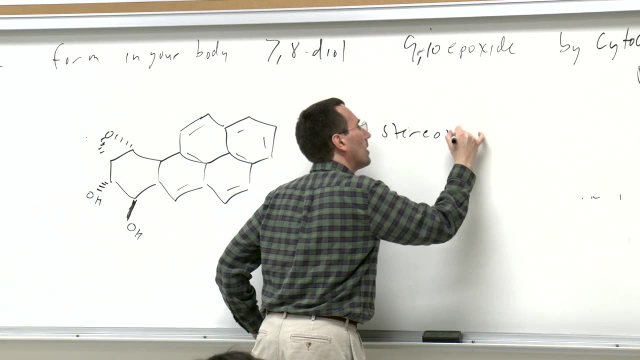 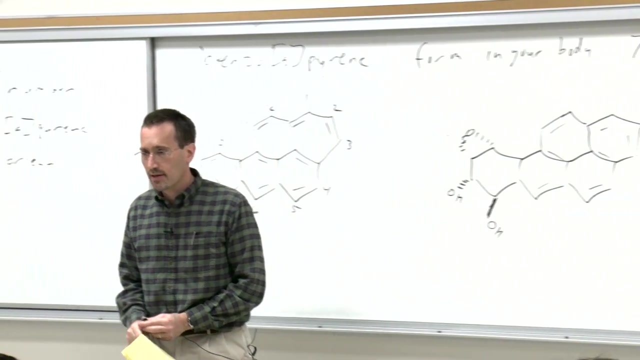 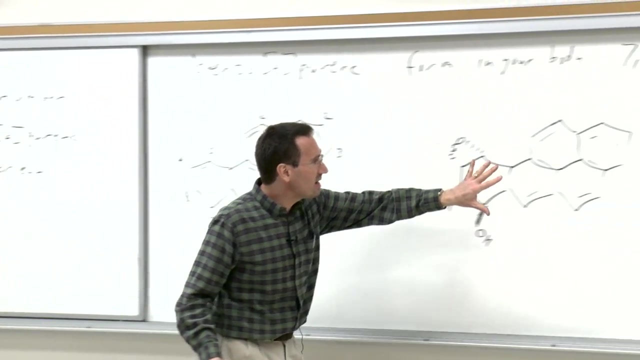 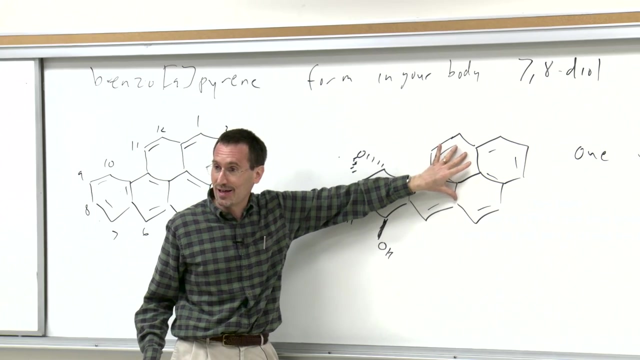 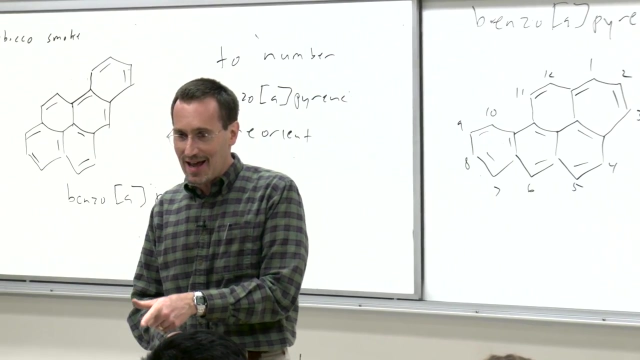 specifying the stereo chemistry in my nomenclature. so I will just say this is one stereo isomer and this is what gives you cancer. anybody have any idea what this big flat hydrophobic region, greasy region, looks like- something related to cancer? where does cancer start? DNA, yeah it. 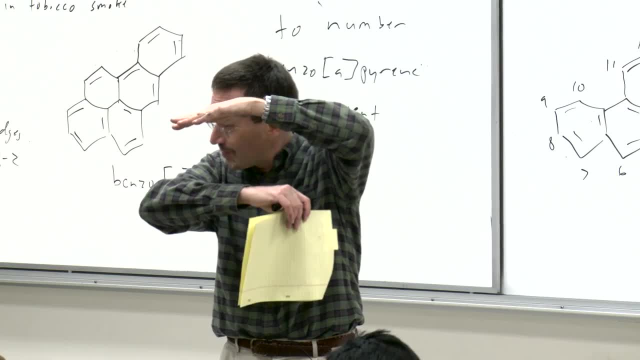 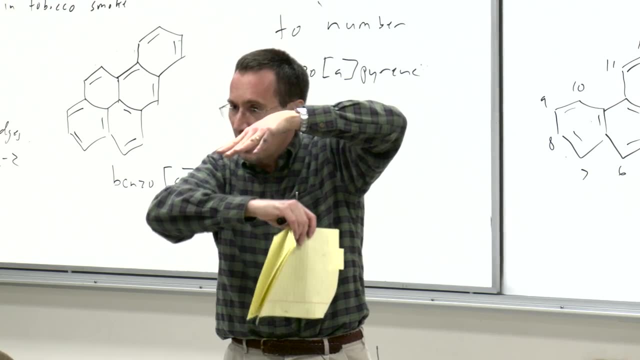 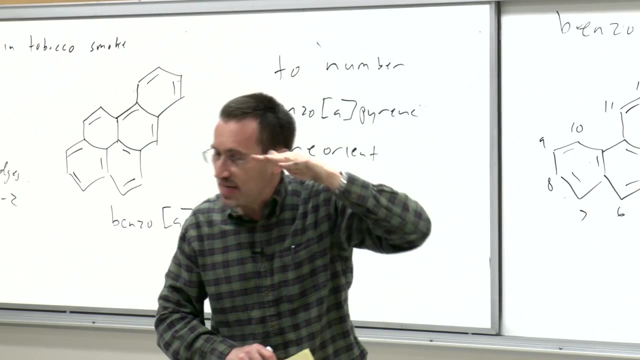 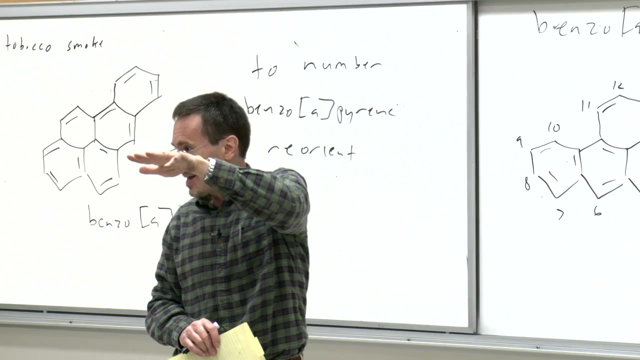 intercalates, so you still have your double helix. big, flat, greasy molecules stick themselves in between the bases. who's had a biochem lab or anyone work with a city and bromide? okay, a city and bromide is a big, fat fluorescent dye molecule that goes into your DNA, but your body has just put a warhead on this big. 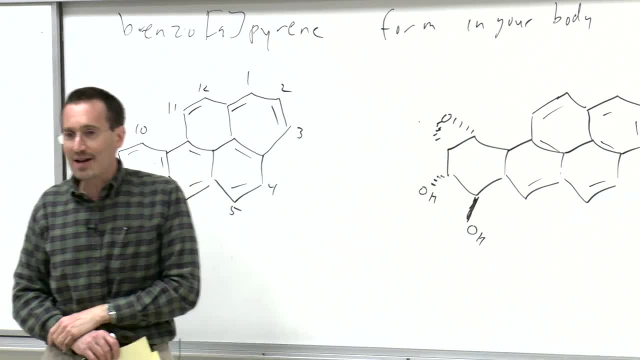 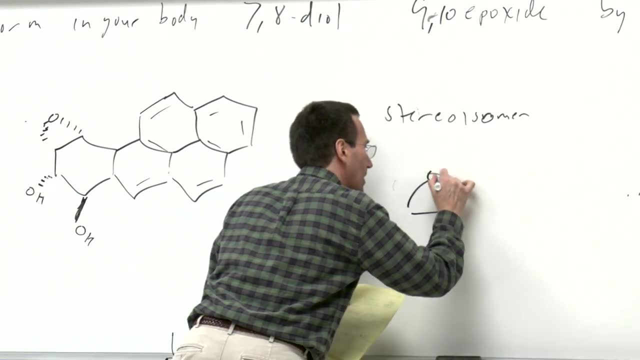 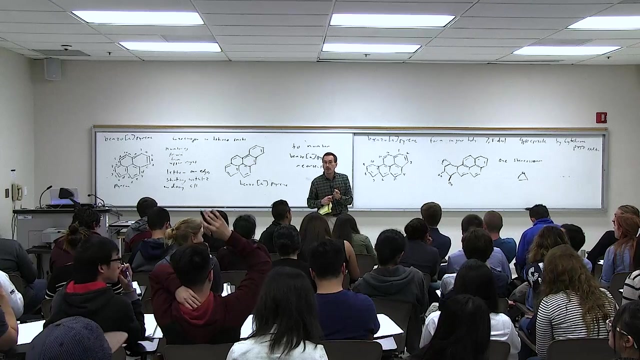 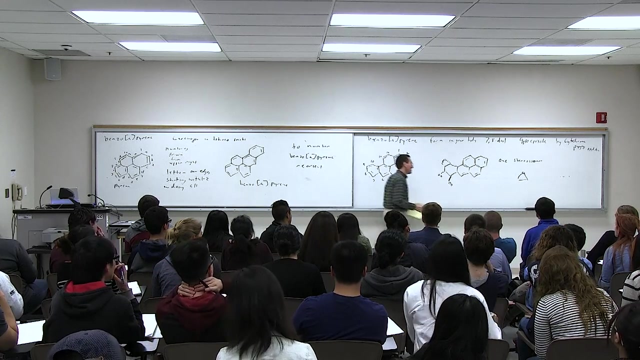 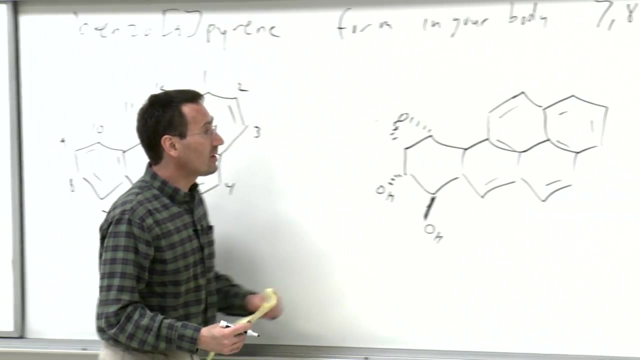 flat molecule. what do you think that epoxide ring? think back to all the way to sophomore organic chemistry, to that molecule, to oxy rain. you used it for something in sophomore organic chemistry- exactly, it's a DNA alkyl. later, so a nucleophile like nitrogen react here are any nucleophile like nitrogen, I believe its reacting. 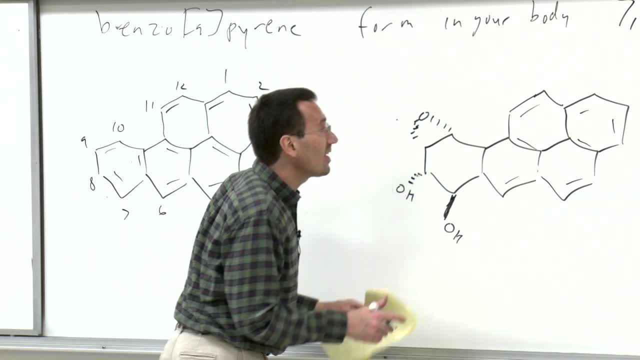 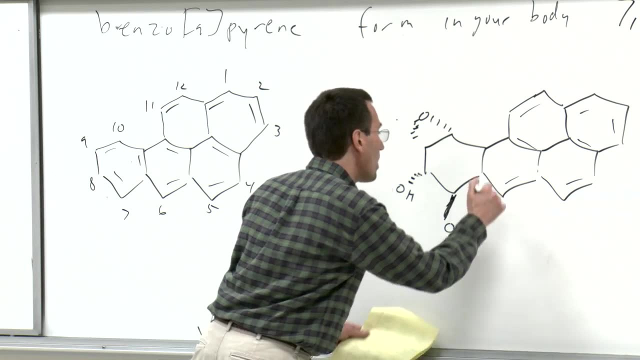 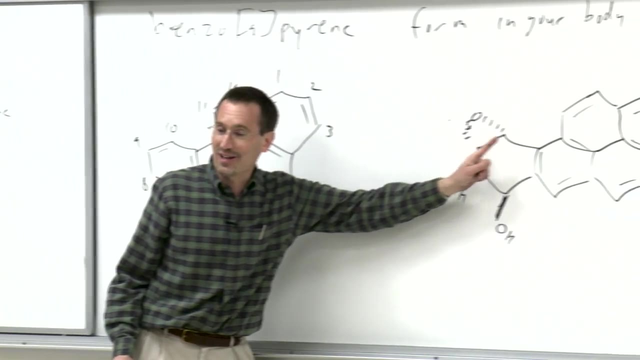 right over here. and what if I hold on? I have managed. what have I managed to do? oh, one more double bond. there we go. so benzylic position, and so it is particularly reactive. You can find x-ray crystallographic structures. 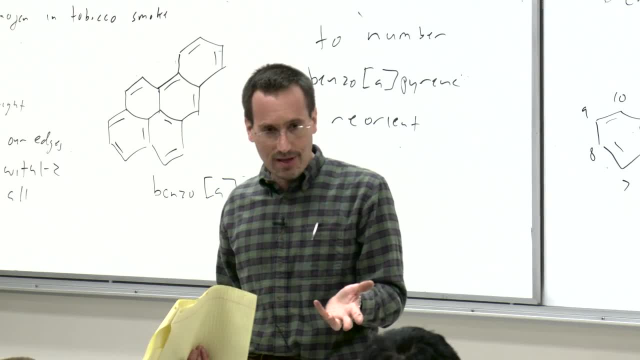 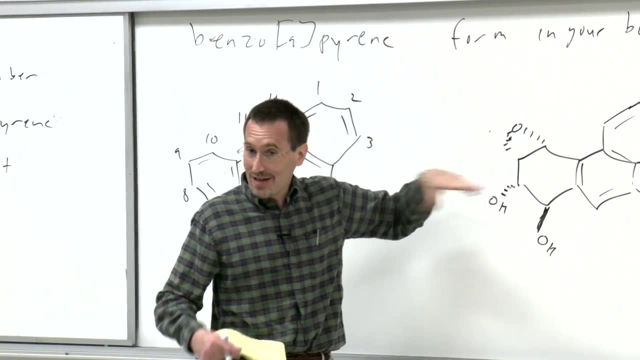 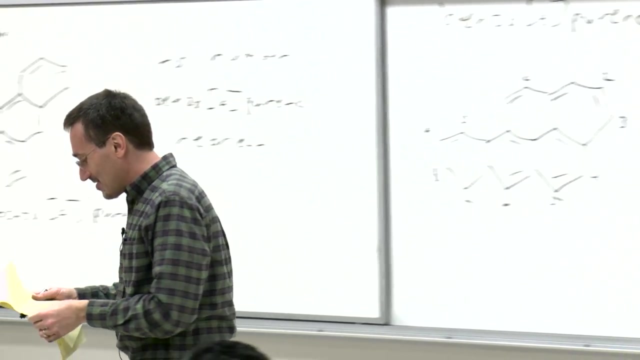 people have studied this. obviously we want to understand how cancer comes about. X-ray crystallographic structures of benzopyrene basically intercalated in and covalently alkylated to DNA, and so that stuff is just like one of the worst carcinogens you can possibly imagine. 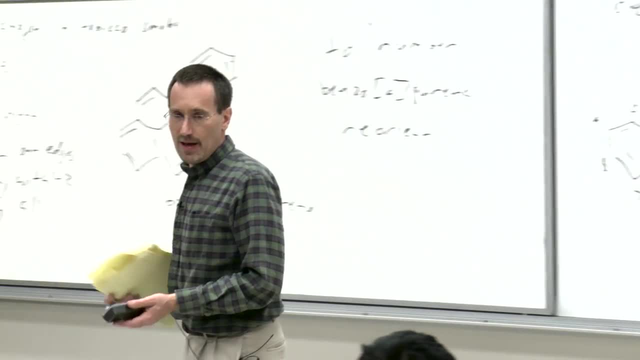 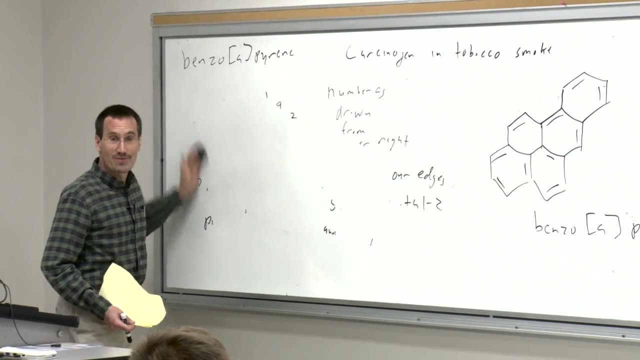 and we're talking micrograms of this compound, because you get a whole bunch of junk when you burn tobacco and you only get a little bit of benzopyrene. but a little bit of benzopyrene And benzopyrene is all it takes to really mess things. 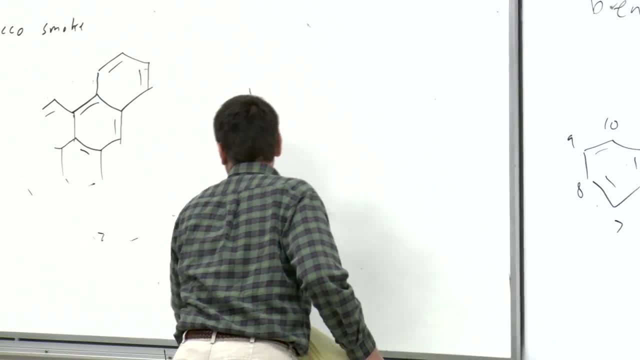 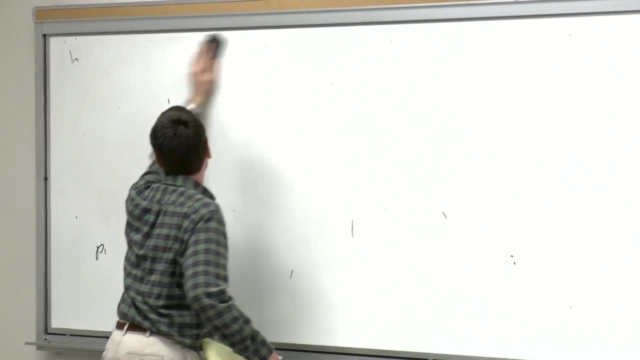 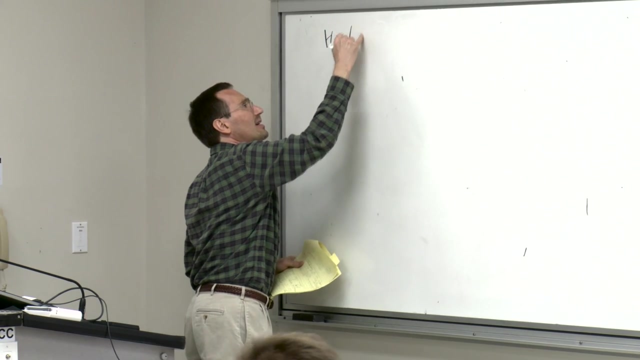 up with your DNA and your lungs are so, so vulnerable because you've got basically tissue exposed right there for all of those organic compounds to come in. Anyway, as I said, sort of beautiful and horrible at the same time. All right, I want to talk about heterocyclic compounds and I want 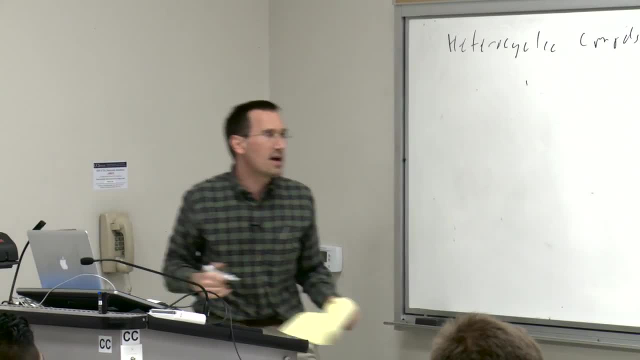 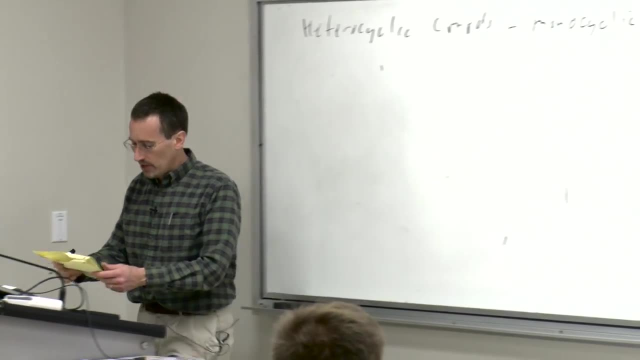 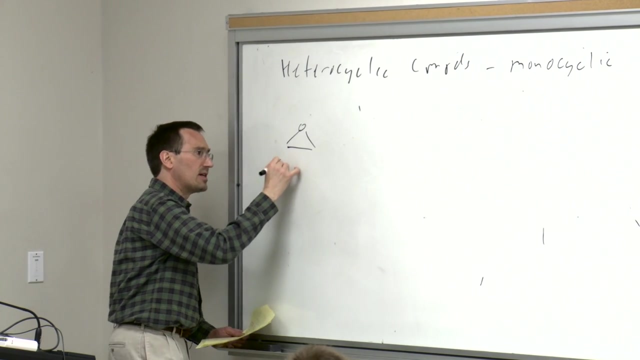 to take you through a few common ones. I'm going to talk about heterocyclic compounds, monocyclic, and then I want to show you another table to make some sense of it, and so I'm just going to write out a bunch that probably roll off of Sebastian. 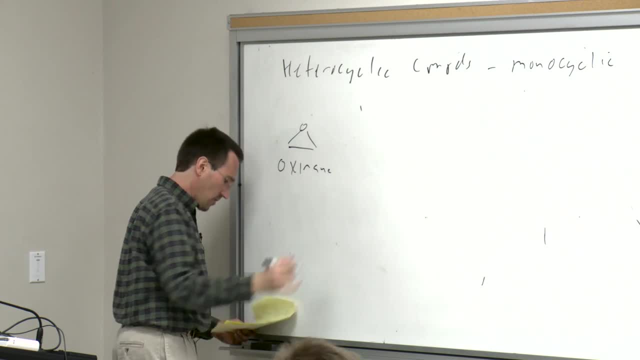 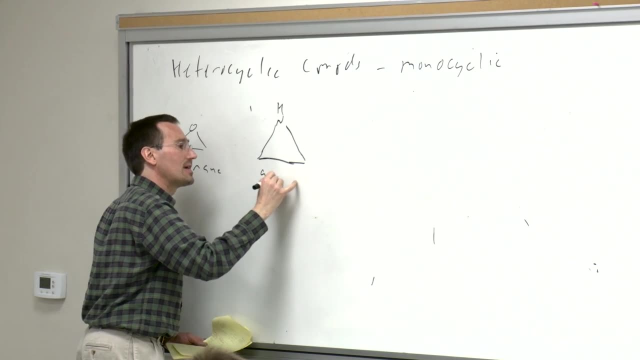 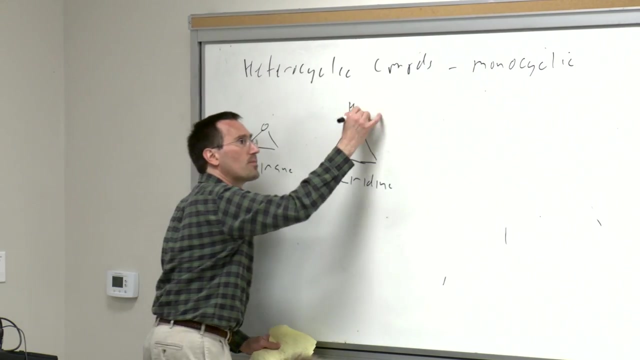 and Stan's tongue, oxirane aziridine. Now I'm not going to go through all of them. Now let me talk about the numbering, for a second. You number from the heteroatom, so you number 1,, 2,, 3.. 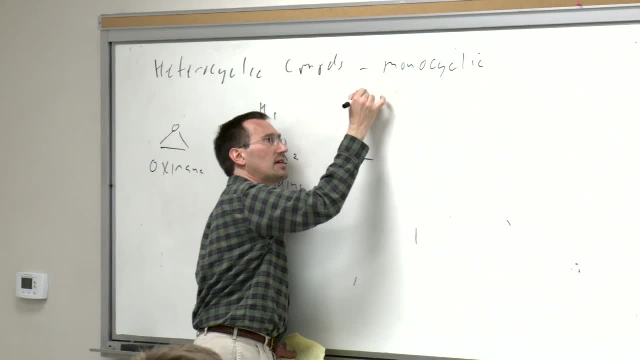 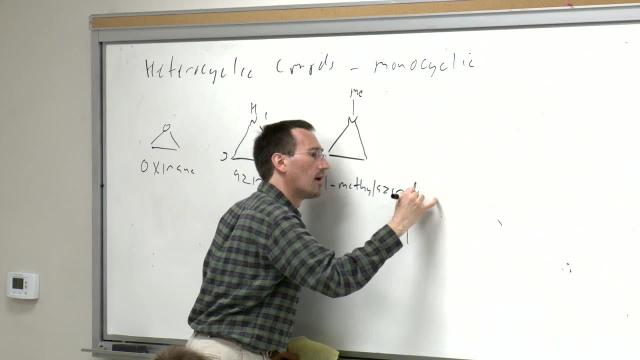 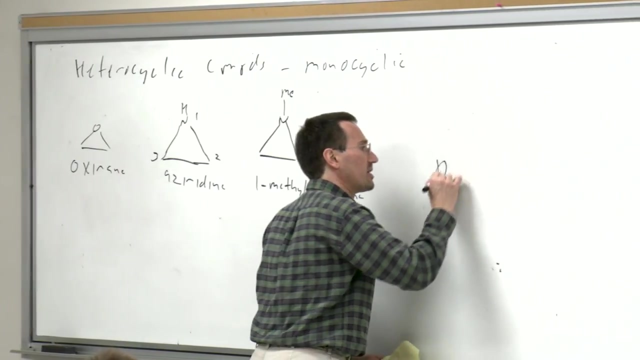 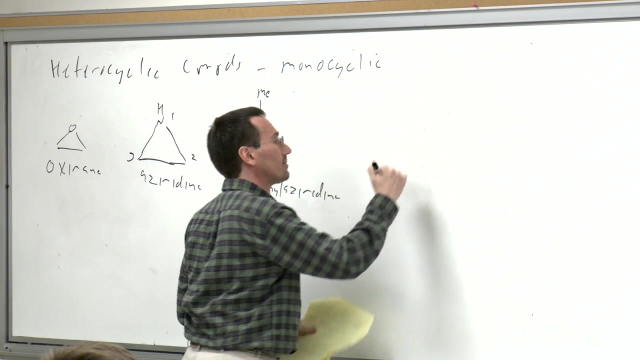 So if we go ahead and we say 1-methyl aziridine, this is 1-methyl aziridine. If I go ahead and say, let's say R2-methyl aziridine, oops, we're going to get a 1-methyl aziridine. 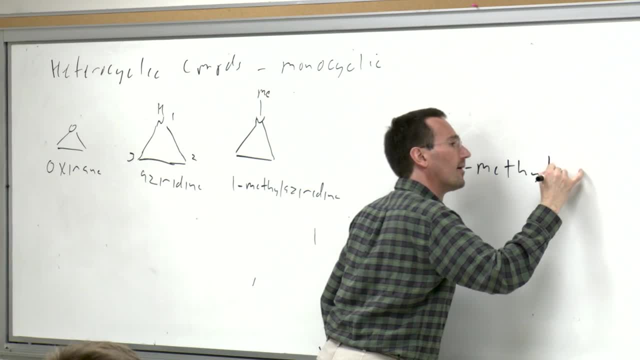 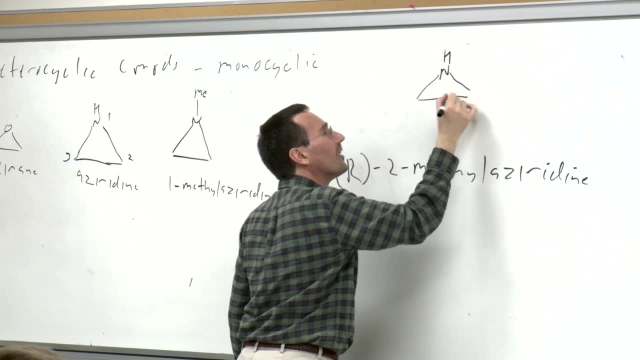 Now we're going to go ahead and say, okay, that means we have a methyl group on the carbon and we're going to put that methyl group so that we have the R stereochemistry and we'll remember. okay, there's a hydrogen here. 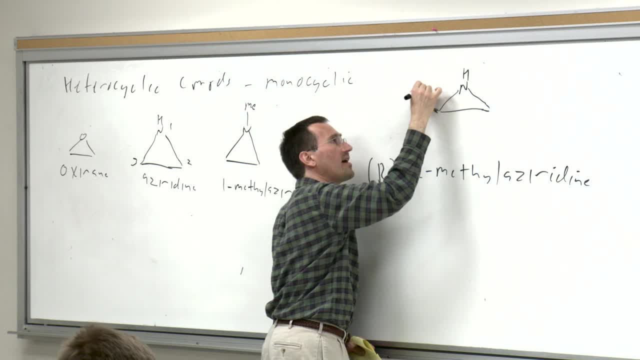 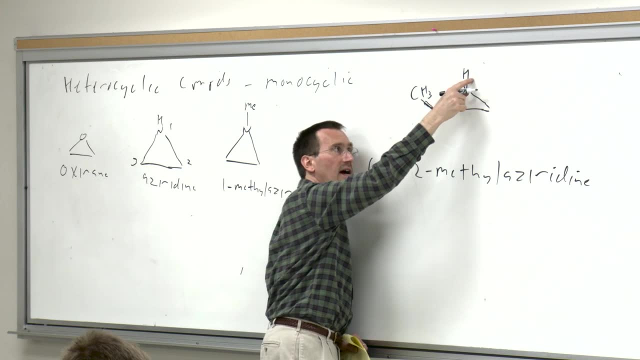 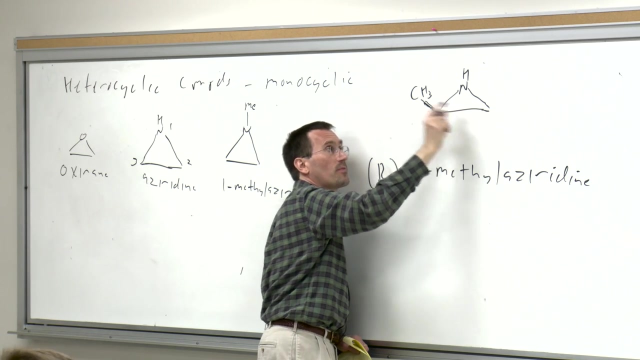 We side down to the bond to the hydrogen. Nitrogen has a bond to the hydrogen. We're going to put that methyl group on the carbon and we're going highest priority this carbon with just two hydrogens and one carbon attached to it and a nitrogen higher priority than the methyl. so 1,, 2, 3.. 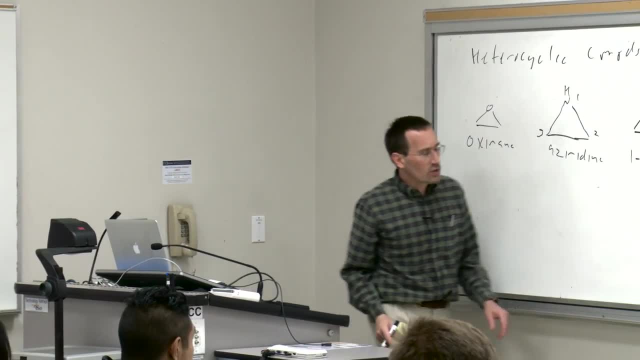 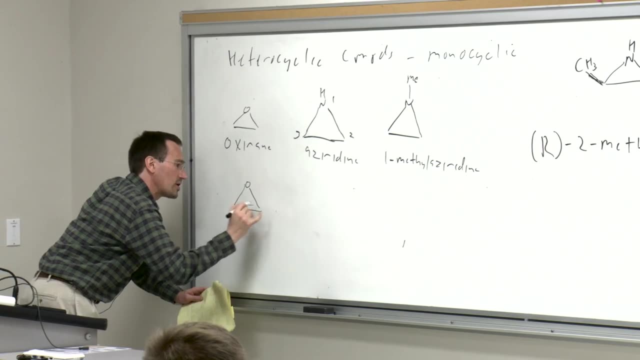 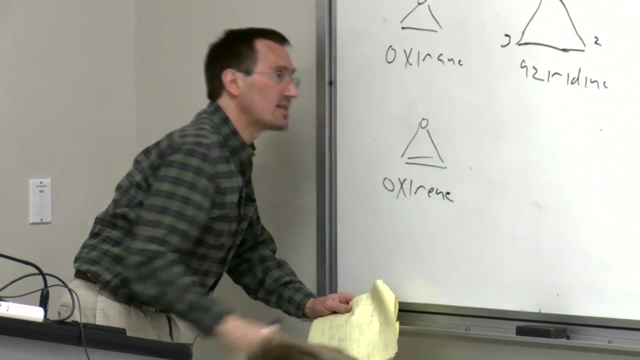 So there's our group And there are all sorts of other names. if you have a double bond- and I'm going to show you how to make sense of all this in a second, so don't worry too much. Oxyrhine, that makes sense. 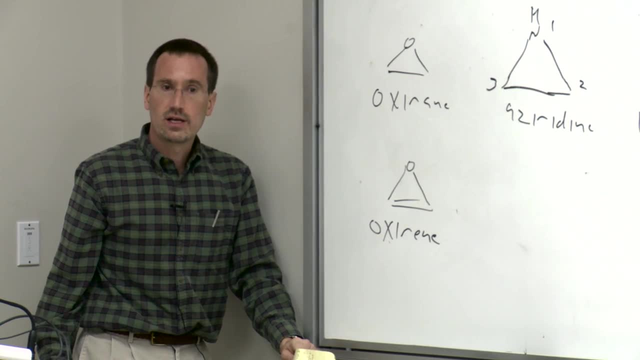 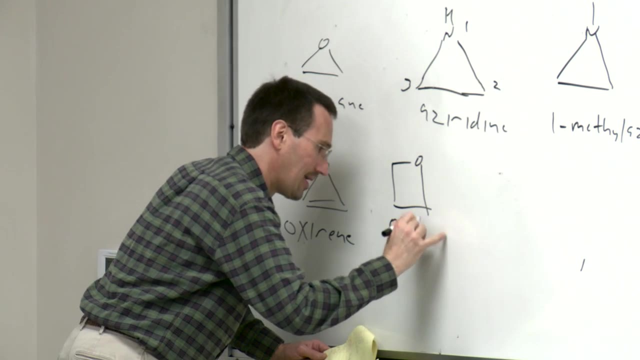 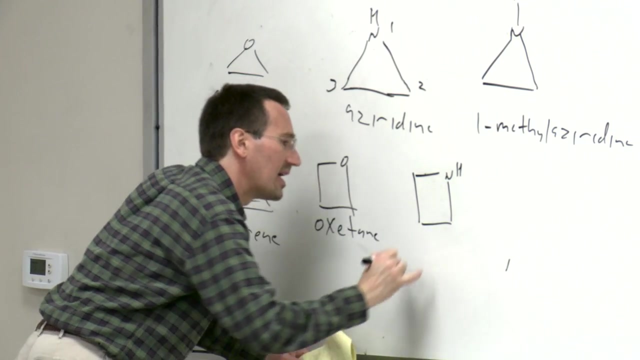 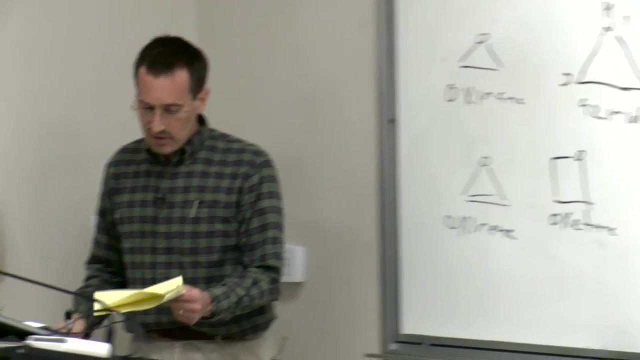 We've got a double bond: A and E for saturated E and E for unsaturated oxytain, and, as I said, if you use these a lot they roll off your tongue. azetidine, and then, just to have some fun, 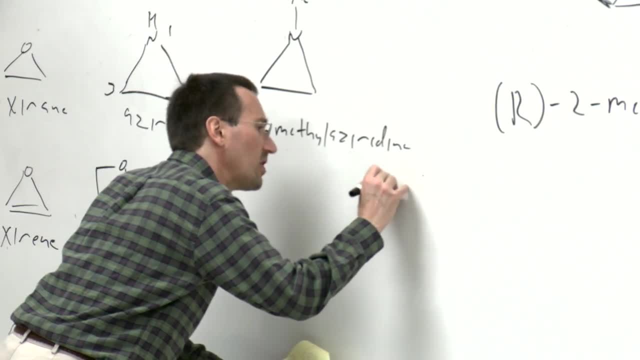 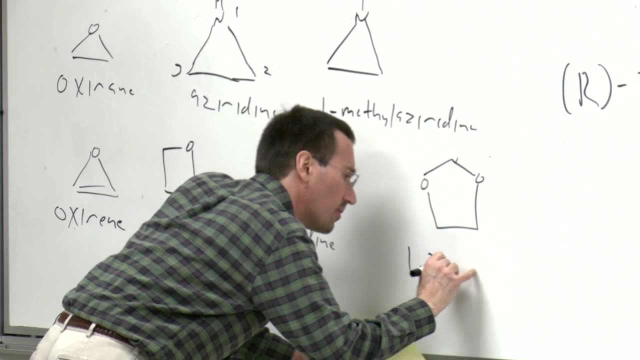 let's do a few variations here. So if we do a 5-methylchloride 6-membered ring with two oxygens, it's going to be 1, 3 in the 1 and 3 position will be 1, 3-dioxylane. 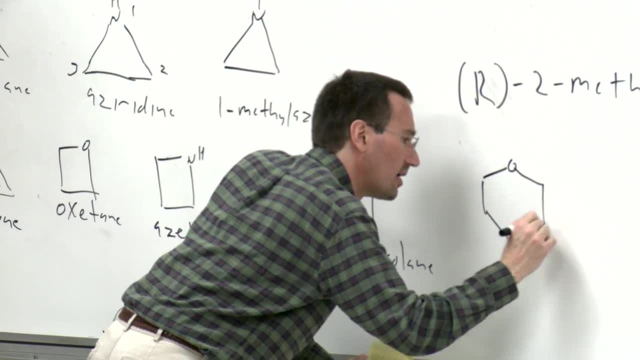 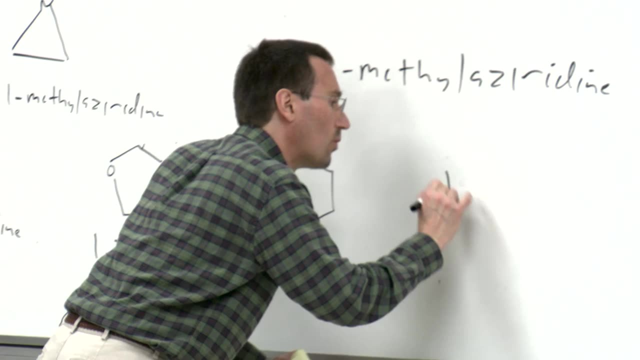 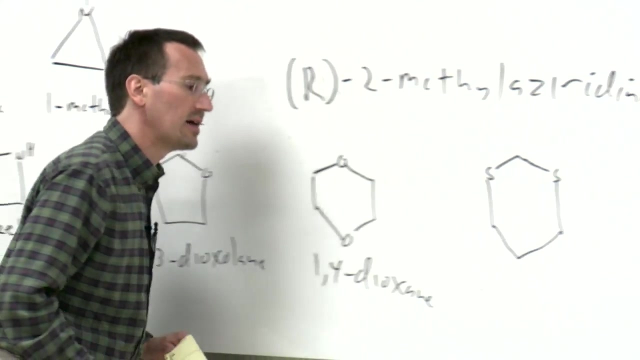 You might have seen for as a solvent 1, 4-dioxane. and let's say- I'll give you one more example- I think we're going to see this in our chapter on synthesis, where they talk about oompa-lung. 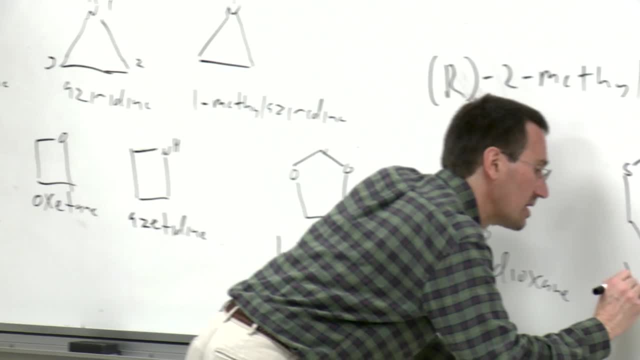 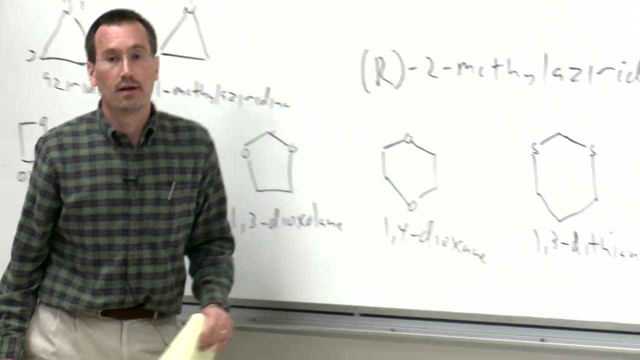 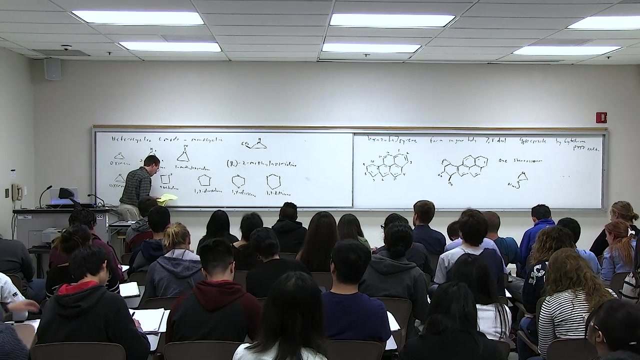 and this is 1, 3-dioxylane, This is 1, 3-dithiane. Yeah, Oh, with the dioxylane, is it dio or diox? Oh, diox, no dioxylane. 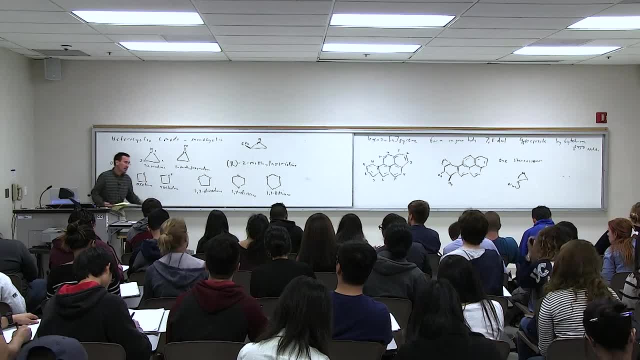 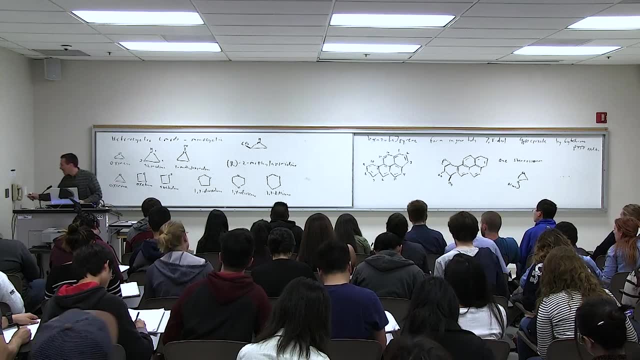 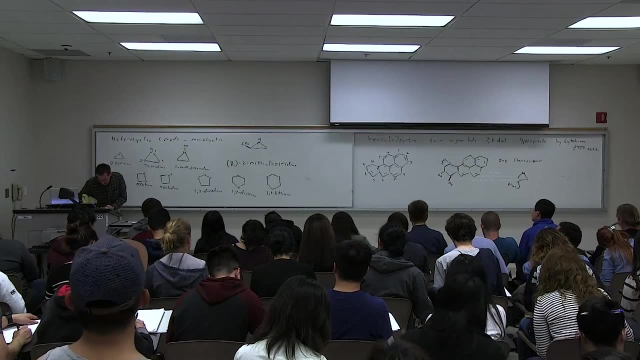 Diox, yep, dioxylane, So it doesn't follow the, Doesn't follow it. Now Let me show you the key on all of this, and I want to put all of these into context here. So remember, I told you that those tables had a lot. 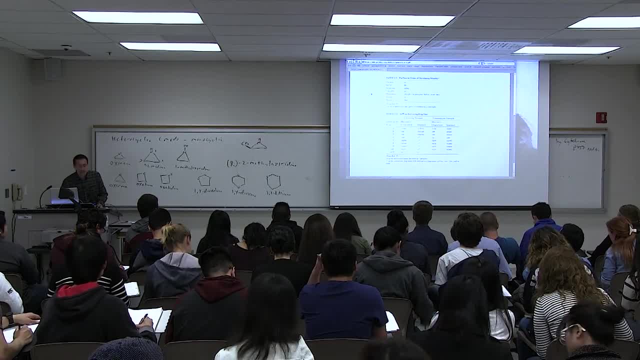 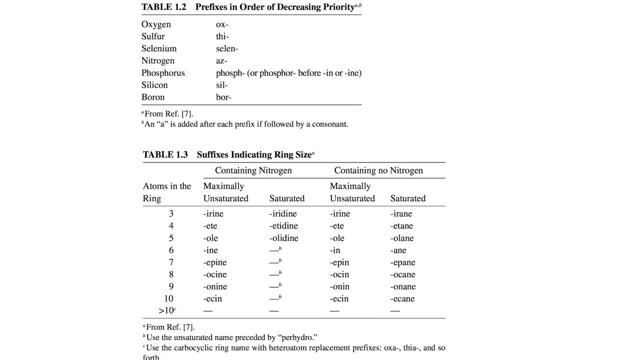 of good stuff in them. Okay, Tables 1.2 and 1.3 make sense of all of this craziness. Let me go ahead. I'll make this a little bit bigger for us All right? Making sense of all of this craziness. 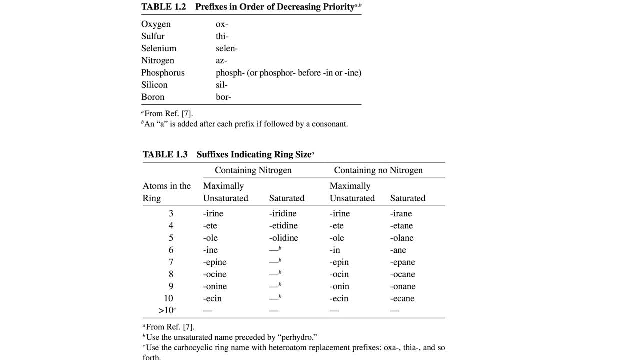 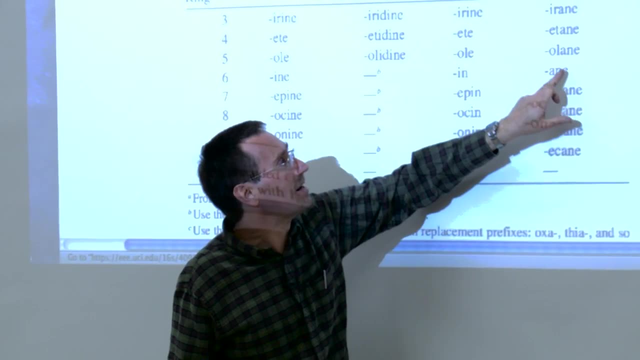 So you choose your atom. ox, for example, ox, Two oxygens. if there are two oxygens, You choose whether you have compounds containing no nitrogen or nitrogen. No nitrogen, You choose whether they're saturated or unsaturated Dioxylane. 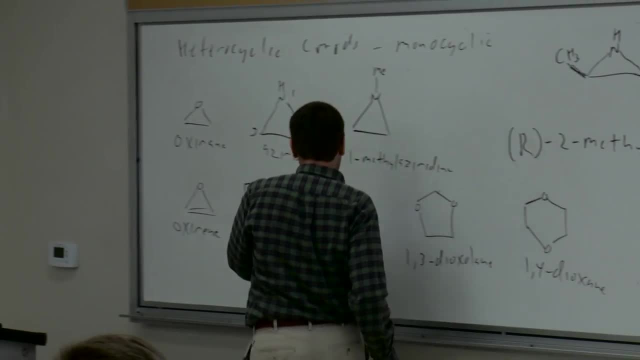 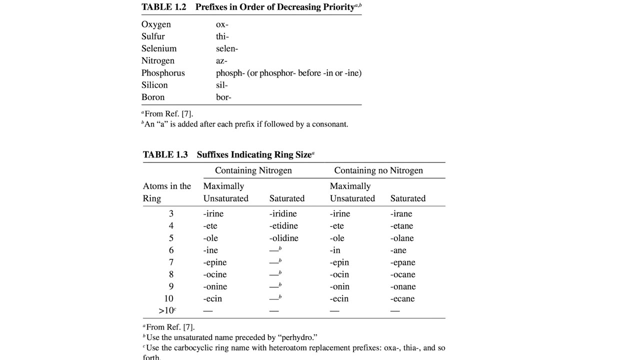 If you have. so what about that crazy oxetane? but azetidine business here. Okay. Compounds with ox oxygen: get ox. Compounds with nitrogen: get A's. Compounds containing nitrogen go under this category here. Four-membered ring azetidine. 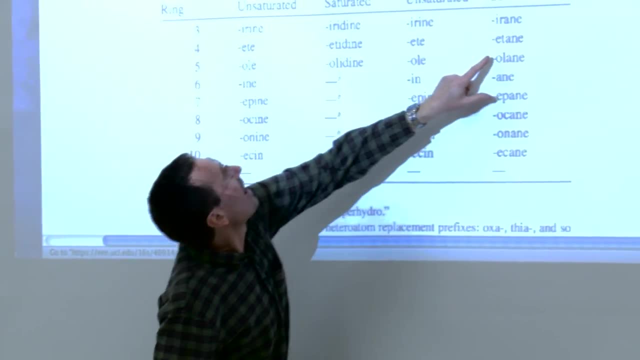 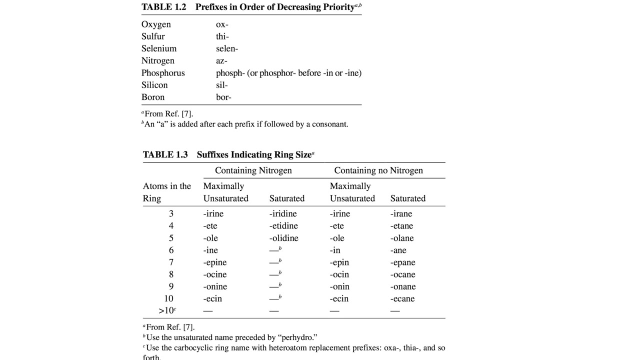 Compounds without nitrogen oxetane here. So basically, it's just run down the table. Okay, It's just run down the table. un-naming them? Yeah, Would something like 1,3-dioxylane the way? 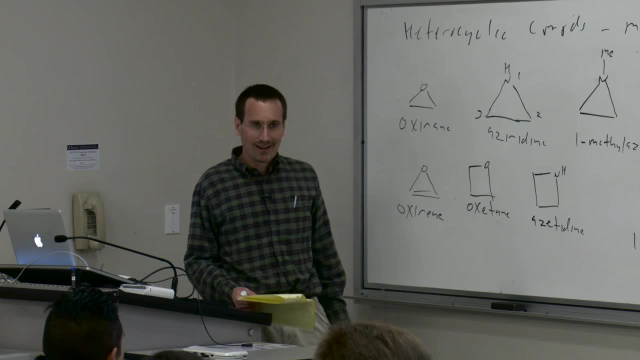 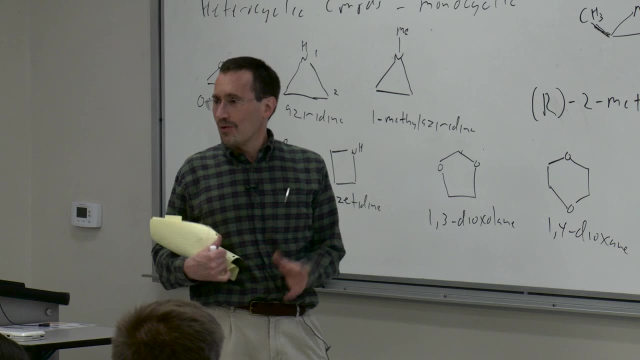 Wouldn't you just call it like a 1,3-dioxyl pentane? You could. You could, Certain compounds have special names And I want you, when you're seeing all of this, take it in Also. have a little bit of a laugh at this. 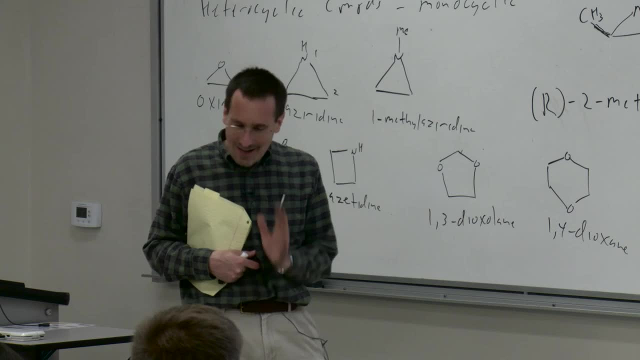 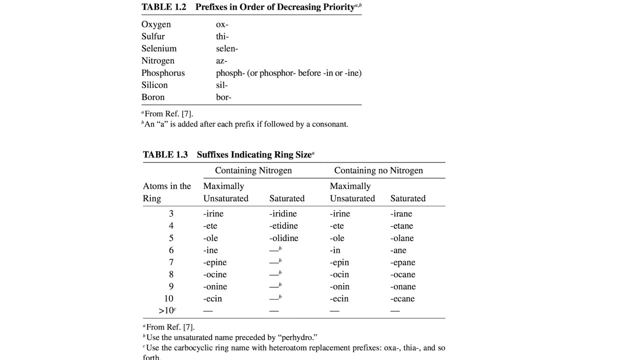 Because some of this, some of this is funny, Some of this is funny, these arcane rules, And again realize, if I ask you anything from this, I'll give you the table. Just have worked through it once as you're working through the chapter and the homework problems. 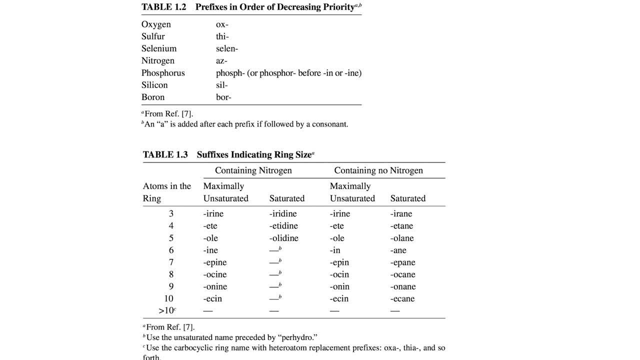 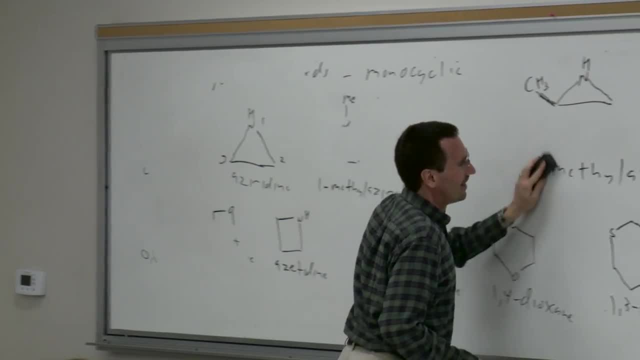 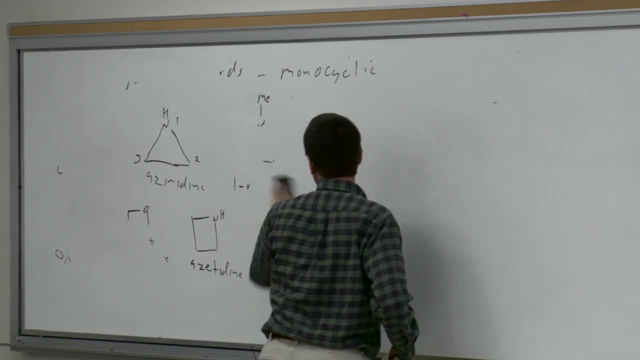 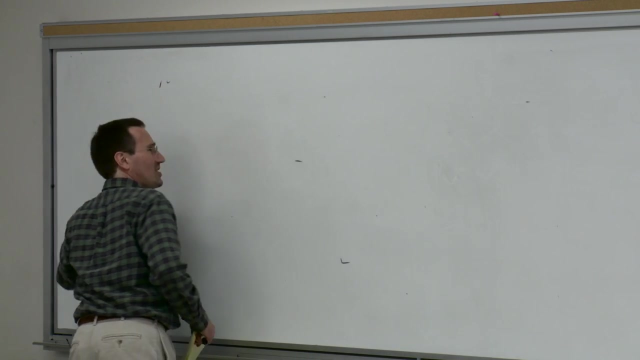 Make sure you internalize it. But it is sort of funny. Now things get even funnier here. All right, Things get even funnier because all of this you can say at least by some way, shape or form is systematic. 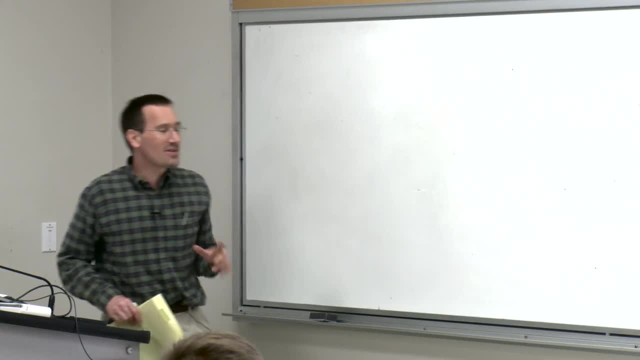 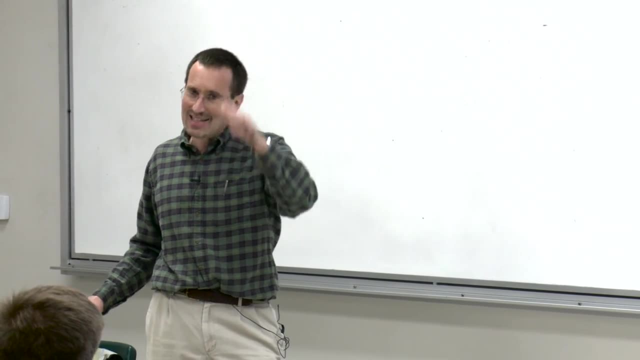 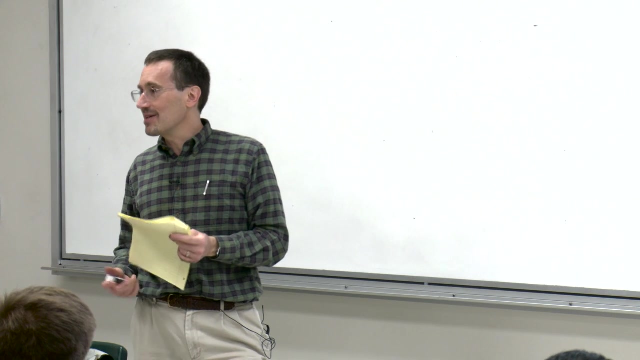 In other words, oops, Okay, In other words, it may not make sense that it's ezetidine but oxetane, but you can walk through a system, You can talk about it. These are molecules that got their names when we understood structure. Or at least got their names. that really stuck when we understood structure. But all of those names like phenanthrene and anthracene came from organic chemists, sort of in the 19th century and maybe early 20th century, where organic chemistry was isolating stuff. 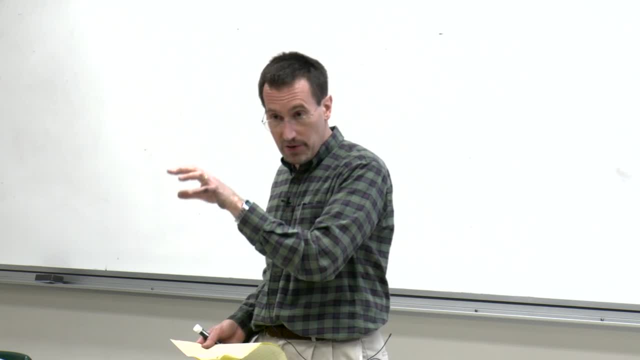 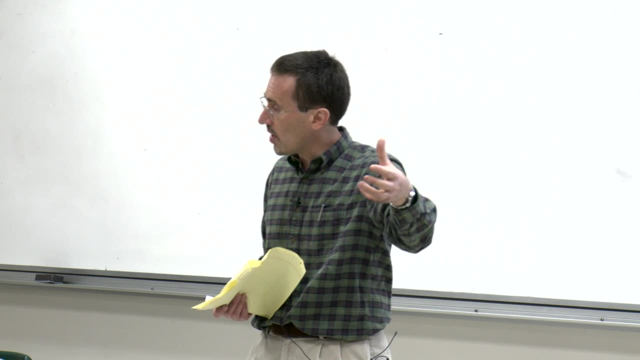 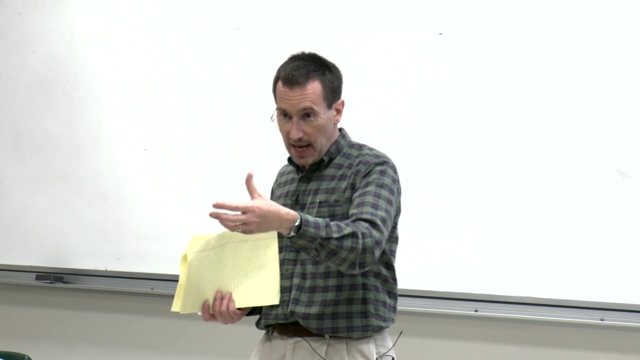 Figuring out: okay, it has this melting point, so it's a pure compound. When I burn it and I calculate how much CO2 and H2O are produced, I get an empirical formula of, say, C10H8. and so you say, okay, I don't know the structure. 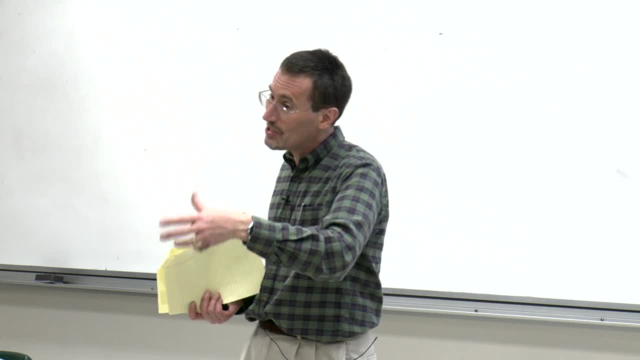 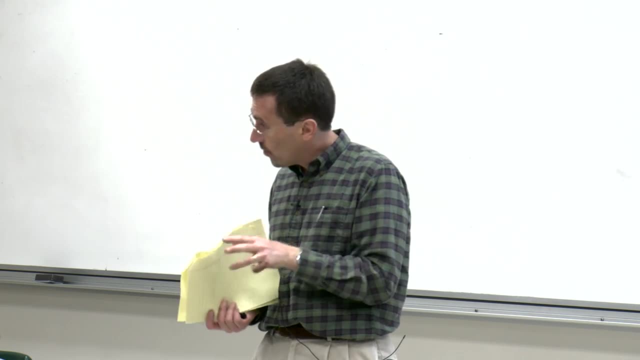 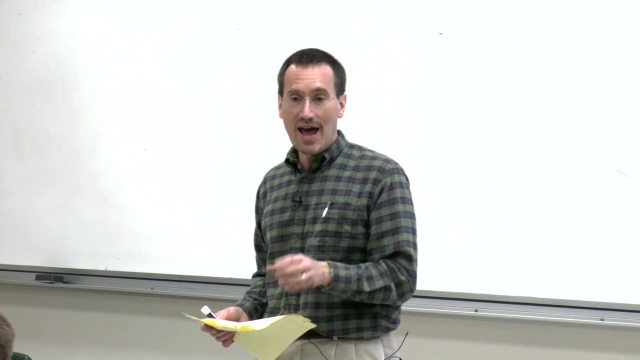 of naphthalene, but I know it is C10H8.. And then, as understanding came along and we understood the valences of carbon, we eventually were able to piece out the structure, But a lot of these initially got the name that they were. 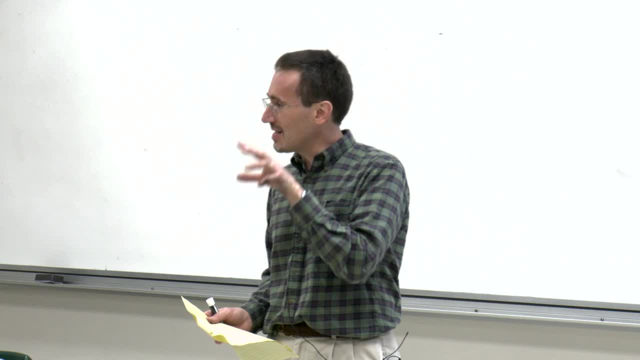 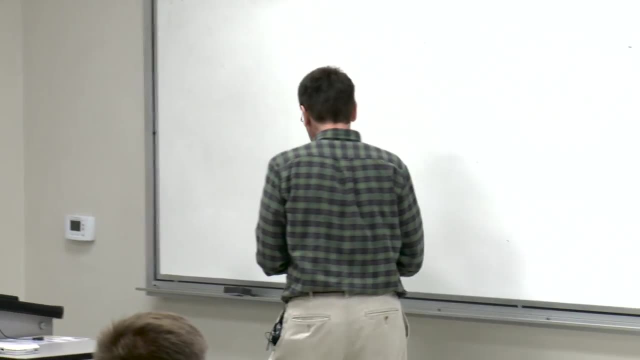 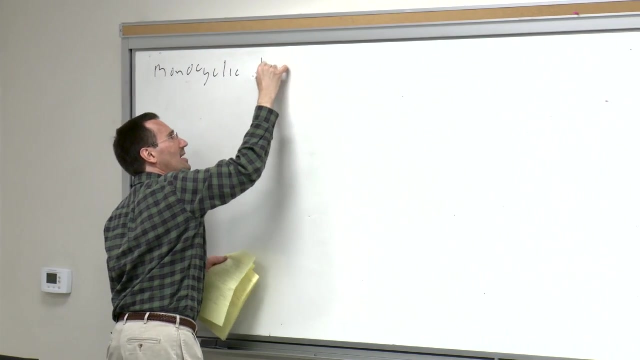 you know, this was the molecule that I isolated when I heat distilled anthracite coal, So okay, So with that there are certain monocyclic, heterocyclic compounds and carb. well, all the carbocyclic ones of course I'm talking about have sort of well. 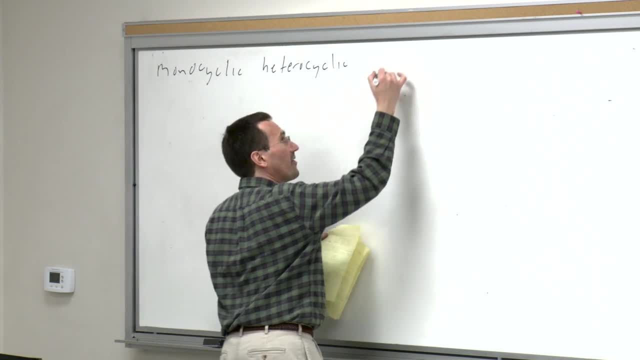 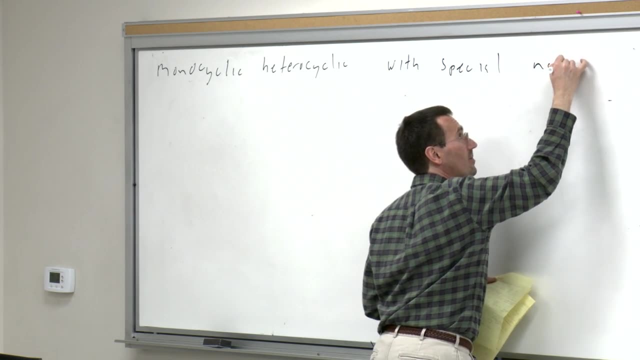 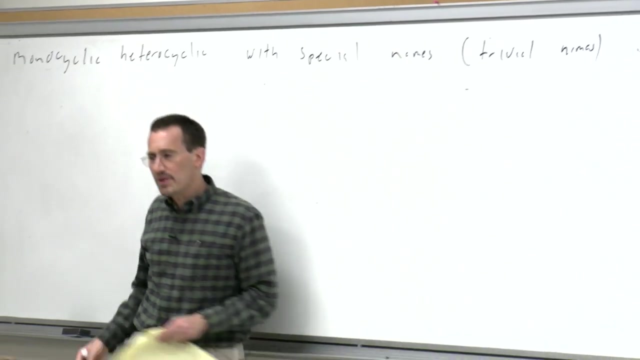 at least the 35 that I mentioned sort of have crazy names, special names. so I'll say: with special names, you can call them, you can call them trivial names. These are the names that came before people knew their structure and stuck. 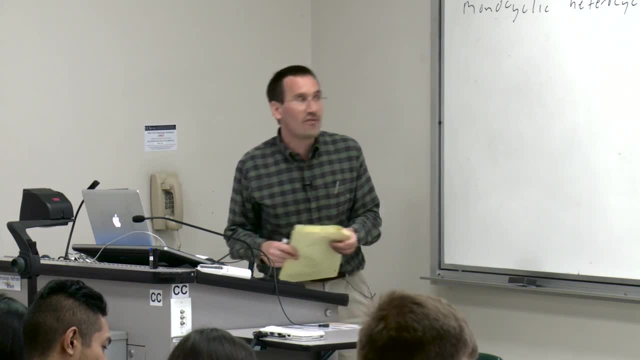 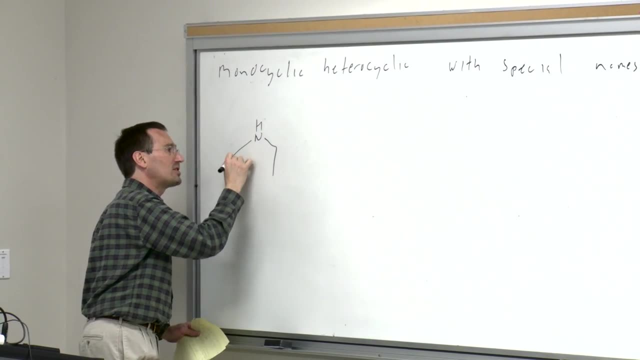 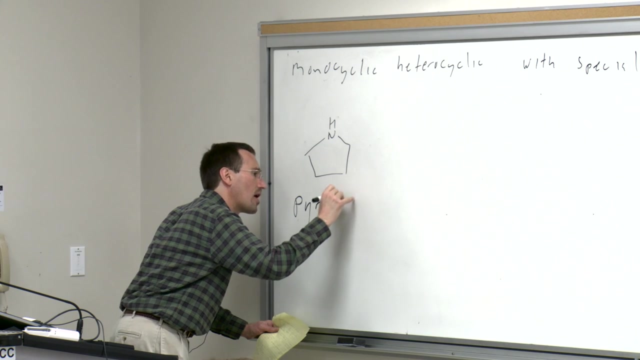 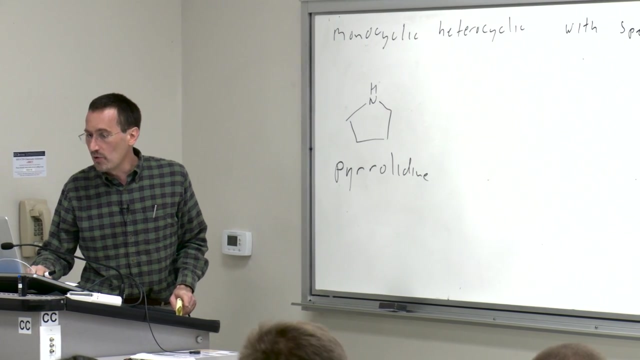 And they just roll off the tongues of organic chemists. So, for example, breaking the rules on the tables 1.2, this molecule here is called pyrrolidine, p-y-r-r-l-o-i-d-i-n-e. And again, don't. I'm going to take us back here and again. 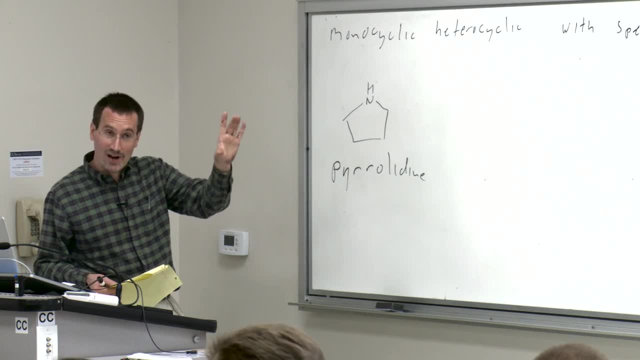 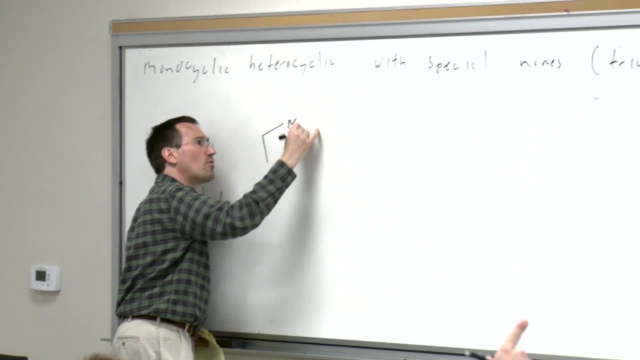 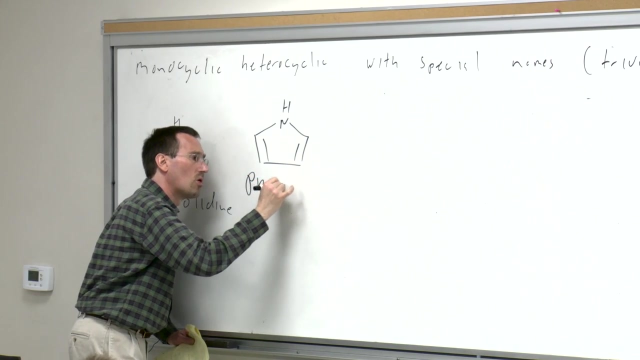 I'll sort of take us over to this, So don't stress too much about this. Have a little bit of laugh of history, But these are ones that also roll off of Stan's tongue and Sebastian's tongue. This molecule is called pyrrole. 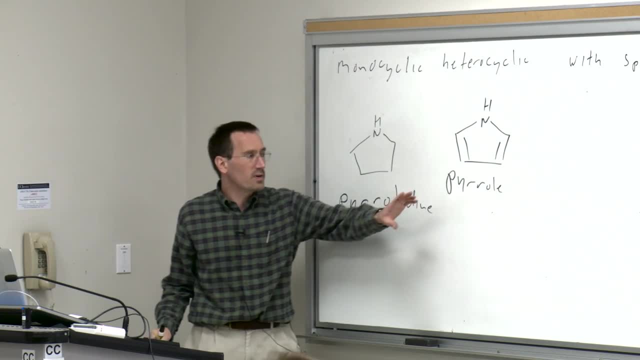 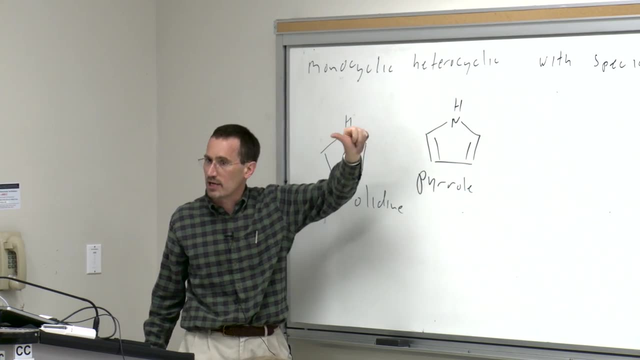 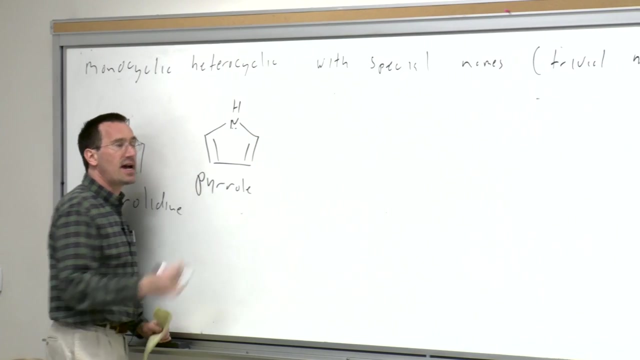 We're going to talk a little bit about aromaticity in the course, but I hope that you remember from sophomore organic chemistry. when you have six pi electrons in a ring you have special stability of an aromatic compound. There's a lone pair on this, nitrogen. 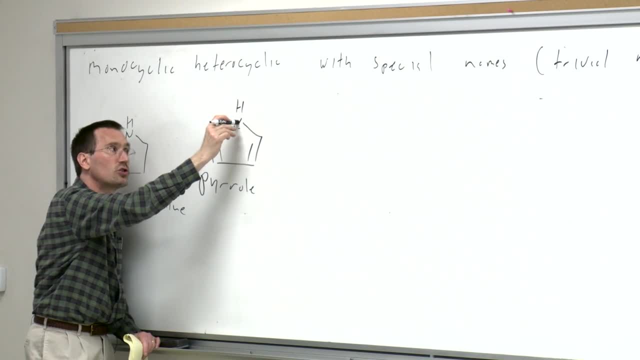 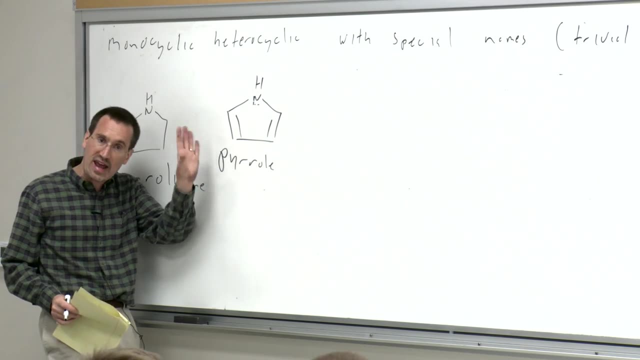 That lone pair is in a p orbital, and so we get 2,, 4, 6.. Pyrrole is an aromatic molecule like benzene. although with about half as much resonance stabilization, It's much more reactive in electrophilic aromatic. 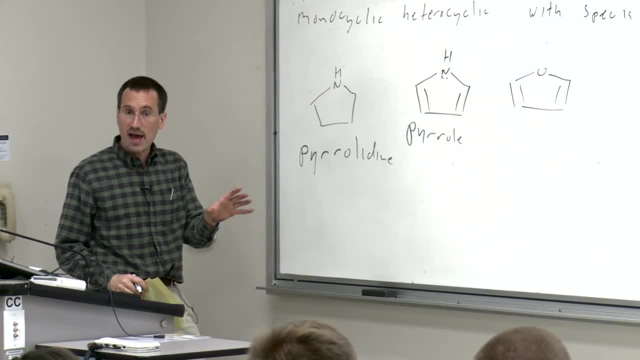 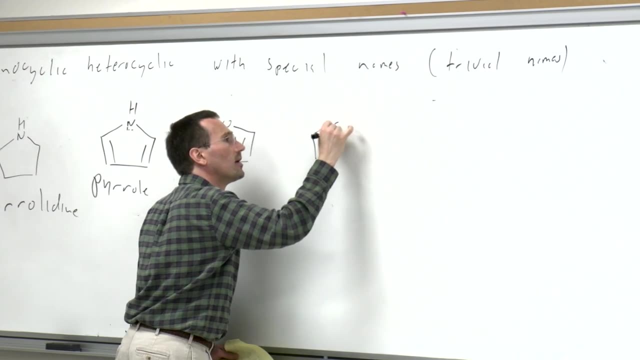 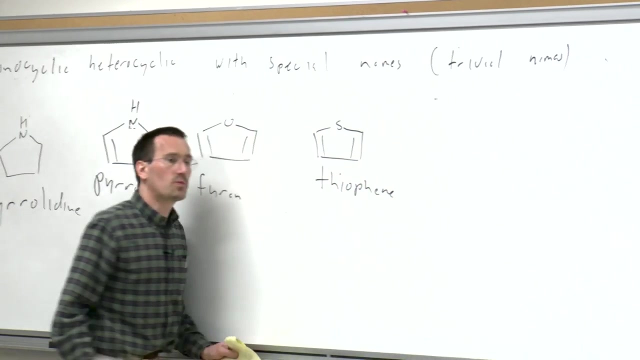 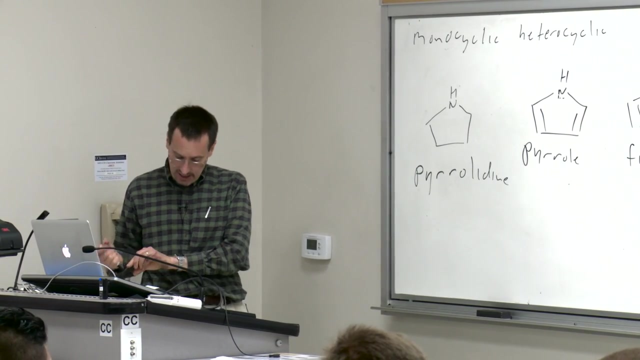 substitution, but it still behaves like an aromatic compound, not like an alkene. This molecule here is called furan, This molecule here is called thiophene, And again, most of these molecules would go back to isolation before people had systematic understanding. 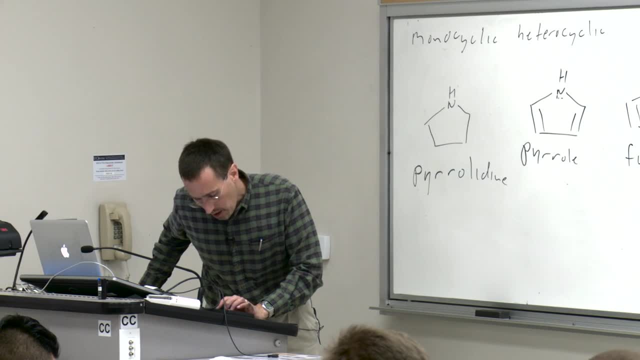 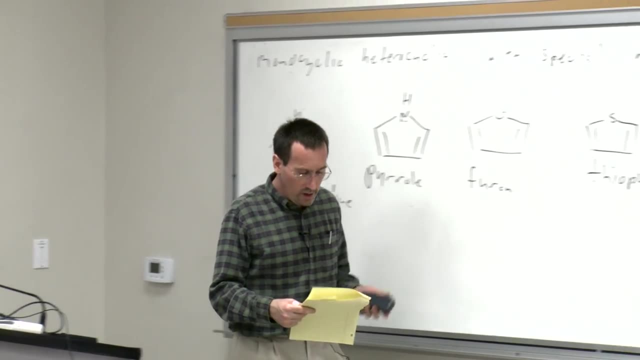 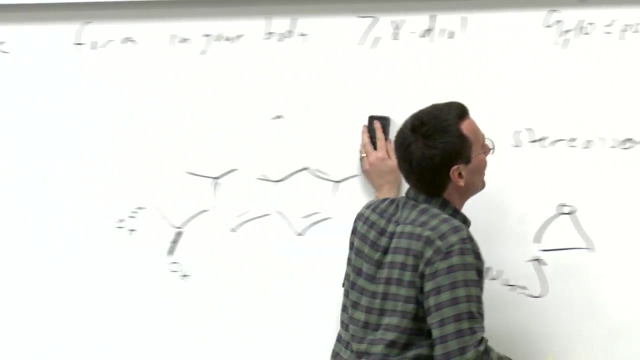 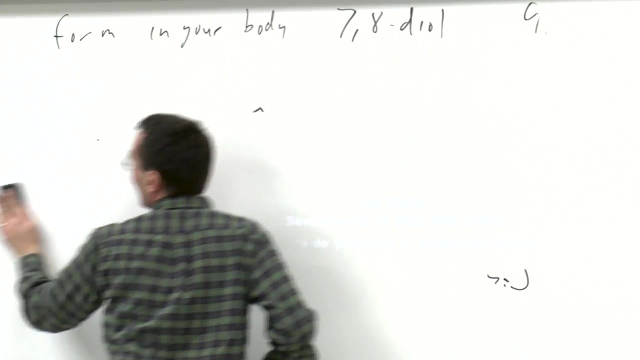 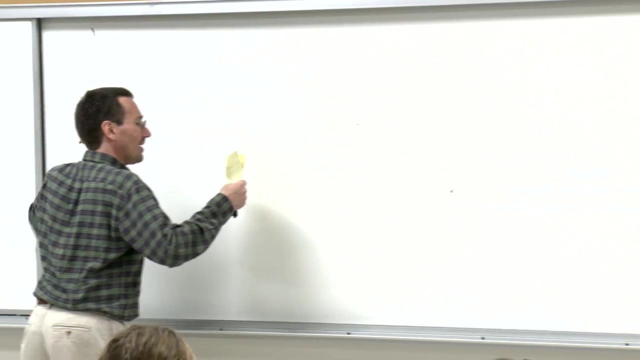 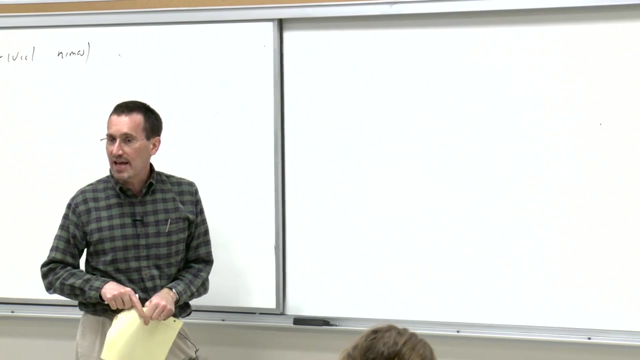 of their structure. All right, So let's see. So I think I want to conclude With a couple of comments about unsaturation here. All right, So for unsaturation, we take a lot of these names and we note. 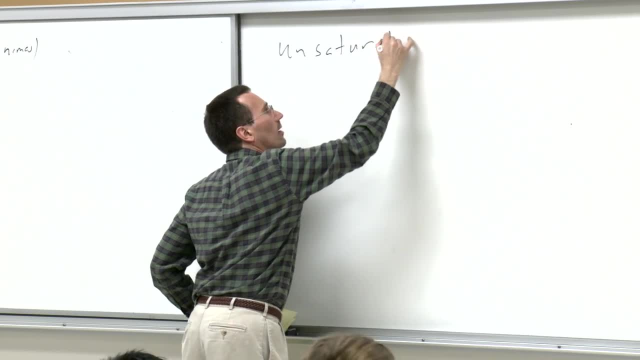 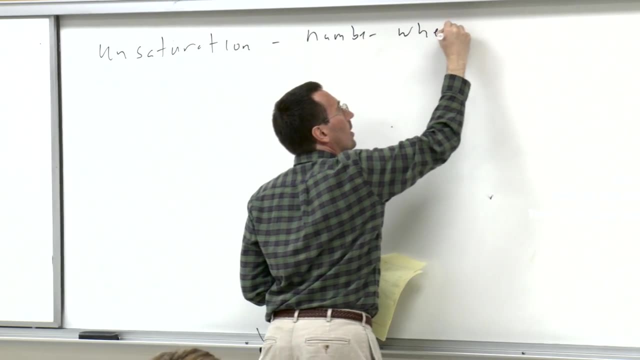 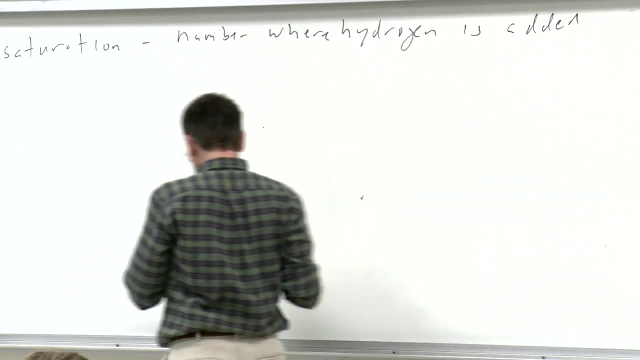 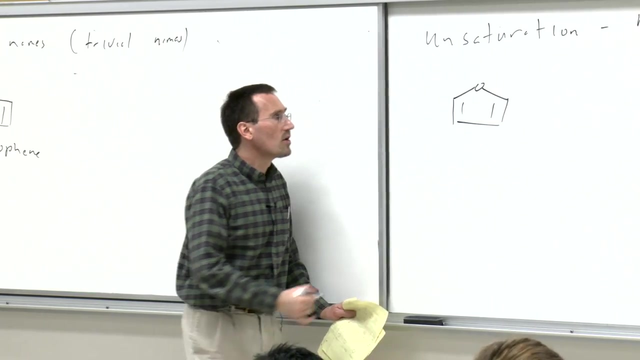 down where the hydrogen is added. All right, So let's start with furan. Okay, So here's furan. We number it, starting with the heteroatom 1,, 2,, 3,, 4,, 5.. 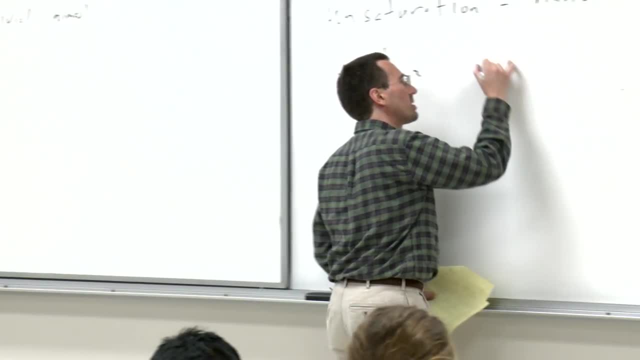 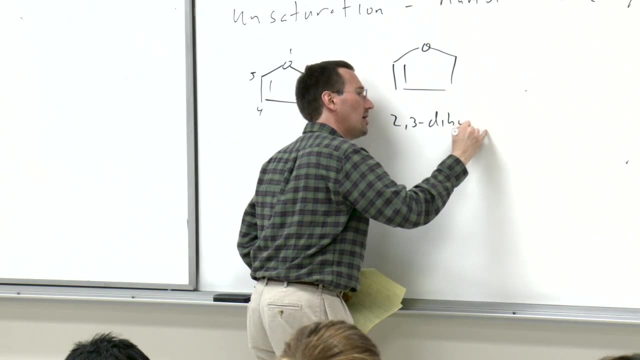 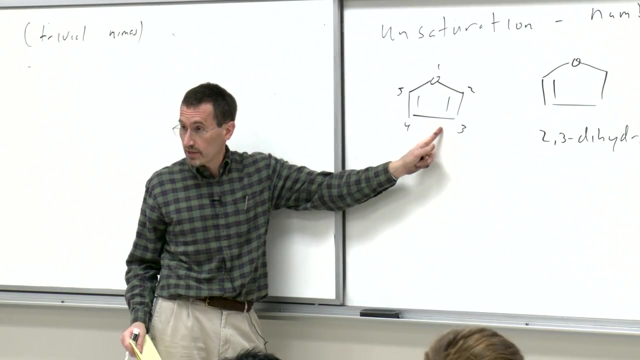 And so if we add two hydrogens to the molecule, we come up with 2, 3 dihydrofuran. if we've added them across the 2 and 3 positions, If we add them across the 1 and 5 positions, 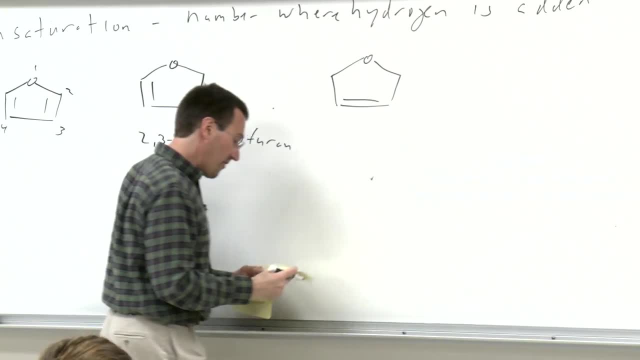 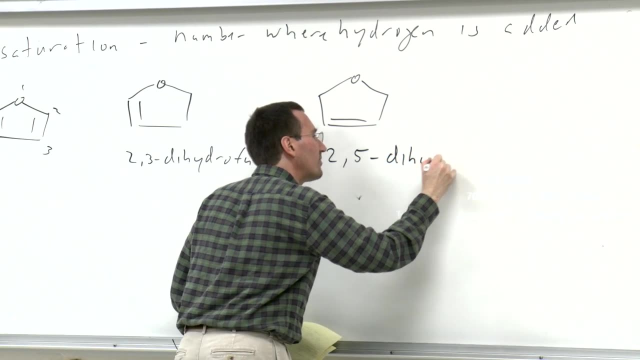 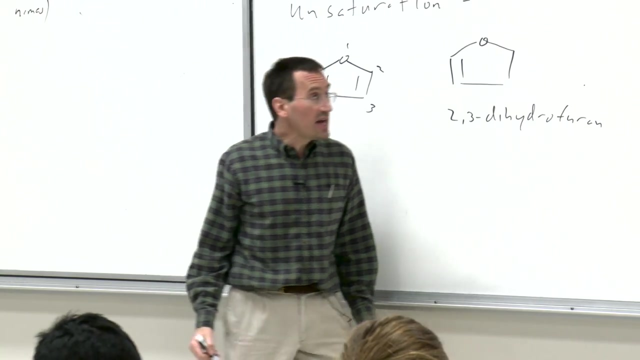 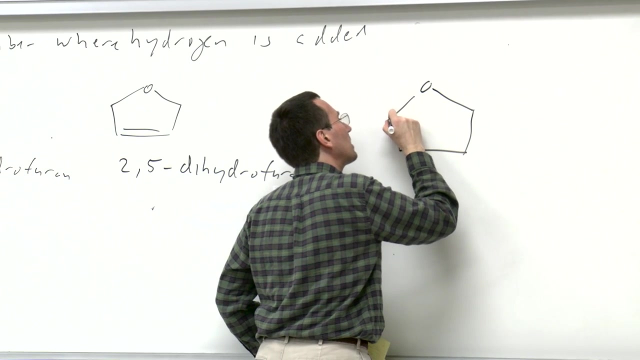 we now have 2, 5.. I'm sorry, across the 2 and 5 positions We now have 2, 5 dihydrofuran And hopefully all of us have seen this molecule in the course of our sophomore organic chemistry. 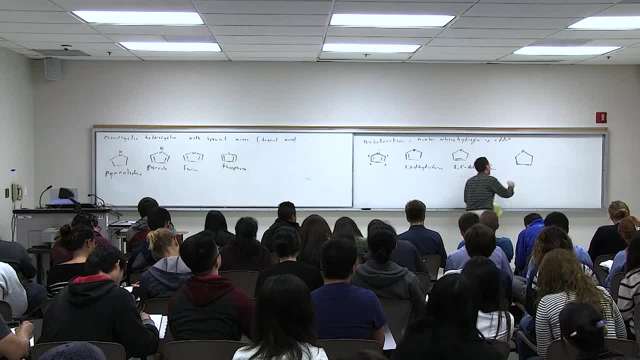 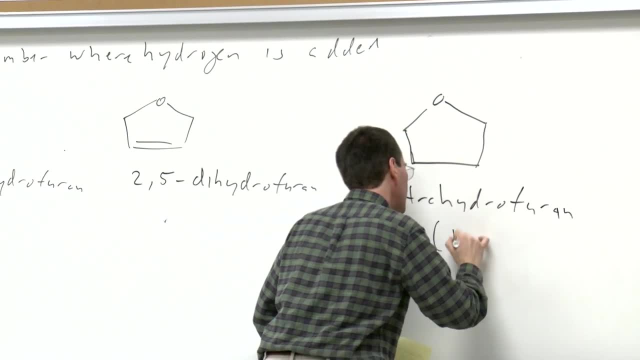 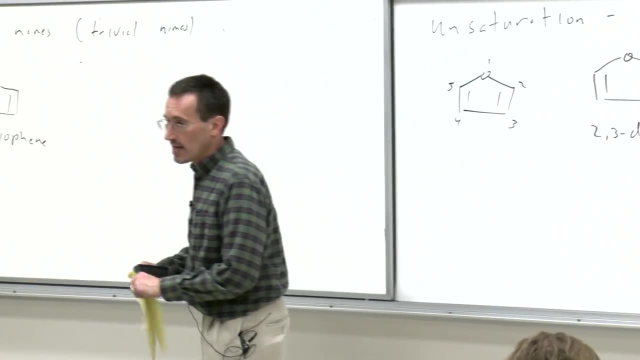 What's the name of that molecule? Tetrahydrofuran, Tetrahydrofuran. All right, So that's it, Thank you, Thank you, Thank you. Commonly called THF, THF is widely used as a solvent in, for example. 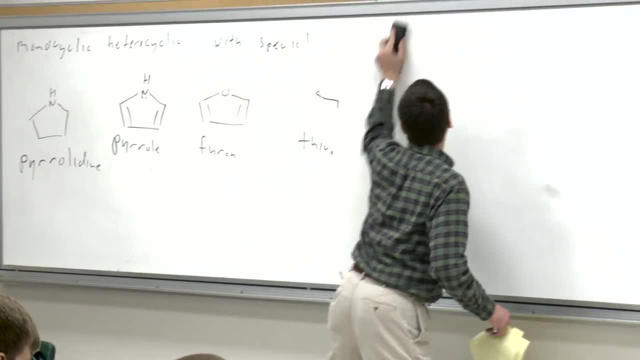 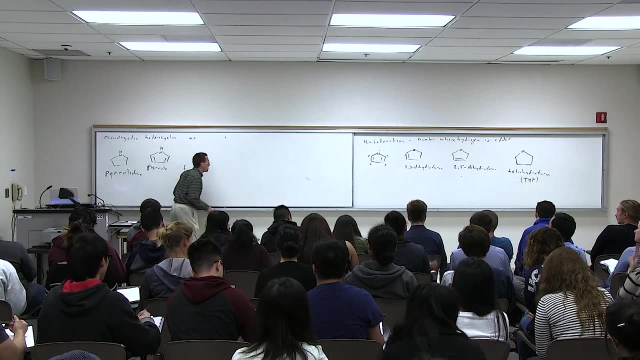 Grignard and organo-lithium reactions. I think we use it widely. Who's had the CHEM 160 class, by the way? Oh, okay, And we've probably used it. I'm pretty sure we use it in the CHEM 160 class, for certainly the first reaction is an. 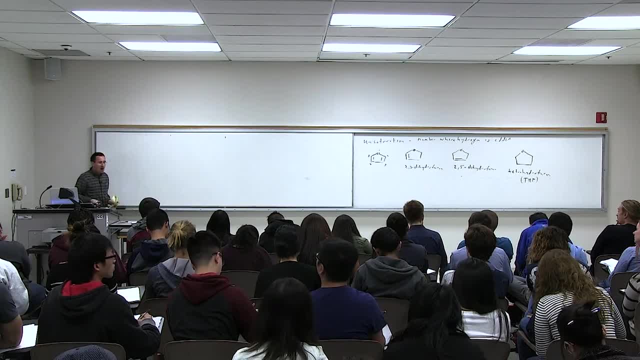 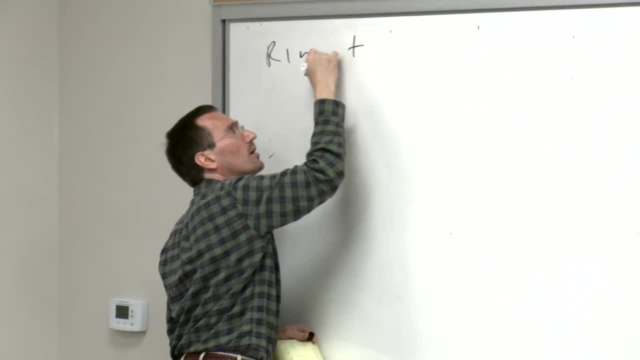 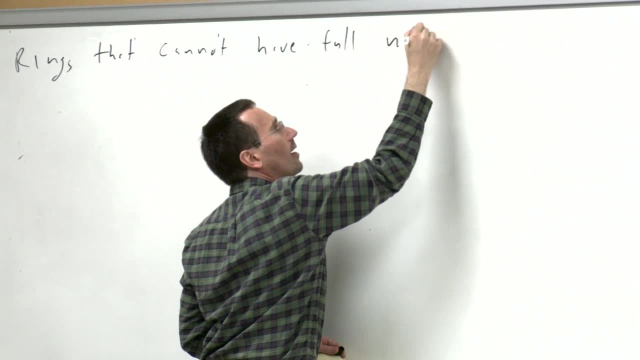 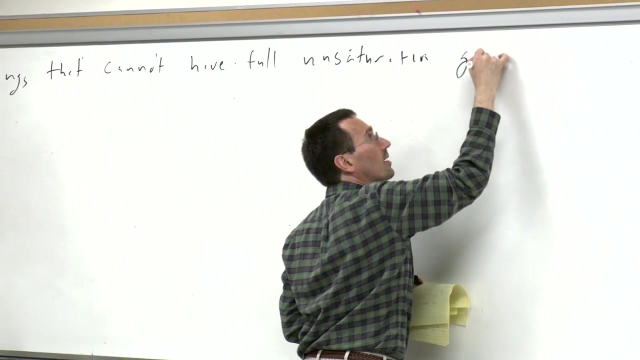 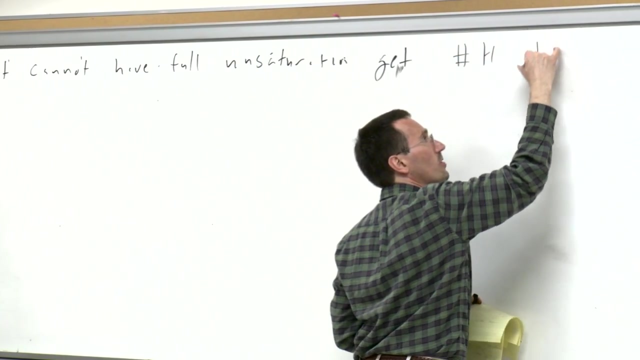 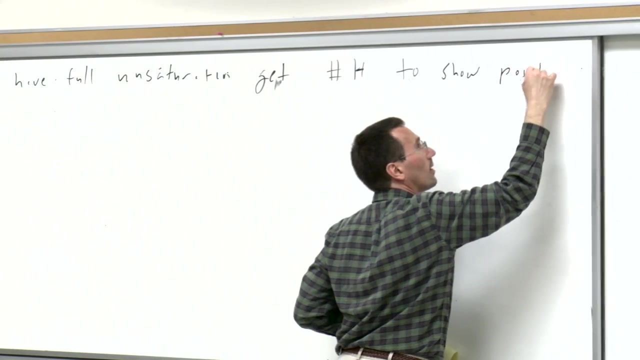 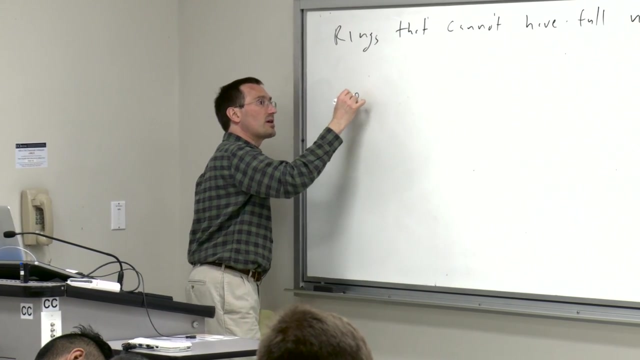 nice aldol reaction and I think we run it in THF All right. last thing I want to say: Rings that cannot have full unsaturation get number and age to show the position, All right, so take a six-membered ring. 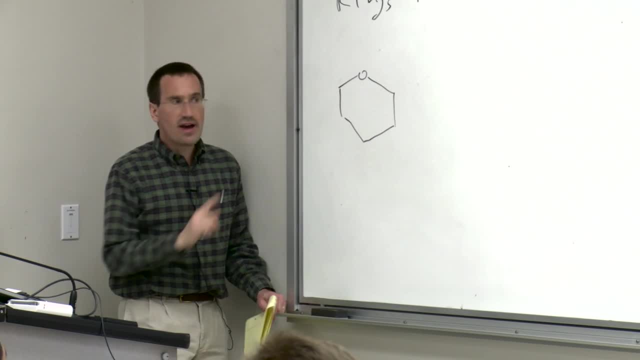 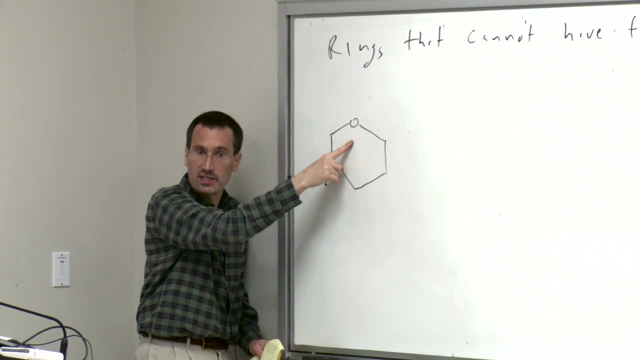 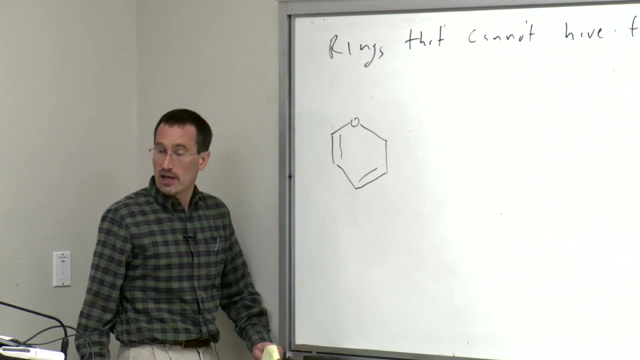 with oxygen in it. I cannot have a neutral six-membered ring with oxygen with three double bonds. I can have three double bonds and a positive charge on oxygen. that's called perillium. but the only neutral molecule I can make- I mean any neutral molecule I can make- 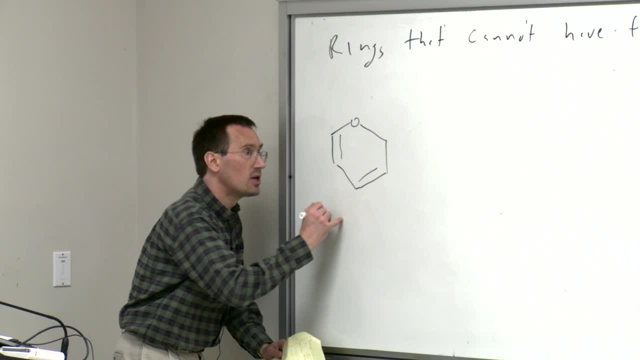 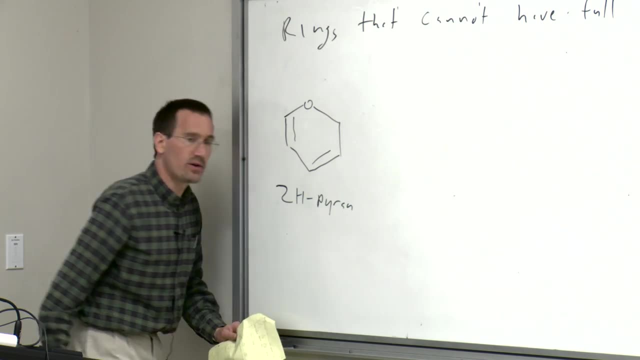 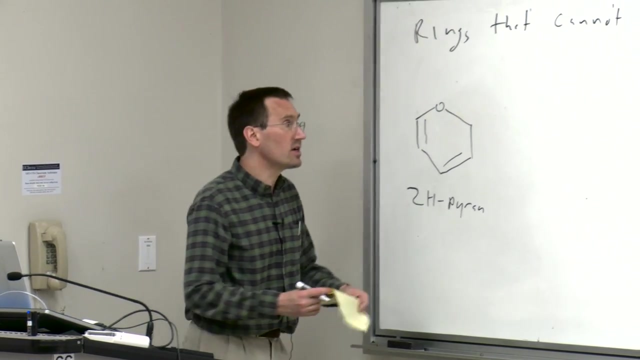 has one carbon that is unsaturated, So we call this molecule 2H pyrran. Pyrran was one of those trivial names on your chart And then if we're going to do a numbering around the ring, so it basically is one. 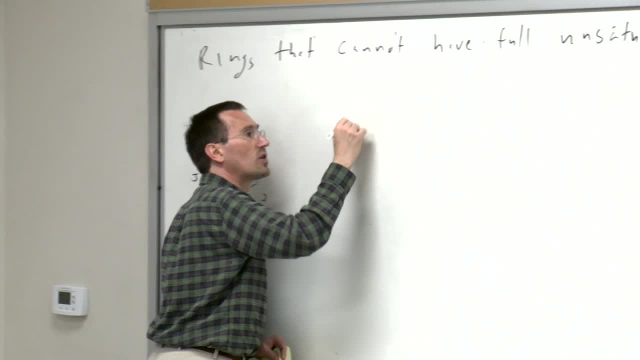 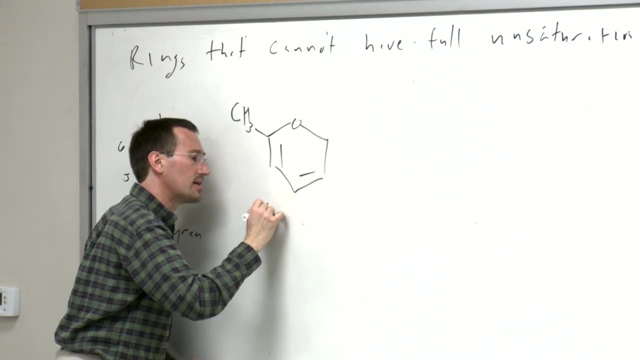 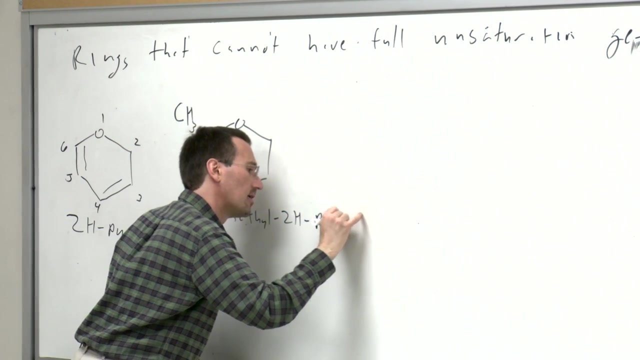 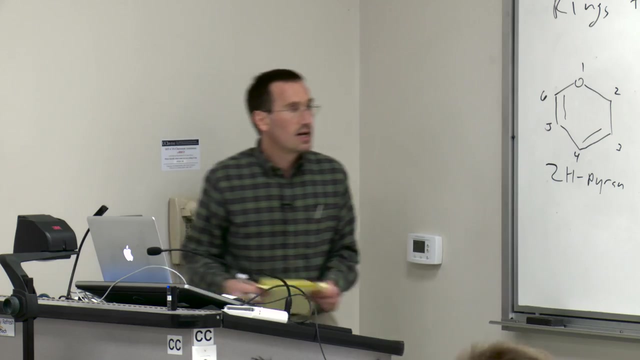 two, three, four, five, six. So if I make a substituted variant of it, this would be 6-methyl-2H pyrran. By the way, if you print on your computer, you would print it with the H in italics and just. 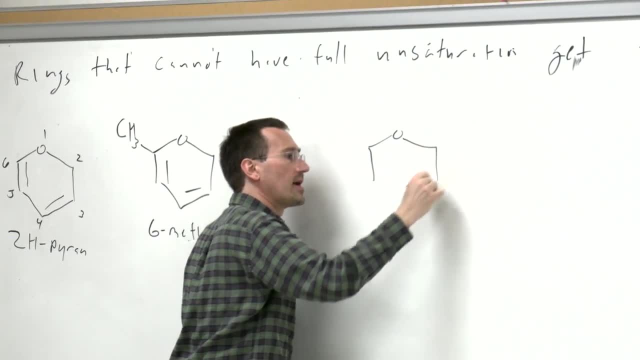 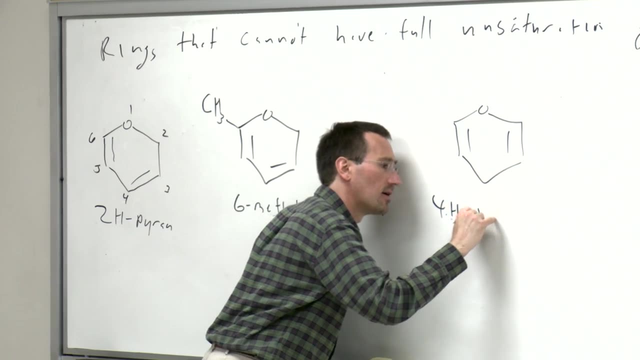 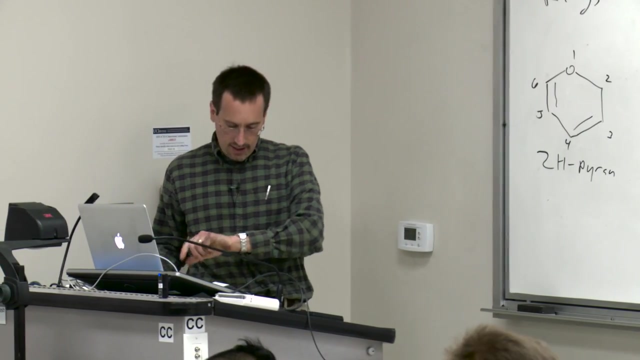 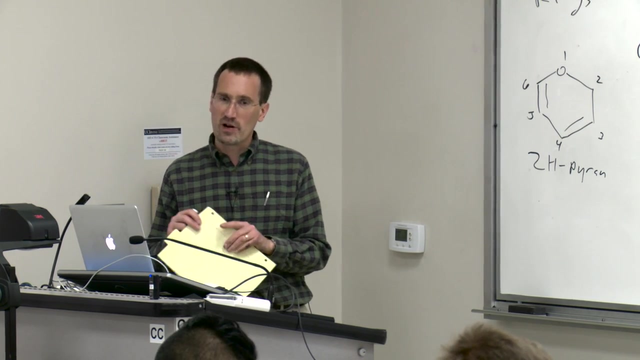 to juxtapose this, I'll show you one isomer of pyrran, of 2H pyrran. this molecule is 4H pyrran. All right, with this brief discussion and the textbook, you have a learner's permit to play with the problems. 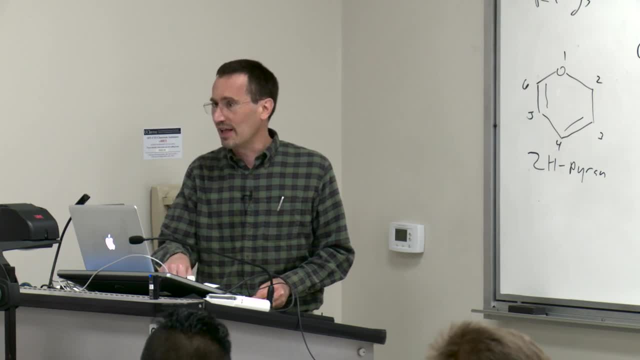 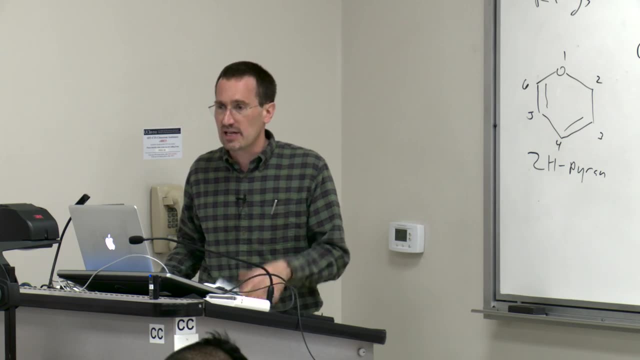 And once you play with the problems, you'll have a solution. You'll have as much of a license as you should have. Read it carefully, play with the problems and internalize some of this stuff And we will pick up talking about the literature.